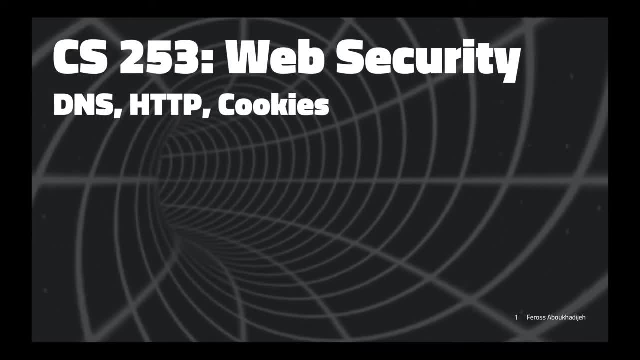 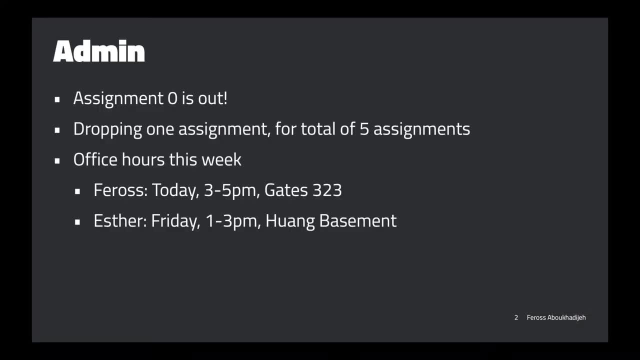 Welcome to CS253, Web Security, Lecture 2.. Today we're going to talk about DNS, HTTP and cookies. So first some quick admin stuff. So Assignment 0 is out. You can go ahead and access that on the website. 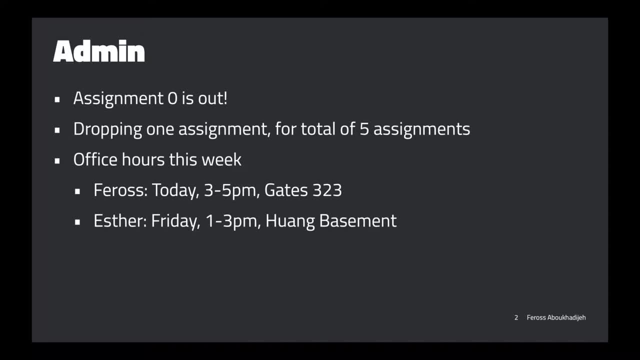 And I decided to drop one of the assignments in the class, so we're going to have a total of five assignments. That includes Assignment 0. So after you finish Assignment 0, there's four other assignments, And office hours this week are going to be for me today at 3 to 5 in Gates, 3 to 23,, and Esther's having her office hours on Friday from 1 to 3 in Wong Basement. 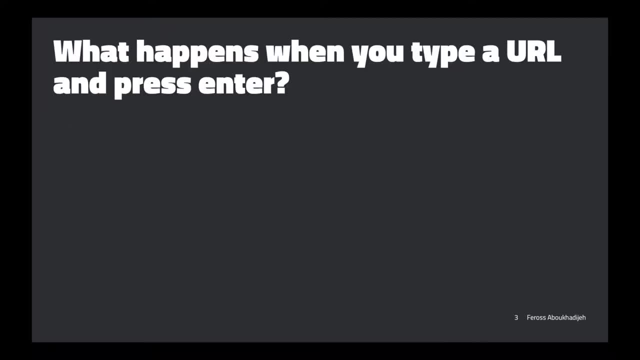 So let's start with considering what happens when you type a URL into your browser and press Enter. So this is actually a really common interview question that is often asked at internships in Silicon Valley, But it's also a good way for us to start to think about you know. 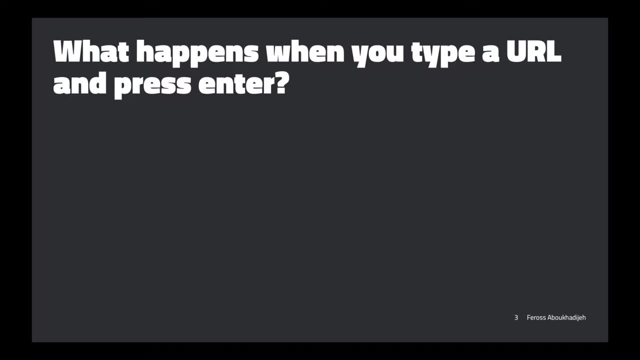 what actually happens when you type a URL into your browser and press Enter, What actually goes on in the browser and what you know. this will set us up nicely for thinking of attacks on this process in the future. So when you type a URL in and press Enter, this can happen. 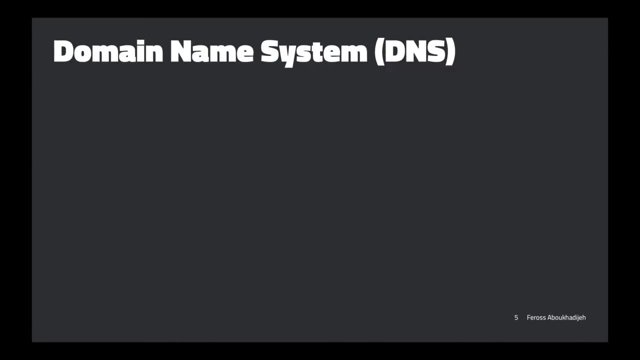 But really what actually happens is, the first step is a DNS query, So the DNS system is a system that translates user-friendly domain names. So IP addresses are the way we address all nodes that are connected on the Internet, And a domain is a friendly, human-readable string that we like to type into our browsers. 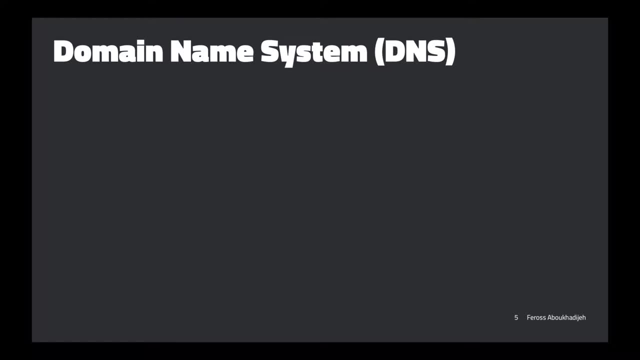 And so we need to do this translation step as the very first step, because the browser doesn't know which server to contact until it does this translation. So we'll go ahead and walk through that process so we understand what exactly goes on. So, at a very high level, your browser makes a request to some server, which we call the IP address. 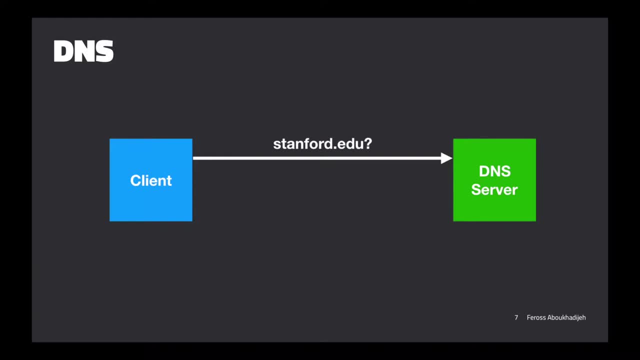 And the DNS server gets this message from the client and it's in the form of a query. So the client is asking a question And the question is: what is the IP address for a particular domain, in this case stanfordedu? 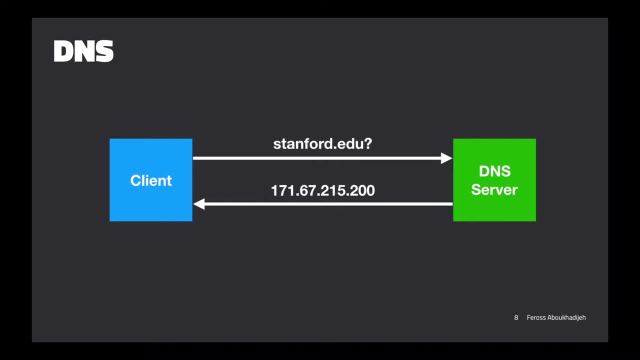 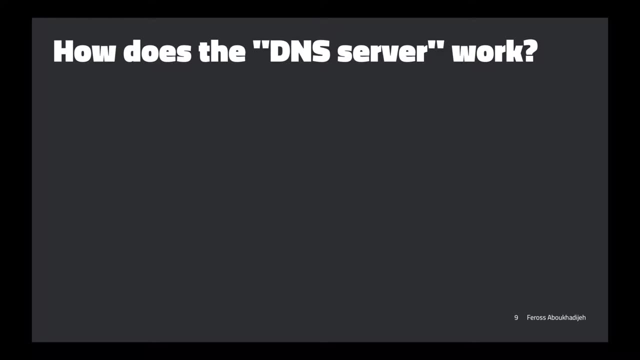 And the server is going to respond with the IP address for that domain. So that's the high level. But what do we actually? what is that DNS server actually doing? So this is a more detailed view of that, of the process. So the client is going to. you know, we start off by sending that same query for stanfordedu to the DNS server. 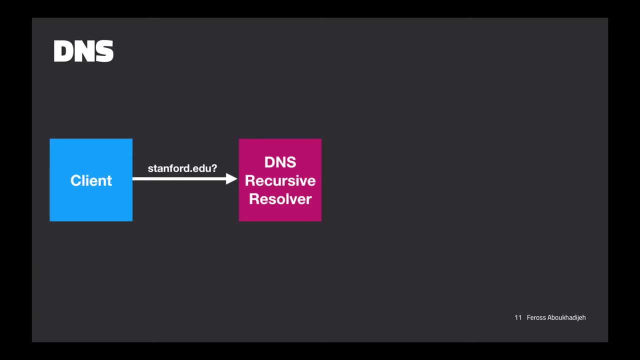 But we're labeling this DNS recursive resolver now, because what the DNS server does is it actually does a bunch of work on the behalf of the client when it receives this query And we're going to take a look at you know what it's actually doing. 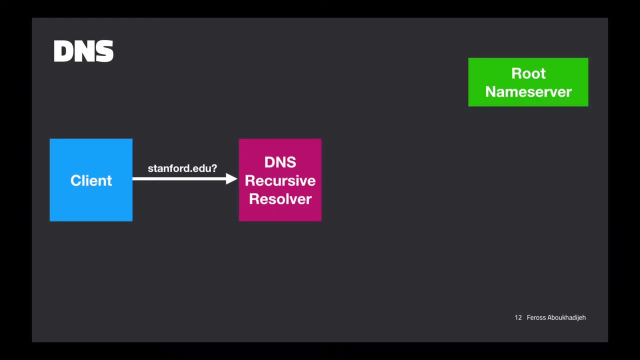 So the recursive resolver is going to take on the responsibility of looking up the IP address. So the client is going to take a look at the IP address for stanfordedu and doing whatever work is necessary to do that, And then it's going to get the answer and send it back to the client. 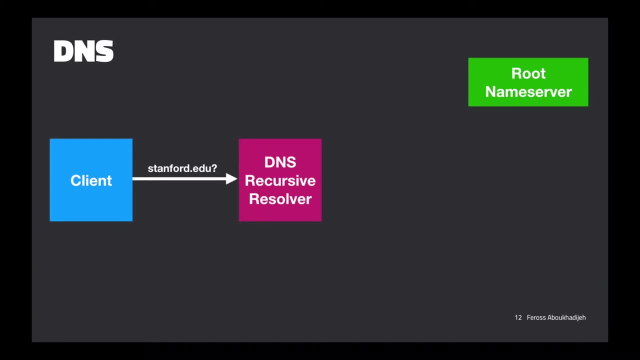 And this process might take multiple steps And that's why we call it a recursive resolver. So this server is going to actually continually make queries to various other servers until it gets the final answer that it's going to give to the client Right. 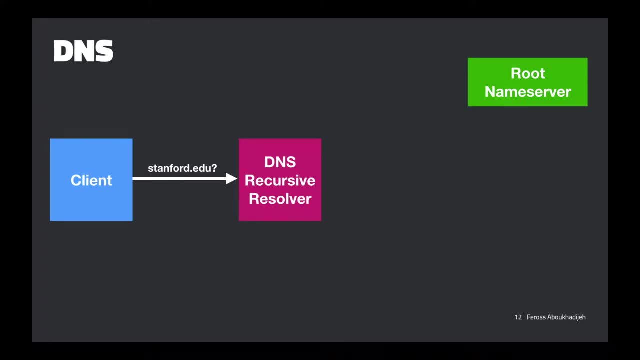 So anyway, there's these root name servers And these are hard-coded into every DNS resolver And they're They're run by different organizations, And so our recursive resolver is going to go and ask that root name server for stanfordedu. 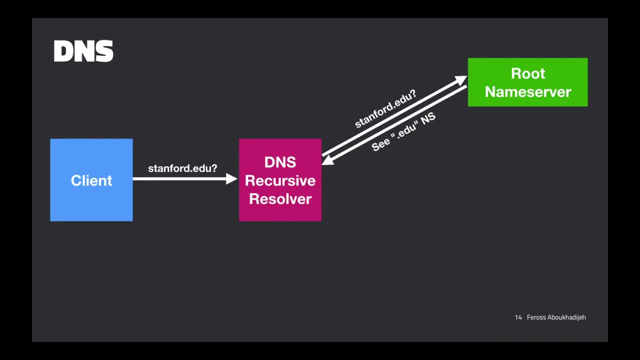 It doesn't know the answer, because again, like this is a problem. There's just a problem with scale here, Like a single server can't keep the records for every single possible domain in the world, But what it does is it delegates authority to another name server that's responsible for just a sort of subset of other names. 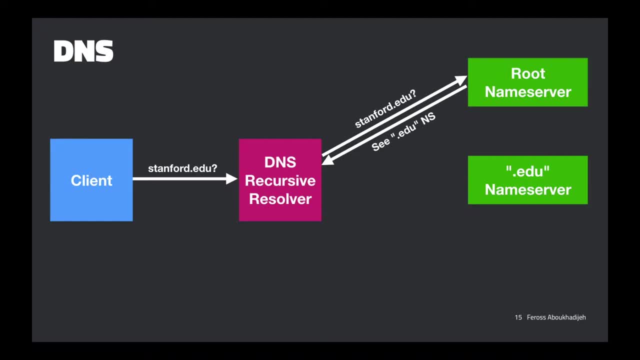 In this case, the EDUs are all managed by a different name server. Now the recursive resolver is going to just go and ask the same question to the EDU name server And again, the EDU name server is also not able to handle a listing of all this stuff. 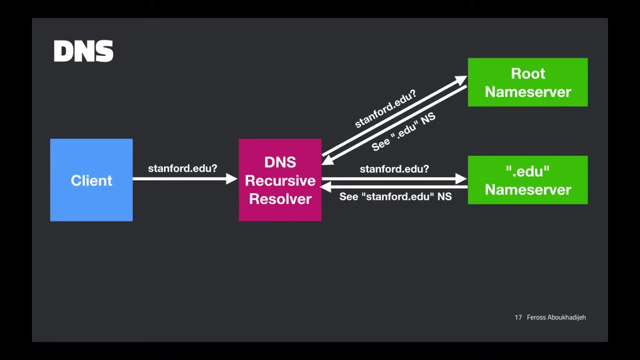 And so it's going to respond with. well, go and ask the stanfordedu name server And we go one level again, And this name server, fortunately, can actually respond, And so this is what's called the authoritative name server. 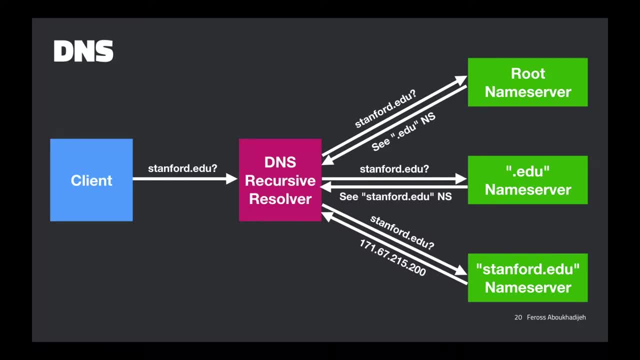 It actually knows the answer to our question And it will respond with stanfordedu address. Cool, Pretty straightforward, Um. What's worth noting here? This is sometimes called the TLD name server, because it's responsible for the whole top-level domain of EDU. 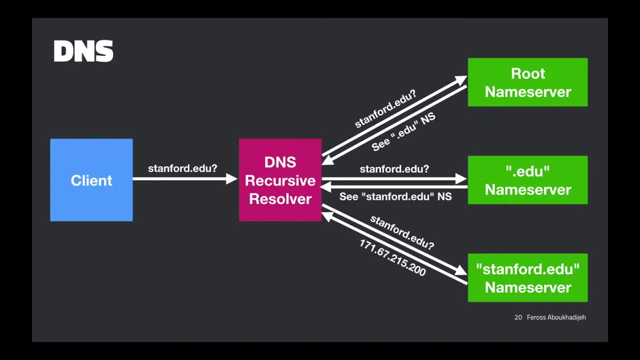 And Let's see Anything else I want to mention about this. Um, I think that's it. Any questions? How many people have seen this before, Maybe, Okay, Yeah, Cool, So So now we have. We have at least a partial initial answer to the question: what happens when you type a URL in? 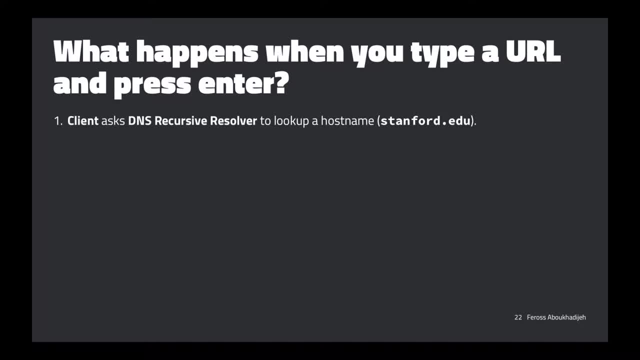 So we do, you know this. we talk to this recursive DNS resolver. It's going to go and talk to the root name server. Root name server responds. Then we follow up. the recursive resolver follows up with the TLD name server, which responds. 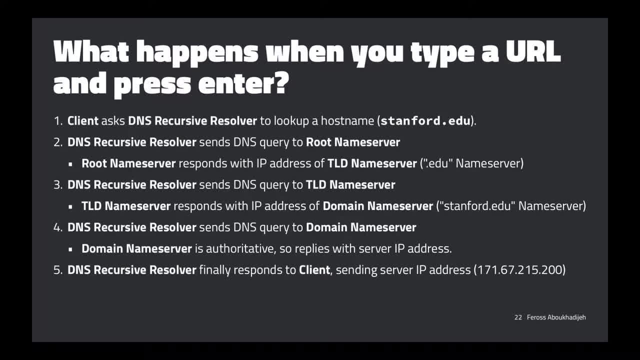 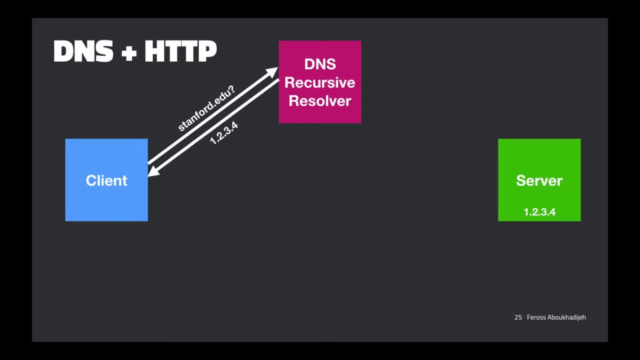 And then, you know, we go again until we hit the Stanford server, which finally can respond with the IP address. Cool, So now let's throw an HTTP into the picture. So this is what it's going to look like. So 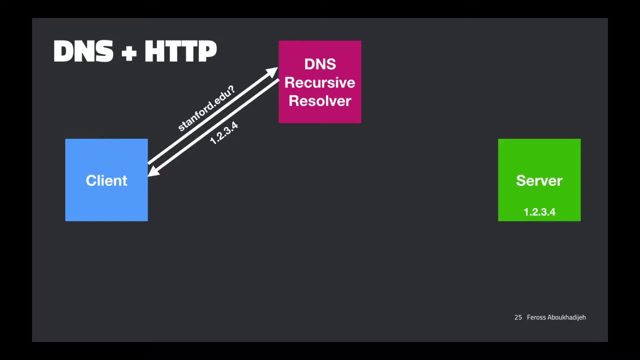 You know we're not done when we get the IP address of the server. Now we actually have to connect to it. So now, when we get the IP, we now know: ah, this is the server we need to talk to, And I guess I changed the IP address here. 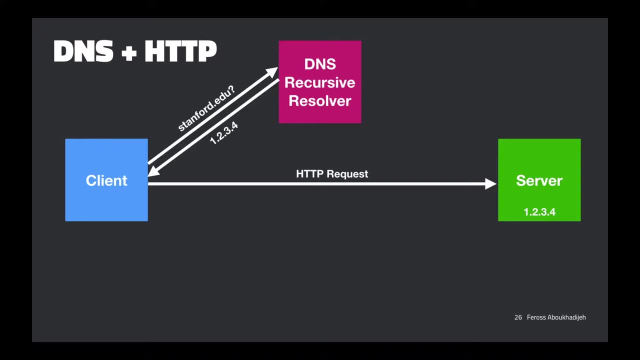 But this is the Stanford IP address And once we, once we know it, we're going to make an HTTP request to it and get back a response. Cool, So now, given this picture, can anybody tell me, do you, can you think of any kind of an attack, maybe on this, this architecture? 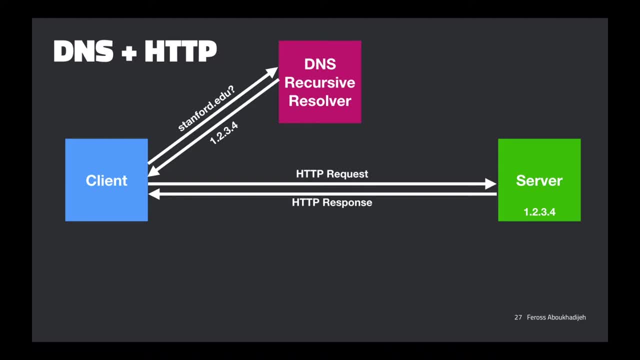 If you were trying to attack, Like a visitor who's visiting stanfordedu, what, what's something you might do? It could be anything, Mm-hmm. Um, if we can somehow, uh, change that number that's being returned from you know the first resolver. 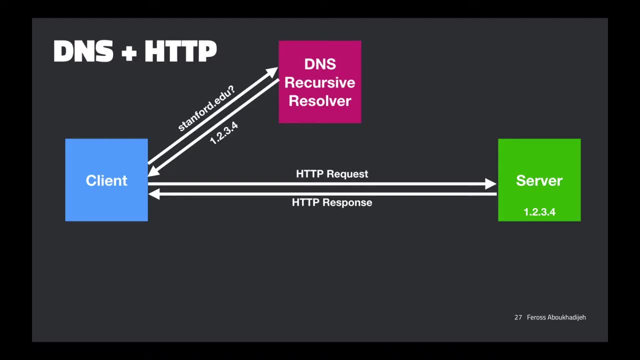 So that the computer would think that this other IP address would belong to Stanford's IP address. Yep, totally, When you type Stanford, the ID would go to that other address. Yep, that's right. Yeah, and you? so you'd be connecting to the wrong server in that situation. 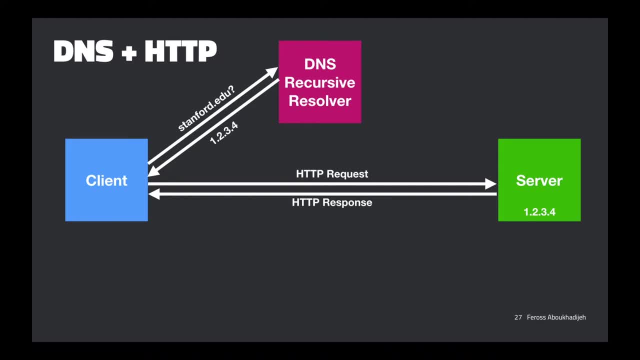 Um, the, the, that particular attack is actually, uh, quite easy to do because, um, these queries are in plain text. So, um, anybody who's uh any, any sort of device on the internet between you and that recursive resolver can insert itself in there. 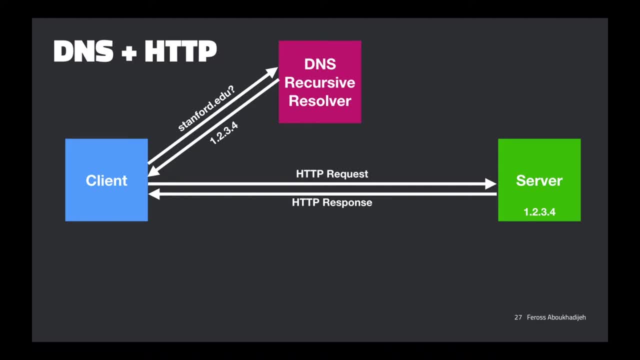 And when it sees that you're making this query, it can just decide to not pass that query onward to the next, like node in the network, And it could just itself respond to you, And then you'll go ahead and connect to the wrong server. 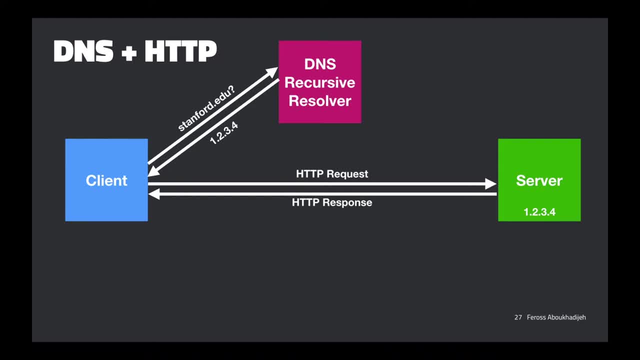 Um, that's, that's, that's totally right. Um, but um, oh, you, you had another idea. No, I was thinking you can attack the response of the server as well. This, The HTTP response. Yeah, that's possible. 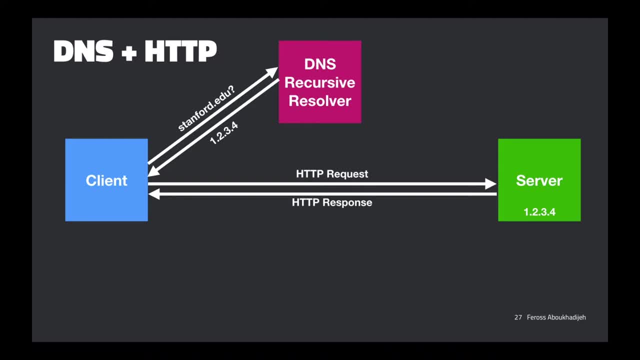 Like modify it and insert it. Yeah, that's, that's totally possible. Yeah, so that's um. do you know the defense against that? No, Okay, Uh, anyone else want to volunteer that? Yeah, TLS. 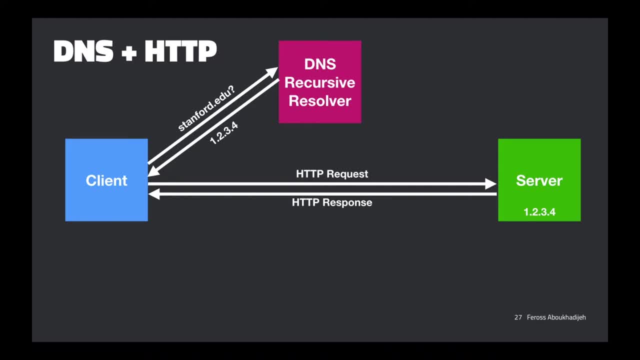 TLS. yeah, So we're going to have a lecture on TLS, But, um, basically, TLS is, is, is, encryption, It's what you, when you see HTTPS in your browser, Um, and what that gives us is, um, a couple properties that are really important. 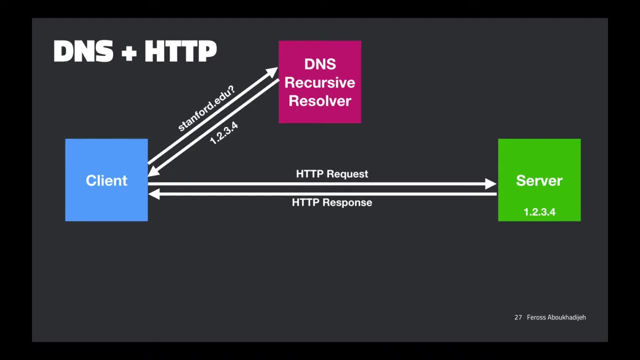 One is um integrity, which means that the response can't be modified. If it's modified, then the client will be able to to tell Um and um. the other one is um authenticity, which ensures that we're talking to the 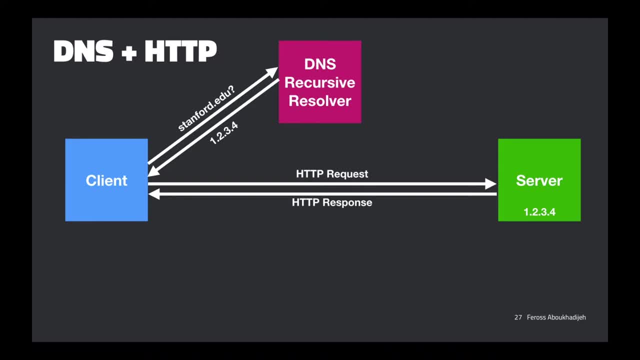 the server that we think we're talking to. So if anybody were to try to insert themselves in there like you suggested and send back a different response, we wouldn't trust it. Um, so that uses um like signatures. 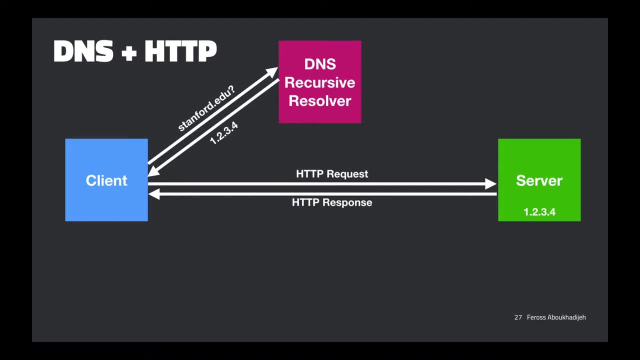 which, if you want to learn more about it, you should take uh 255, which is an amazing class. Um, but yeah, so, um, so yeah, we can interfere in the, you know, in the in the HTTP process. 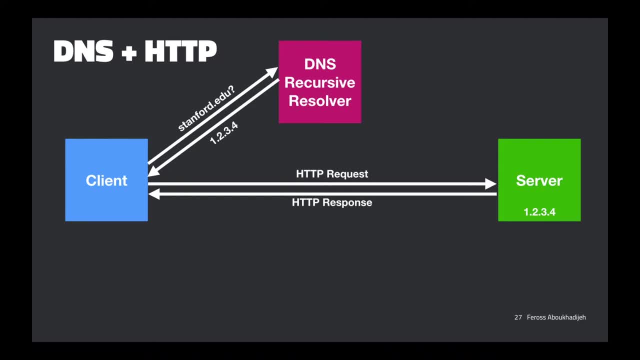 or in the DNS process. Totally, Those are both both valid things. Um, with HTTPS. um, of course, like I said, we'll be able to detect that somebody has has sent us to the wrong server, Um, but one thing that's interesting is um. 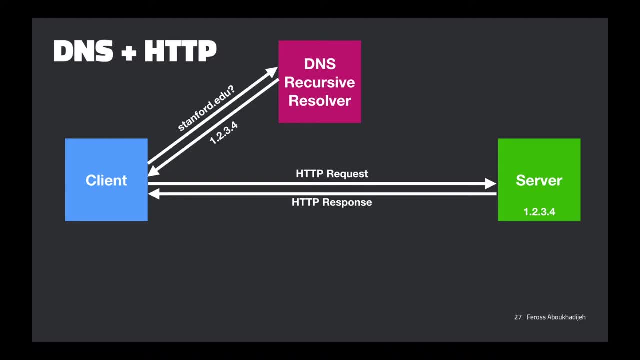 uh, let's see here. So, so yeah, if, if you're, if you've inserted yourself in here and you're here, actually I have a picture of it. Um, oh, no, it's, it's later. 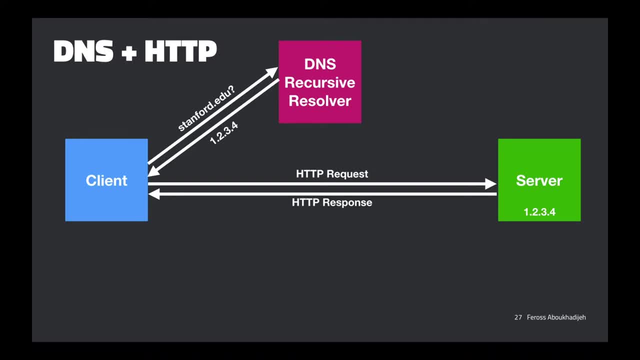 Um, yeah, we'll, we'll just get to, we'll get that, get to that in a sec. So, just uh, just to um review some of the the stuff we talked about. So, um, right, so you can change the DNS records. 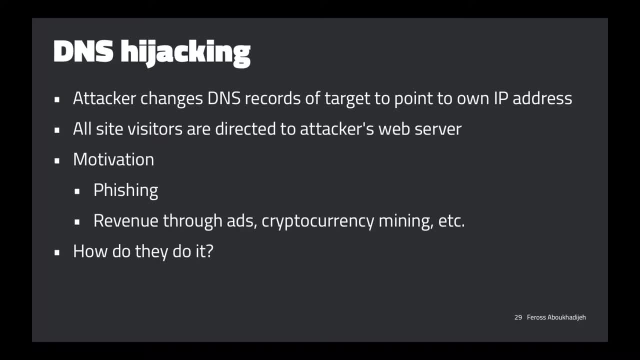 of the target domain and point it to your own IP address. And now, when visitors uh go to the site, they're going to be directed to the attacker's web server. Um, and the motivations for this are like: now you know you can basically load anything you want. 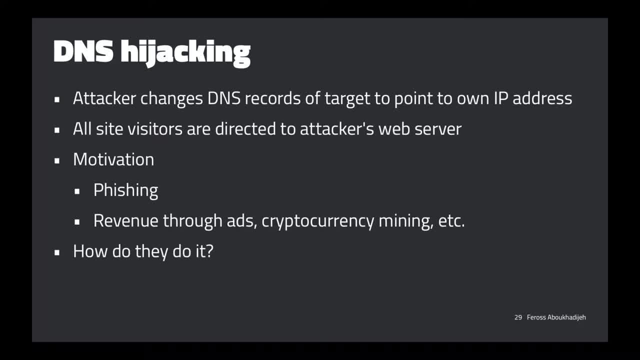 Um, and the user's going to potentially think that that's the original site. So you know that's called phishing, Um, and you can collect the user's passwords or whatever you want to do. Um, there's also, um, you know, money-making things. 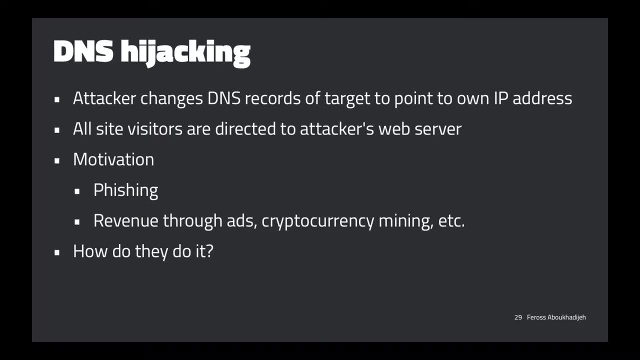 Like there's these JavaScript crypto miners, which are pretty hilarious Basically, um, it's a bit of JavaScript code you can put in someone's you know, put into a web page, And that's going to actually try and mine like: 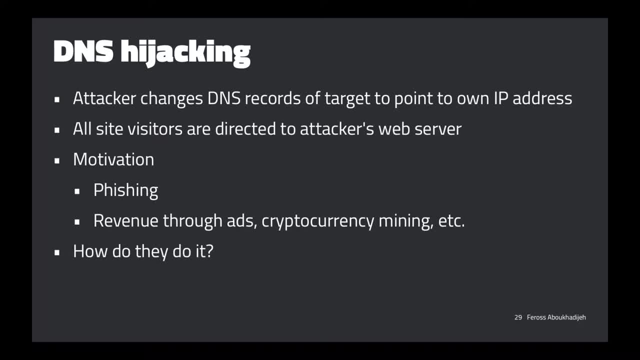 typically- I've seen it- they mine Monero for whatever reason. Um, I think because it's easier to mine that on CPUs. I think that's the reason. But anyway, it's pretty hilarious because you might be on a laptop. 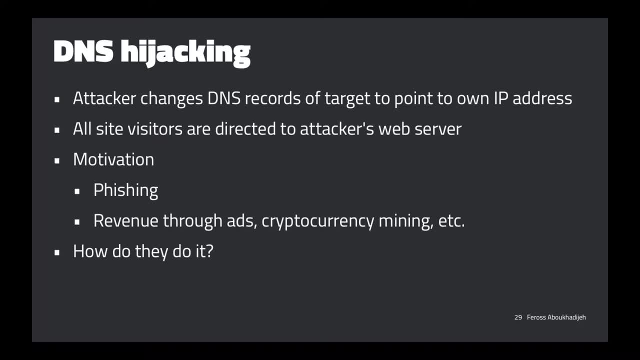 which is not very suited for mining cryptocurrency. But the attacker doesn't care because, um, you know, even if they can make like five cents, um and burn $3 of your electricity in order to do so, that's still five cents of profit for them. 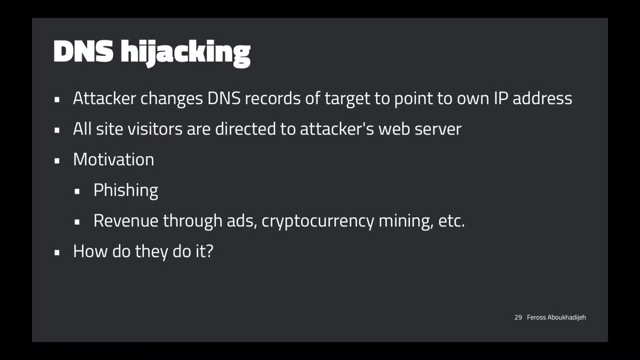 So that's kind of a pretty hilarious attack vector, um, or attack that we see in the wild, Um. and then, of course, you can just like change the site Subtly, including including ads in the page. 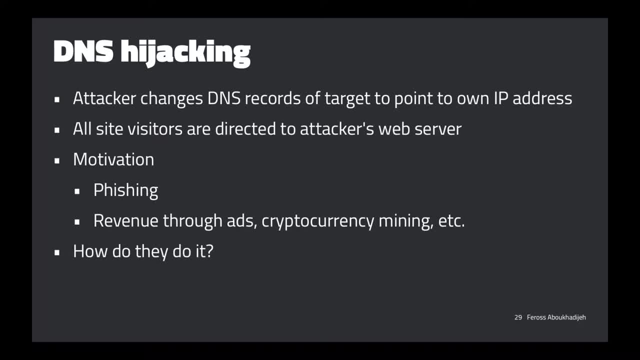 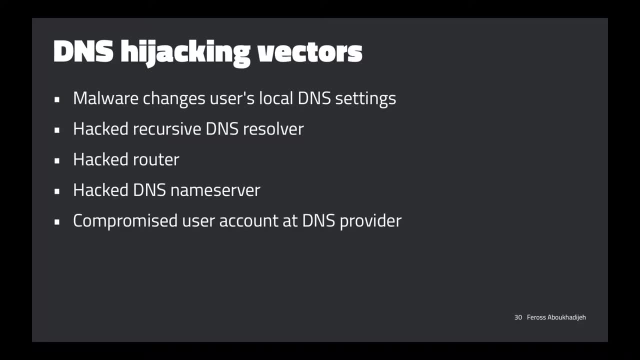 or something like that, and it's another revenue source. Uh yeah, so so, um, how do you actually go about doing this? Um, there's a couple of of of of different places you can. you can, uh, affect DNS. 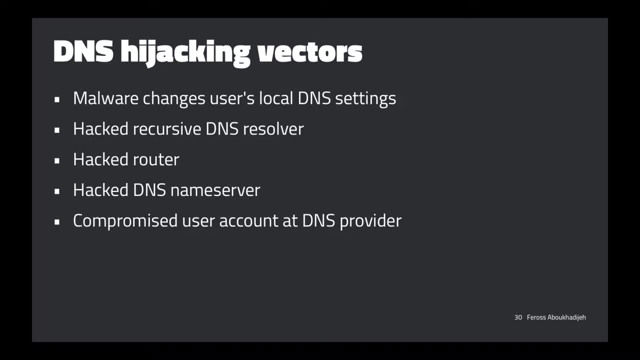 So one is directly on the on the user system. So if you have malware on your machine, um, the malware can go in and just change your local DNS settings so that it's going to basically route a domain to a different destination than it should. 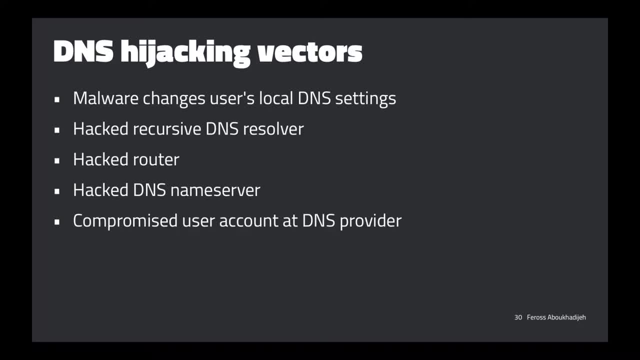 Um, you can, uh, you can actually just do this yourself on your own computer. if any of you have ever um, uh, modified the Etsy hosts file before, Um, that's, that's a way to basically say: you know, whenever I do a a DNS lookup on my computer, 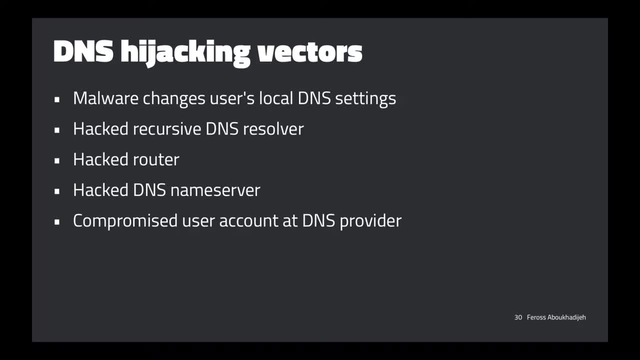 I don't care what the true answer is. I want to hard code in this IP address as the answer, which can sometimes be really useful if you're testing, Um like, you're trying to test your website and you want to just say like: 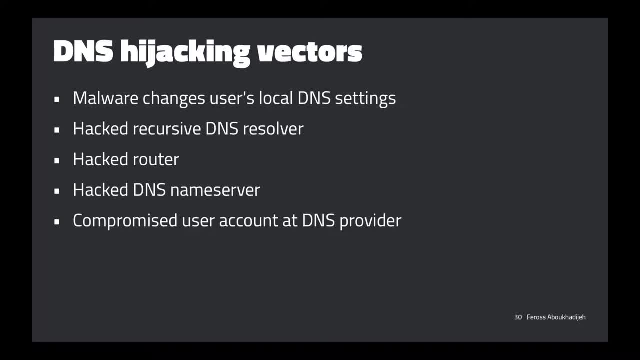 okay, always point it to my own computer when I, when I type in my domain name or something like that. Um, but malware can go ahead and change that and that's that's really not good. Um, you can have the DNS resolver itself get hacked. 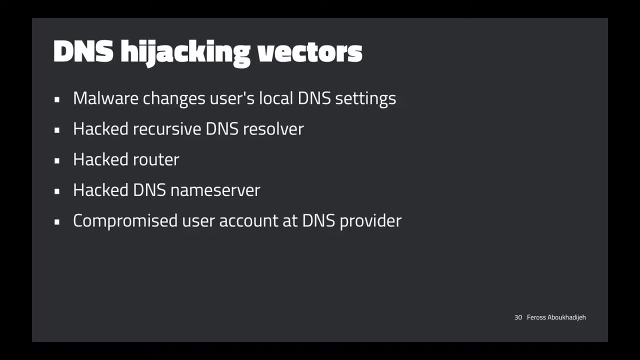 um and um. typically, you're using the DNS resolver that comes from your internet service provider, Um, so in the, in the case here at Stanford, it's just Stanford has like an IT team that provides this for us. 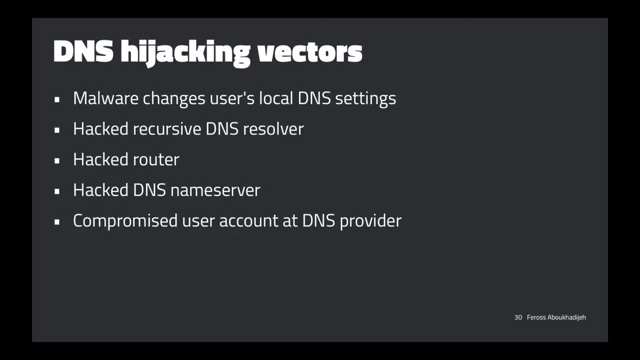 Um, if that server were to get hacked, it could just start giving out wrong answers to everybody and our browser's going to go to that. you know that wrong IP address. You can also have hacked routers and um, and then the DNS name server itself. 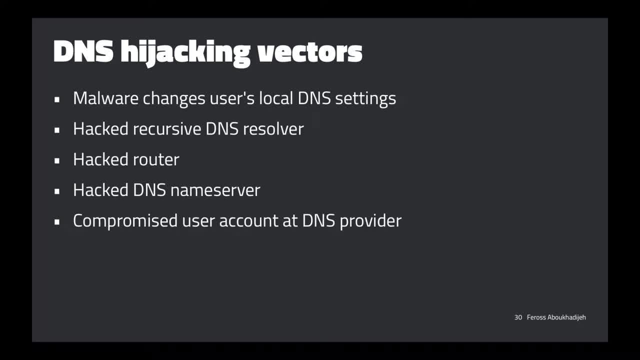 So that's the actual um, the thing that's responsible for, let's say, Stanfordedu. If that thing is hacked and it's just going to give out the wrong IP address, that's another, another issue. And then, lastly, like you, you might have um. 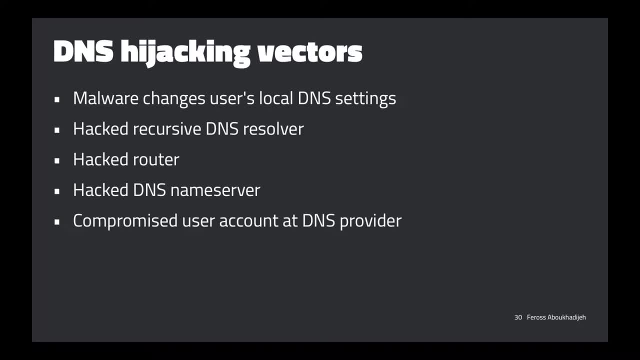 a company that you're, that you're paying to provide this DNS name service for you, and if you, your account there gets hacked, then we can go in and, of course, change, change stuff. Um, so this is the the flow in that situation. 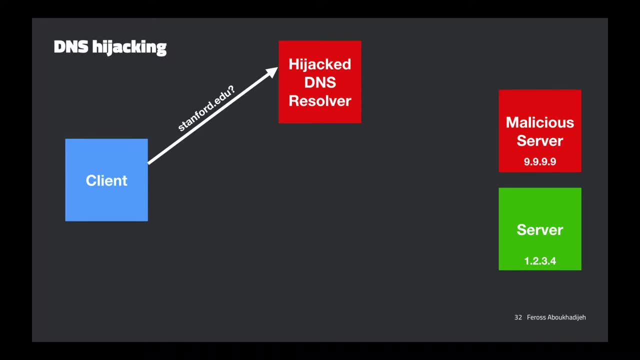 So you have a hacked DNS resolver. You have, um, uh, the request goes to it, It responds with the incorrect IP address, and then your browser just connects to the malicious server. Um, and there you go. Um, so, so, so. 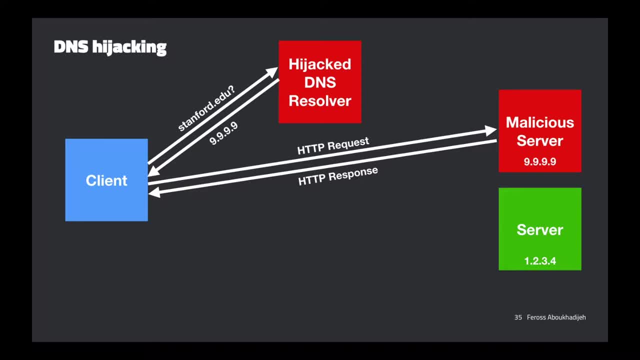 so we mentioned HTTPS might help us here. Um, so how, how, how? how might HTTPS help us here? Anyone have ideas? Yeah, Uh, since HTTPS provides, um, you would know that the malicious server is not the real server. 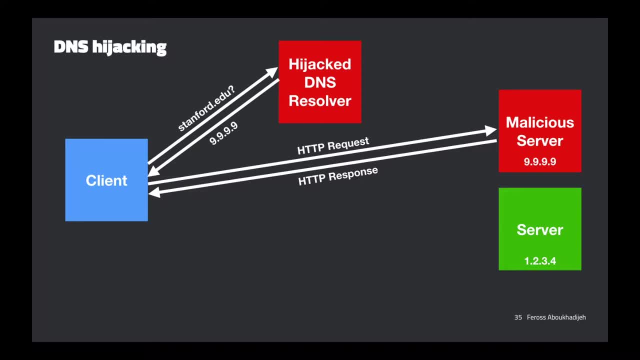 Mm-hmm, That's correct. Yeah, That's so. so to repeat: um, I mean if, if your browser's expecting to get back a certificate that says, oh, we'll talk about this stuff later, We're getting a little ahead of ourselves here. 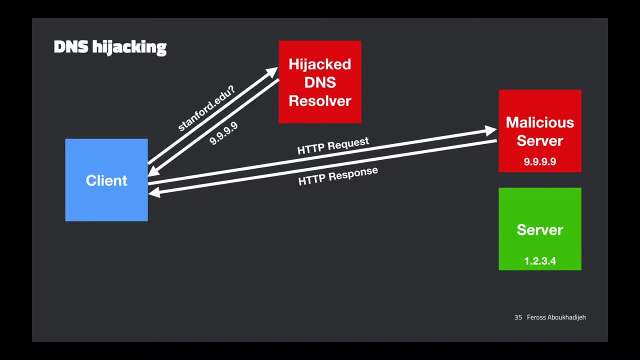 by getting into the details of of HTTPS, but um, uh, but I think that's okay. Um so, so if there's a way that this server could, where the browser expects the server to prove itself to the client before it trusts it and before it sort of um. 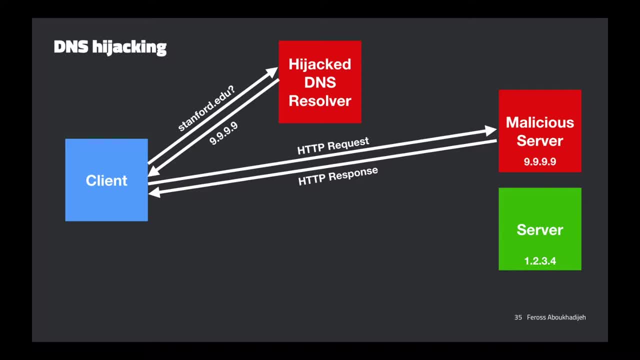 gives you the lock in your browser. basically, then, we would be able to know this happened, Um, the the interesting uh, like kind of uh wrench that uh gets thrown in here- is that, um, there are uh services. 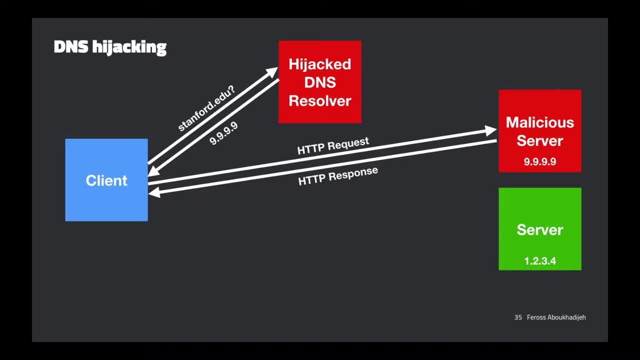 like Let's Encrypt, which um provide free certificates to anyone who can prove that they are in control of a domain right. If the attacker is able to make it so that when Let's Encrypt or any provider, who's gonna issue these certificates? 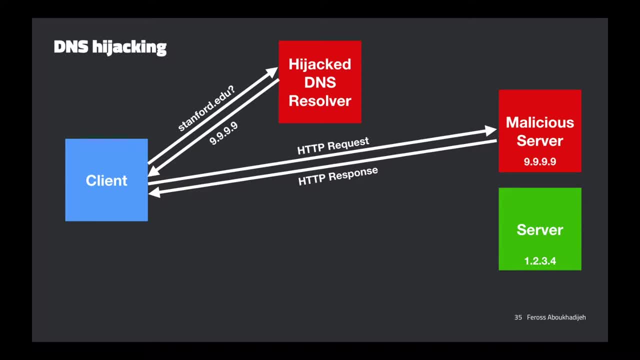 if they can make it so that when they go and check, like what is the server that Stanfordedu is pointing to, and they get back this wrong answer, um, then the that that provider is going to now connect to the wrong server. 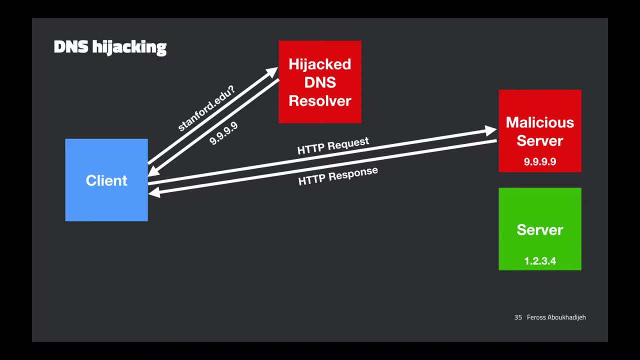 and it's gonna issue this challenge to the server that says: prove that you want me to actually issue a certificate right now. and the attacker will say: yeah, of course, issue the certificate. give me that, please. And now they have a certificate that they can provide. 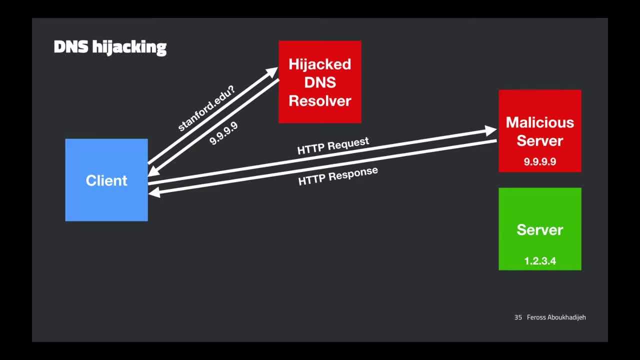 in this response. that will make your browser trust it. So this is actually really bad. Um, even HTTPS- uh, you know, in the way it's normally used, can't help you at all here. Um, it's really bad. Um, yeah, so, 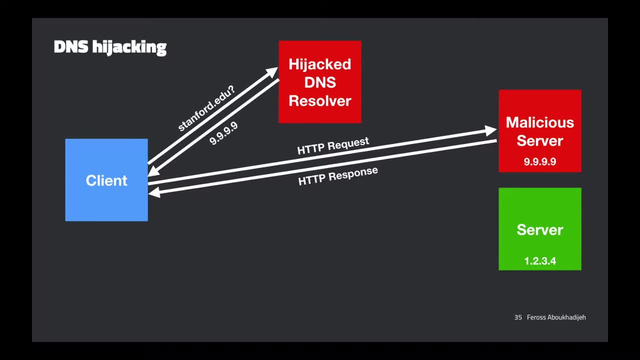 does that make sense to everybody? Any questions? Yeah, Yeah, so, um, we'll have a whole lecture on this, so I apologize for getting a little ahead of myself here at this, but, um, but basically the way to think about it is: um, there's, there's. 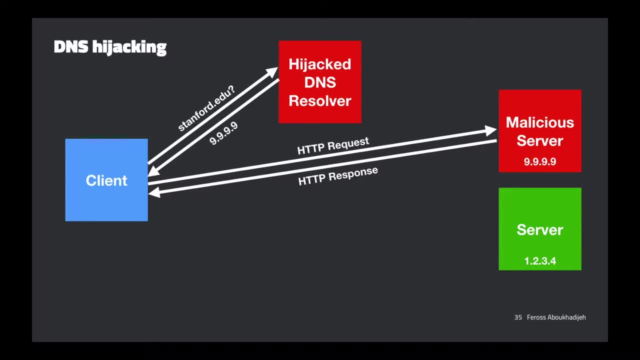 a company which, if it can prove- um, if you can prove to to the company that you're in control of a domain name, right then they're willing to say: okay, we proved, like we, we're convinced that you own. 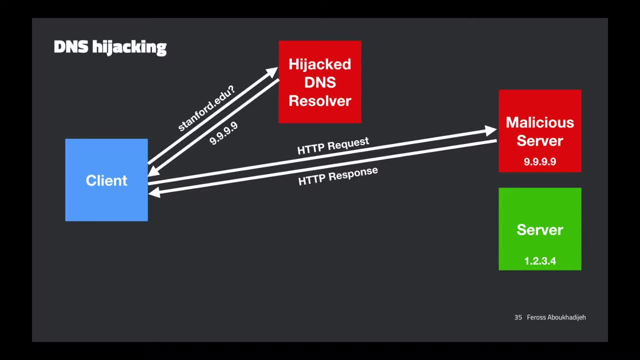 this domain. so what we're gonna give you is a um, basically a file. it's just a text file, that's a certificate, that um you can now that that person who owns that domain can now attach to all the um. 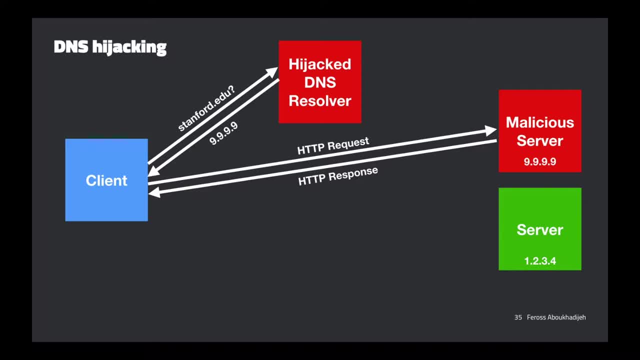 basically attach something to the, to the response that they give to everybody, and now the, now, the uh, the client can know for sure that the person who sent this response is in control of this um, of the private key that goes with that. 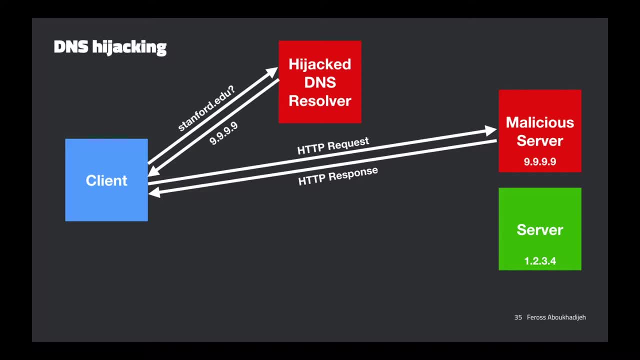 certificate, And so, basically, they're the person who's actually running this, the server in question. Um, oops, um, so, uh, and so that's important because, um you know, on the internet, like all these, uh, all these, 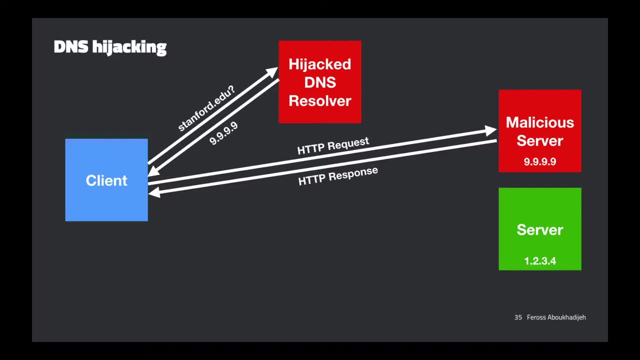 requests and responses are getting jumped around over many nodes, and a lot of these nodes are controlled by completely different entities than the client or the server. They're just random companies, Um, or, you know, government agencies, in some case have uh can affect. 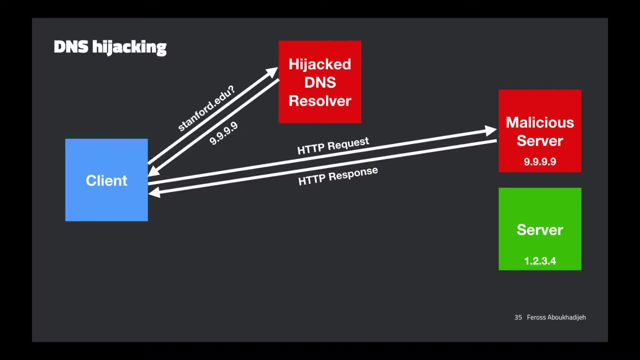 those nodes and they can modify those requests. or, you know, like we were saying before, insert themselves in um and send a different, different response. And so, if they don't know the private key that goes with that certificate, 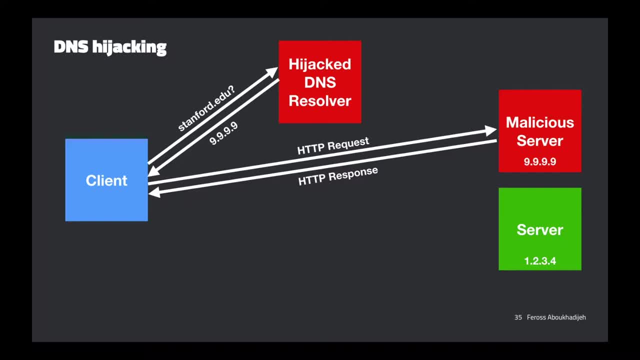 then they won't be able to do that, right? That's kind of the idea. Does that make more sense? Okay, Yeah, we'll have a whole lecture on it. Um, cool, In fact I'm trying to get um, trying to get Dan Bonetti. 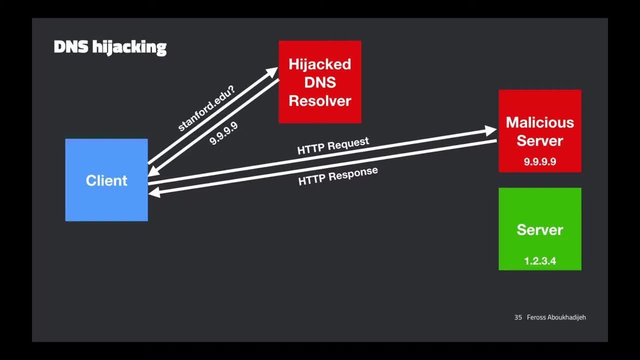 to give that lecture because I think he'll do a really good job at that. Um, but yeah, he might be one of our guest speakers. We'll see He's really busy, Um, but yeah, okay. So so just some some stuff in the news about this. So, 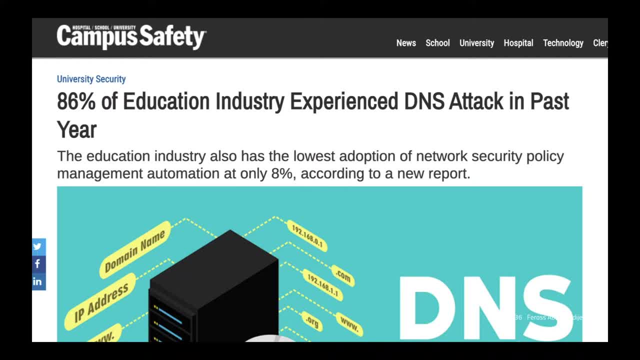 a ton of education, um, like a ton of ton of universities and schools and stuff, are affected by these kinds of attacks, Um, and mainly it's to steal people's personal information. So if you, if you can convince um, if you can trick like an administrator, 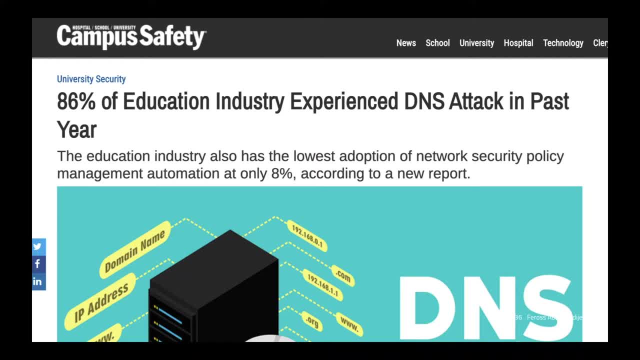 to to go to a different site and log in there and then you can get their credentials and steal everybody's um their everybody's socials and their payment information and stuff like that. Um, a lot of schools don't have, like, don't invest. 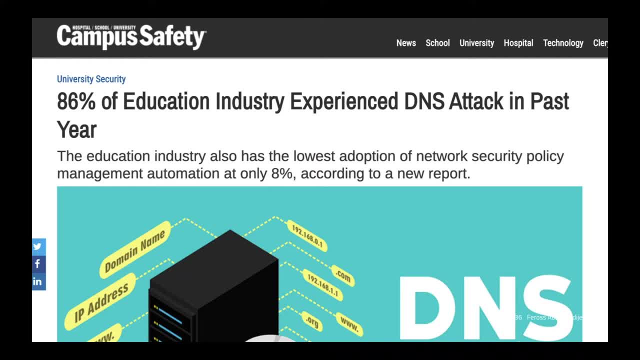 in in their, in their IT infrastructure, because they're not funded very well. In some cases it's like one person who's like responsible for a whole school district or something like that, And so there there's just like lots of um misconfigurations. 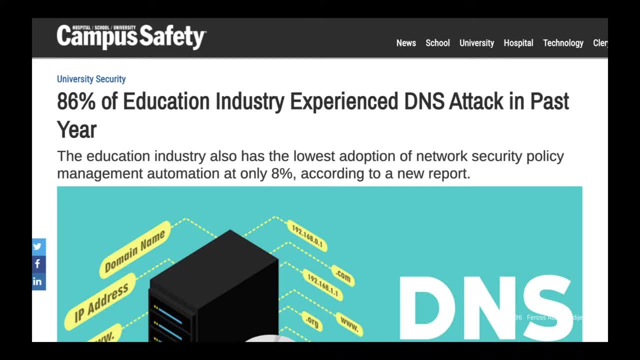 and um weak passwords and people just haven't like tried, tried very hard to to secure this stuff. Um. so, yeah, it's, it's a huge, huge number of attacks. Um. another place where you see this: 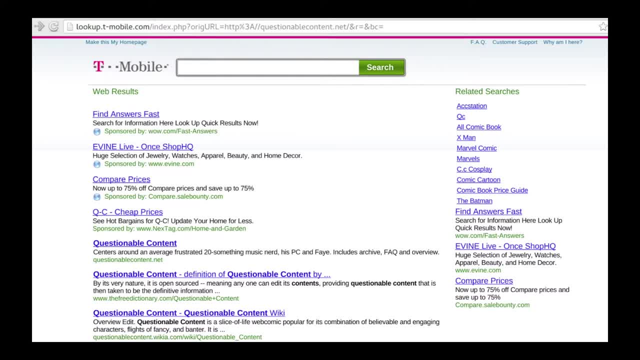 is um. internet service providers will actually do DNS hijacking, Um. so you're not, you're, you're, you're um moving your head up and down. Pierce, Have you seen this before in the wild? Yeah, I've seen it a lot with like back in the day. 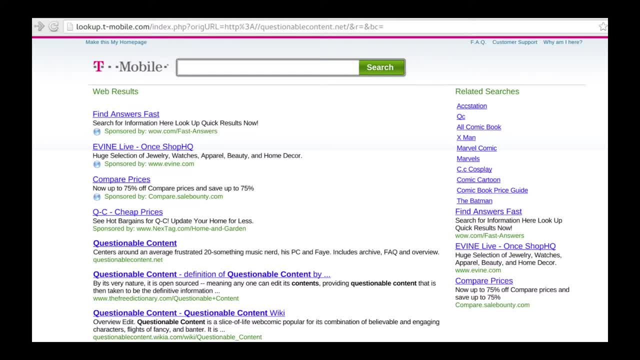 with, like those browser toolbars They would like hijack, like um domains that wouldn't have, I guess- uh, that wouldn't be valid- to point to their own search pages and like sell ads. 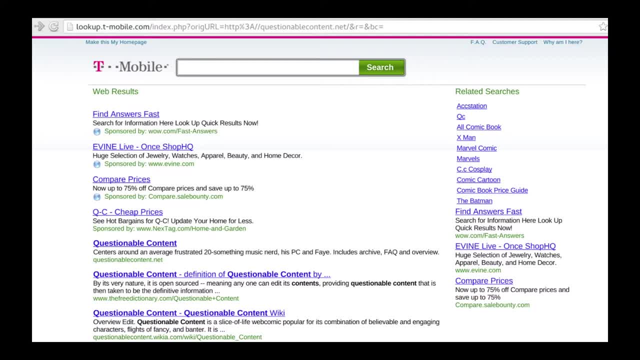 Yeah, that's exactly what this is here. So so to repeat, um, what what's going on here? is that? um, if you type in a domain that isn't valid, so it's like a, it should just return a browser. 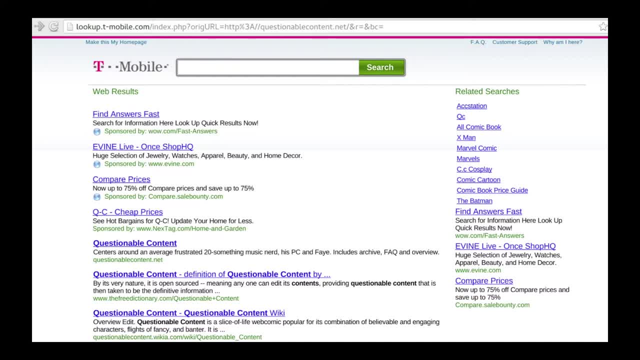 error page to you Like there's no actual server there, There's no record to find. Um, what this? what these companies are doing is they're saying: well, well, why don't we just show you a page that's like more useful than an? 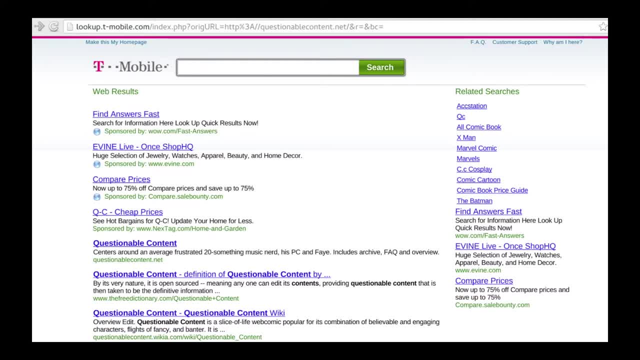 error page. right, An error page is, just like you know, not gonna help you, But we can show you a nice, useful search page with lots of nice- uh, I guess those are, yeah, sponsored by, sponsored by, um so on and so forth. 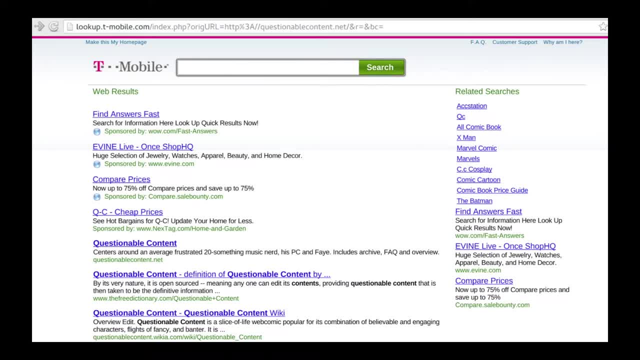 So it's, it's like, yeah, it's gonna make them more money. Um, the the bad, the bad thing with this is that, um, in this case, this is actually for a domain that exists, Which is a webcom called Questionable Content. 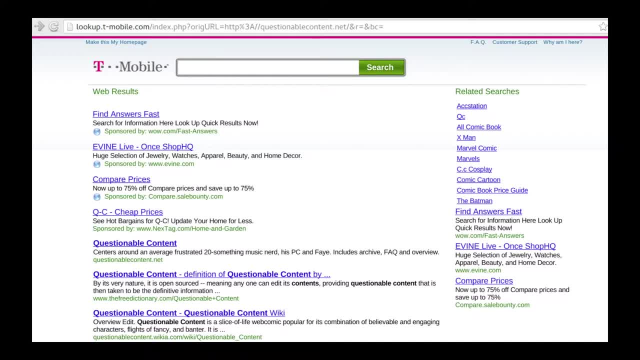 And they're, they injected themselves in there anyway, So their, their implementation is buggy. Um, so it's just a, it's just a bad idea. Like this is like the kind of thing that an attacker is doing. You don't expect, your, your. internet service provider to be doing this to you. Um, but yeah, you can, and actually T-Mobile does do this to you. I have T-Mobile and you can turn this off. Um, if you, if you, I think, if you go to the bottom. 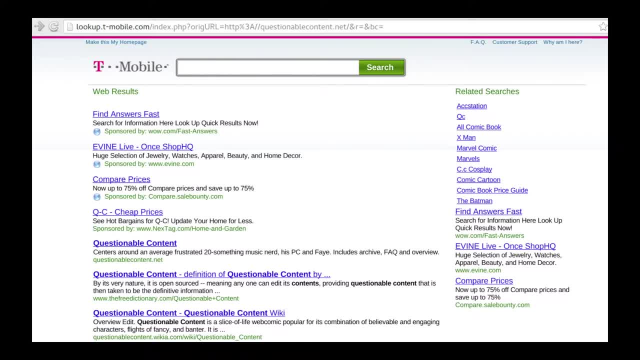 or there it is. Why am I here? You can tell them like: stop this. But anyway, yeah it's, it's really bad. Comcast also does it as well. Um yeah, Cool, So, um, so yeah. 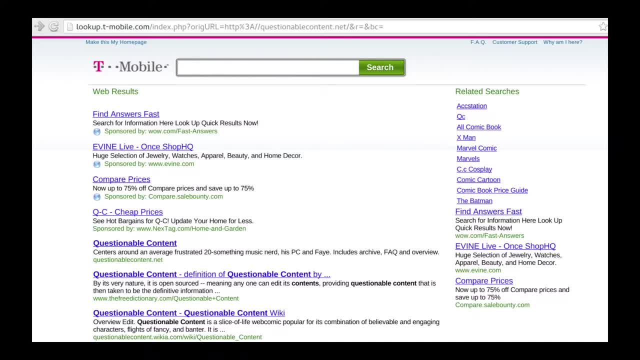 but in the case of, in the case of the ISPs doing it, one thing that's nice is they're not- at least they're not, going and registering certificates for the domains that they're, that they're hijacking They're, they're just um. 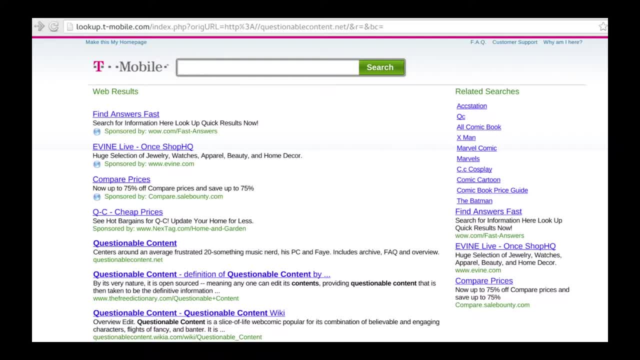 they're sort of they're just responding with these, these error pages. Um, if they were to try to do this to a site that was actually HTTPS right, they wouldn't be able to provide that certificate to prove that they're the true um. 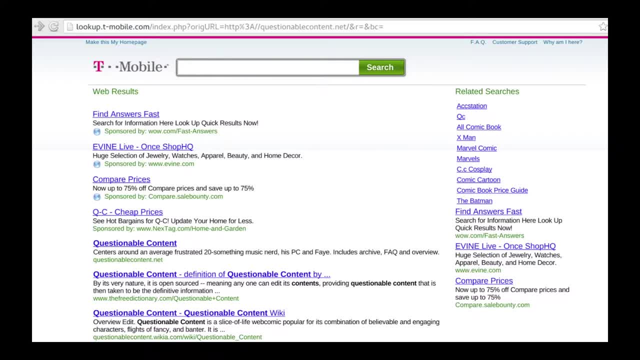 owner of the domain, right? Um, in this case, I think this is HTTP. You can see it there in the URL, So that's why they're able to to return a page and then the browser. the browser trusts that. 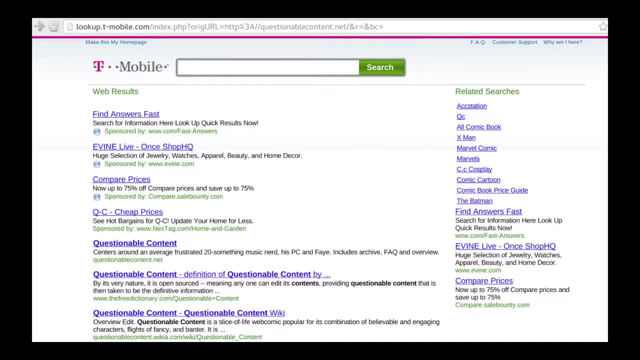 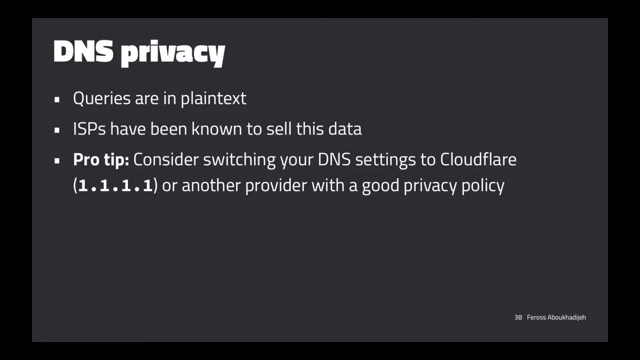 Cool, Any questions about this? Cool, So, okay, so, um, so yeah, let's talk about now about, um, just a few of the privacy things that come up. So we talked about security of DNS, but privacy is. 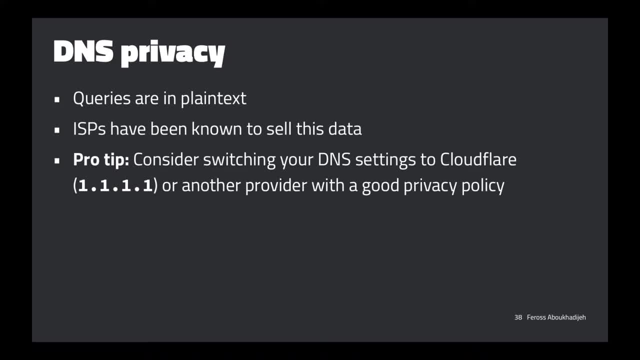 also a big deal. So we talked about how the queries are in plain text: um and if you're. if you're um, if the server that's sitting there, that recursive resolver, just wants to like log every request that you're making to it, they can do that. 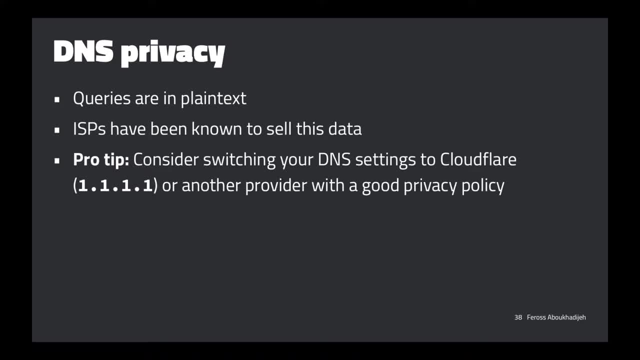 And they can produce these lists of of domains that you've looked up. basically right, And these companies, these internet service providers, have been known to sell these lists. So they'll say, like you know, the this subscriber. 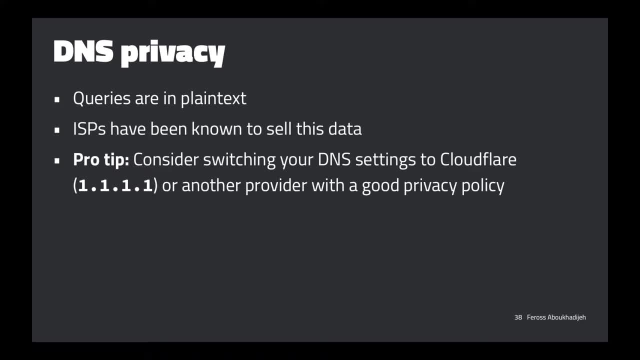 this internet subscriber, like, frequents these domains. Um, and you know that's obviously not something that you probably expect to happen, um, or expect your expect a company that you're paying to be doing, but, but this is possible because 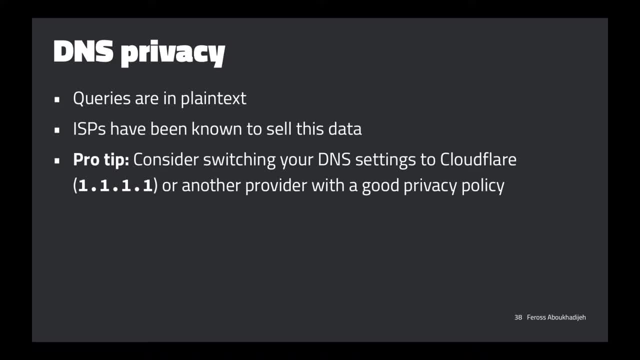 of the way the protocol is designed and the fact that those queries are in plain text. Um, so one one like just personal trick you can do if you don't want this to happen is: um, you can just set your. 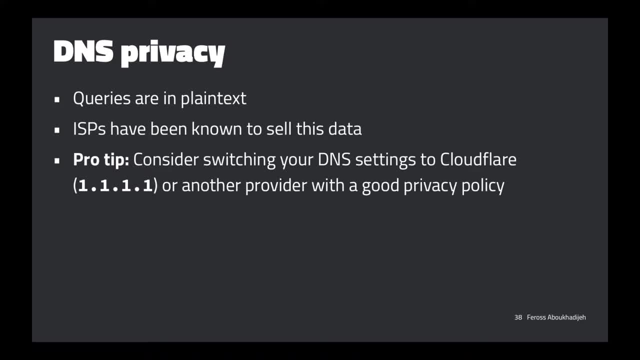 DNS settings on your computer to, um, a different company, uh, that you have to trust again. but, um, at least certain companies have posted privacy policies that say that they that they don't sell your stuff, In particular this uh service right here. it's really easy to remember. 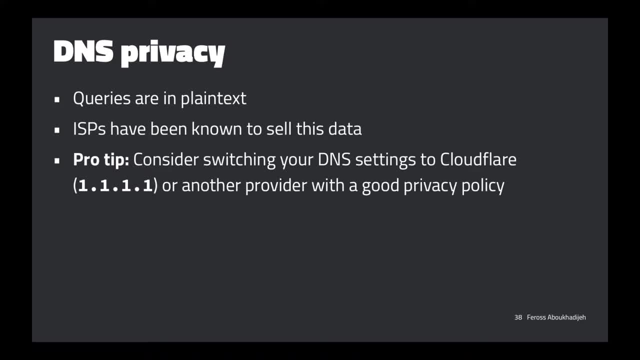 It's 1.1.1.1.. They um got that IP address. uh, that's a CloudFlare service which provides a DNS that doesn't. they say: sell your um DNS queries to companies. Um, I think on Android. 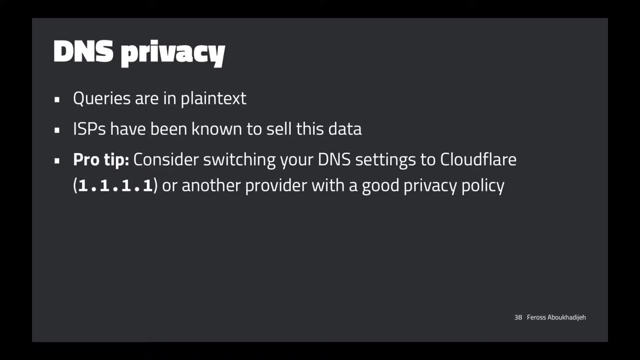 they now can also encrypt your DNS. Oh, is that? uh, So the other people on the network can't see it, even if they aren't your DNS provider, Even if they aren't your DNS provider. Yes, yes, yes. 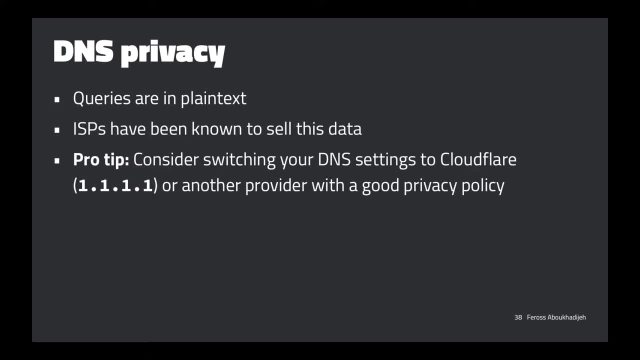 I was about to mention that next. yeah, So what you're referring to is: I think there's this, uh, there's this sort of enhancement to DNS that's brand new. that um is is being developed at the moment. um. 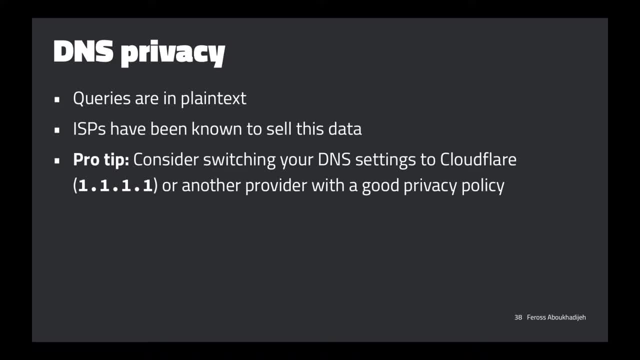 called DNS over HTTPS, And the idea there is: um uh, we want to um uh encrypt our DNS query itself so that people who are, you know, observing that query can't, can't actually see it. So so, in this situation here, like, 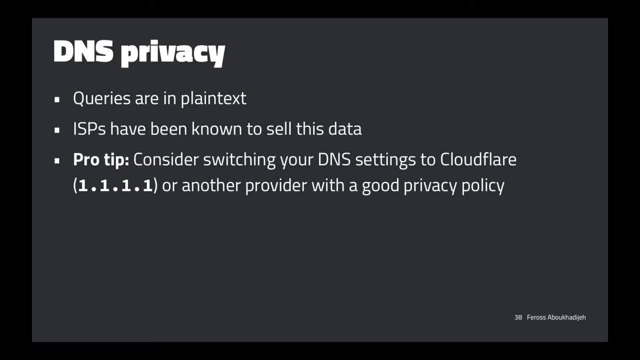 uh, going back a second to the way that. so I was suggesting that we all use CloudFlare as an example as our DNS provider. We're sending these queries. they're still in plain text, right? The? the difference is now. 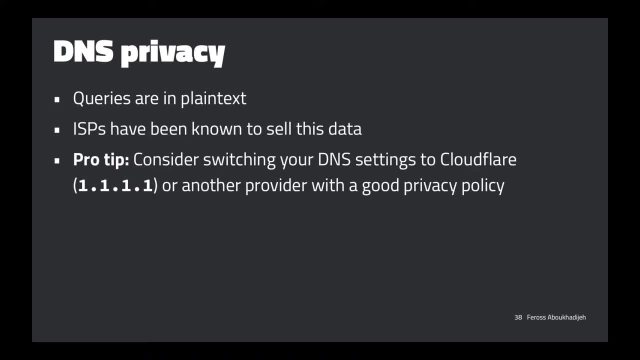 like now, CloudFlare, when it gets this query, it's going to not save a copy of it and sell it to somebody, It's going to send back the answer to us. But but this communication is completely in the clear here. It's plain text, right. 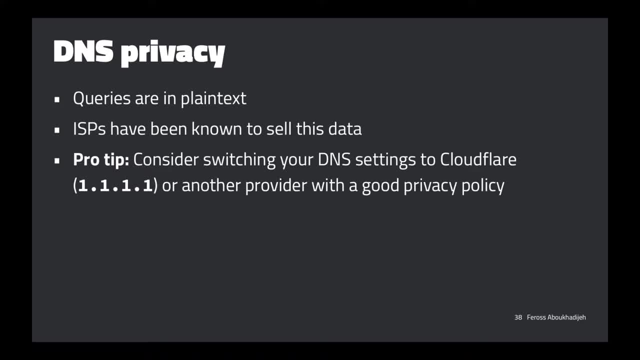 So, uh, again, our ISP, if they wanted to, could say: oh well, you're not sending your DNS queries to us, but what we see? you're sending them to CloudFlare and we can, we can just see the query. So we're going to go ahead and 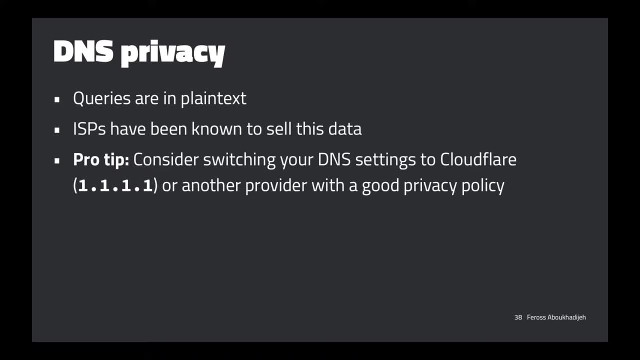 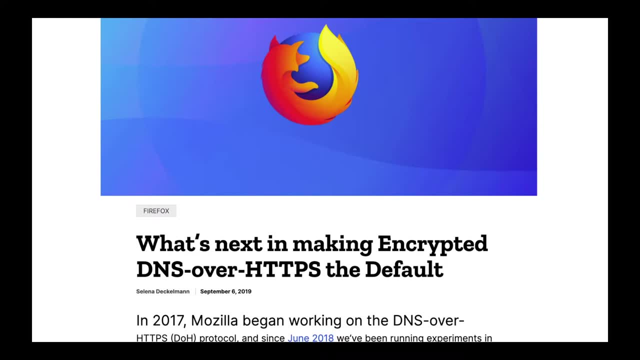 still save that information anyway. That's. that's the problem we're trying to work around here. So the solution to that is this thing that is called DNS over HTTPS, And the idea there is: well, let's just make a connection that's secure, that's encrypted. 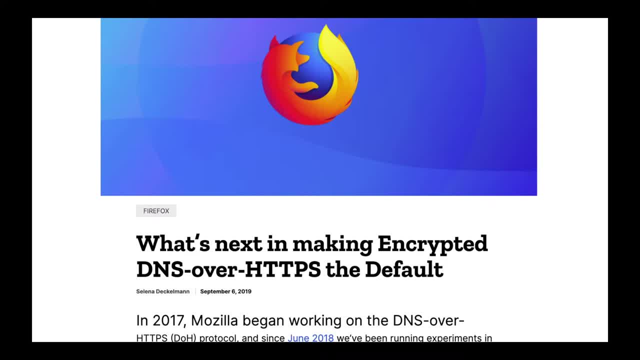 and then we'll send our query and get a response over. that Um and that sort of sort of solves this problem, And Firefox just made this the default, So that's really nice. It's not. it's not getting Chrome or any of the. 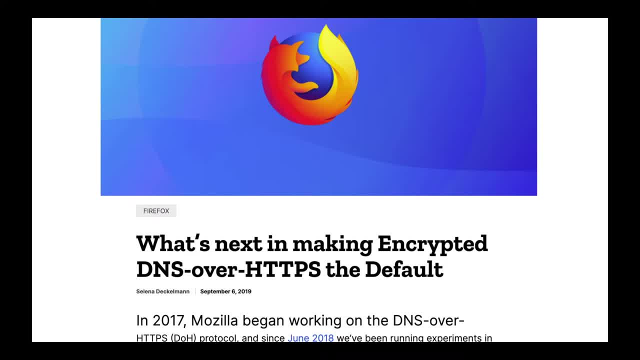 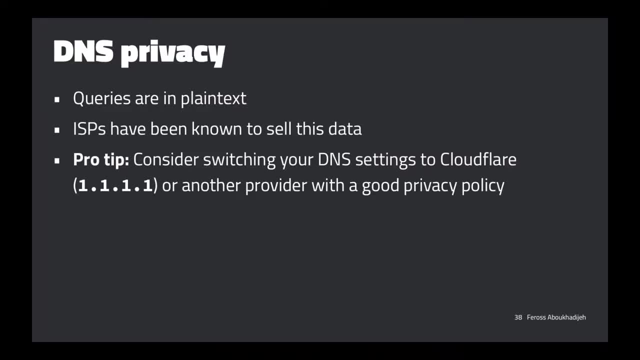 other browsers, though some of them are starting to test it out. But yeah, this is really cool, And the reason why this is particularly cool is that, even if you change your own operating system's settings to use this provider, here you know. 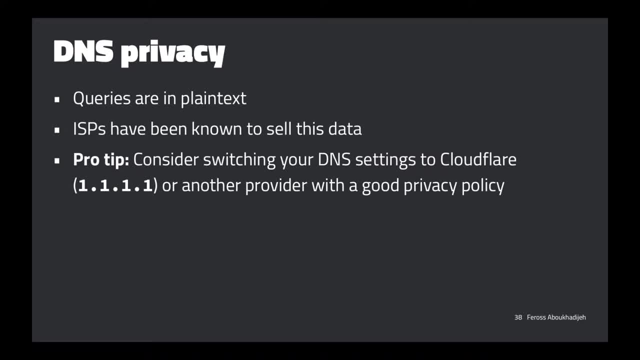 you end up, the query still goes over. you know unencrypted, So you want to. you want really DNS over HTTPS for your whole computer, but MacOS and Windows don't support that, So the next best thing you can do is just have the browser do it. 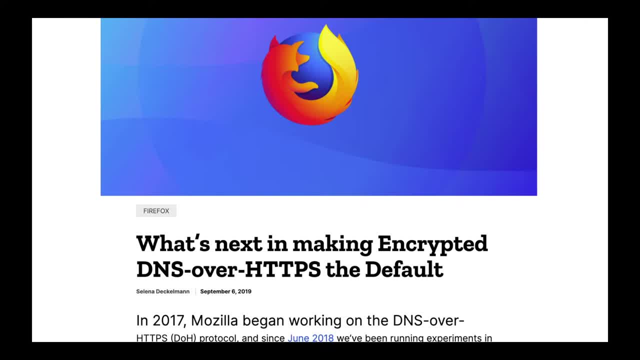 Um, until that's, until that's supported. Cool, Somebody had a question. I was just wondering what exactly is Cloudflare, and is it a free service? Yeah, they're a company that provides CDN services, so they basically take your site's content and can put it on. 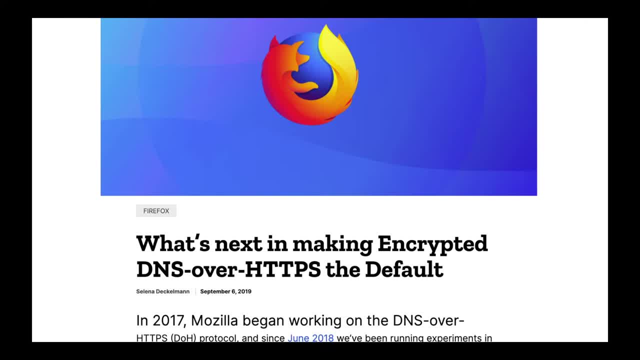 servers all around the world so it's faster, And then they just sort of provide a bunch of these other add-on things like DNS, Um, and it's a good question like: how do they provide this for free? It seems like there must be some game going on. 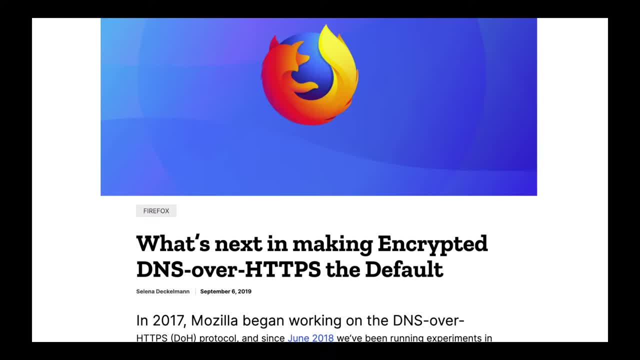 there. Um, I would- I don't know, just do your own research and see. But I think they're legit. They seem good. But yeah, Does DNS erase TCS using TCP? Uh, yeah, I believe it does. Yeah, so I think the reason why you're asking that 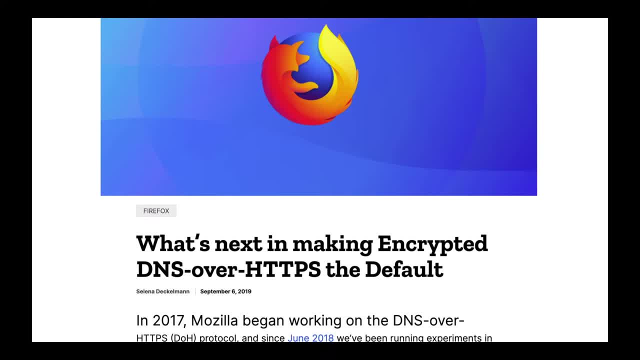 is because DNS is UDP based. Yeah, this would be using TCP, That's right. Yeah, But it's kind of different, Mm-hmm, If I chose people on my network but not anybody else like I should like. 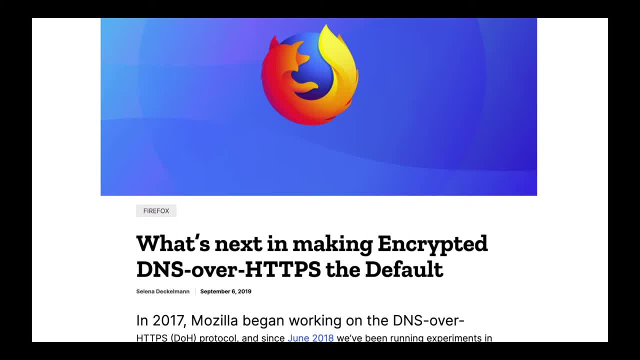 what's it often like for like my router. If I just want my router to do the actual DNS and then respond to me, Mm, Yeah, you could do that. Yeah, so you can set up your router to actually do. 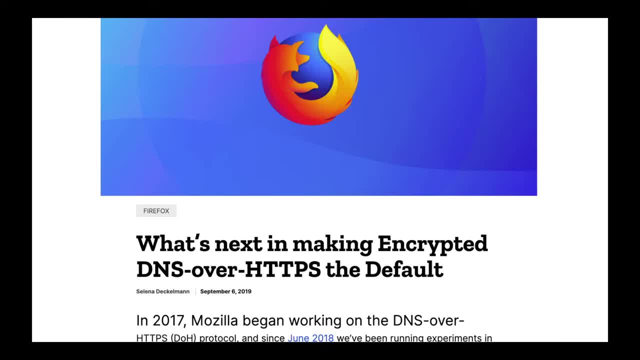 DNS over HTTPS, and then everybody who's after your router won't be able to see it, but then your local network will. it'll be whatever people are using, so you might reveal it to them. yeah, Cool, cool. So now let's. 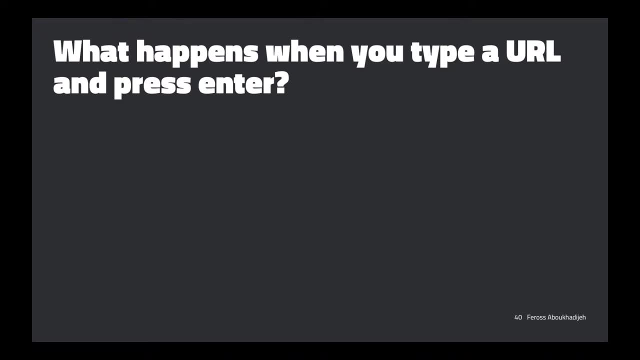 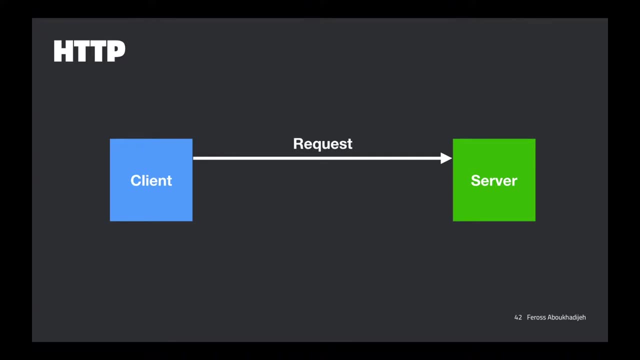 look at our new picture. So what happens when you type in a URL, or let's get back to that question, I mean, and so let's focus specifically on the HTTP part again. So we have, so now we have our IP address. we know what it. 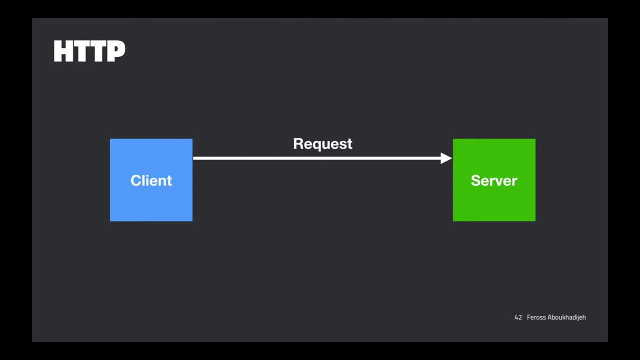 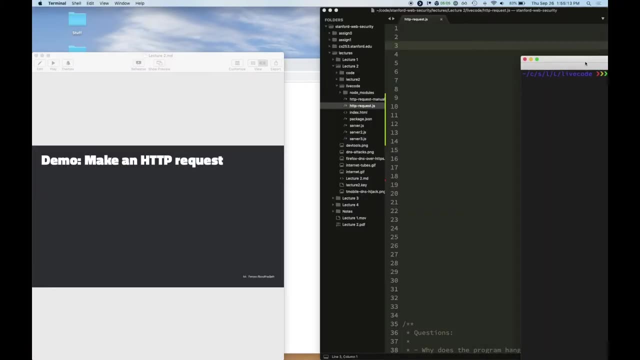 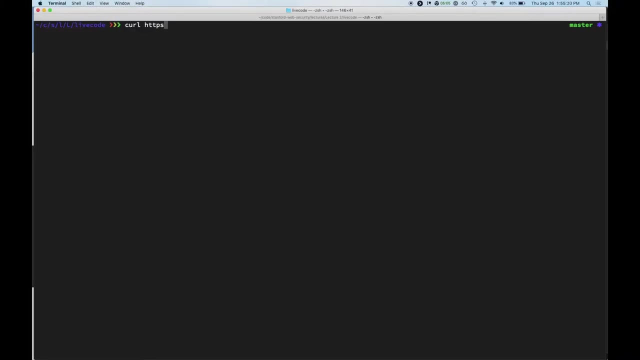 you know, we know who we're trying to talk to. our browser makes the request to that server and it gets back a response. So this is something you've all seen or done before, but we're going to just make a request here to here. I'll make this bigger. 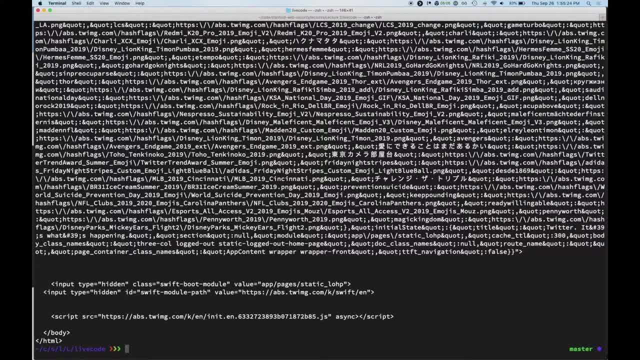 to Twitter and we can just see. that's an HTTP request that we sent and we're going to see. we just got back a response. Is that big enough for everybody to see? Yeah, So that's just. we're just making an HTTP request there. 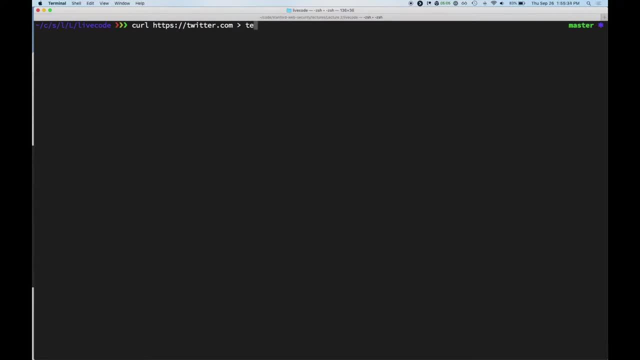 If we want to actually view that, we should probably save it to a file. Here we go, save it to an HTML file and now we can open that up and we can see that we actually did. that's what we downloaded. 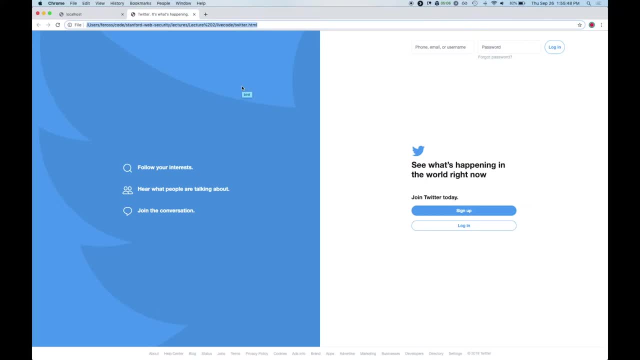 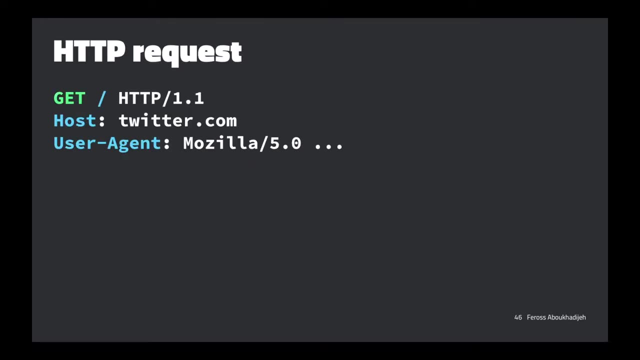 And we can see the URL there is off of my file system here, so that's pretty cool. So, yeah, HTTP requests nice and simple, So that's what's actually getting sent over the wire. so that's just some text, And 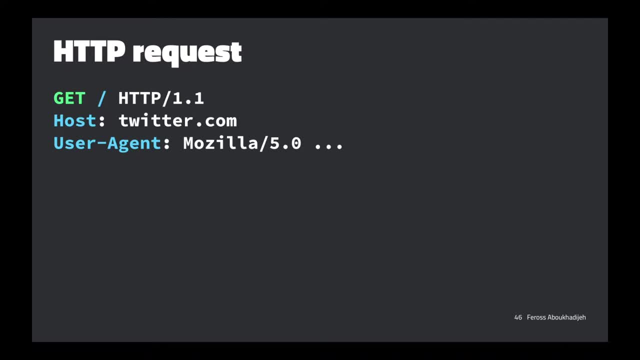 there's just a couple things to point out. The first line is the thing that actually explains the request and the file we're trying to, the resource we're trying to request, and then we have these headers, which are just key values that are underneath it. 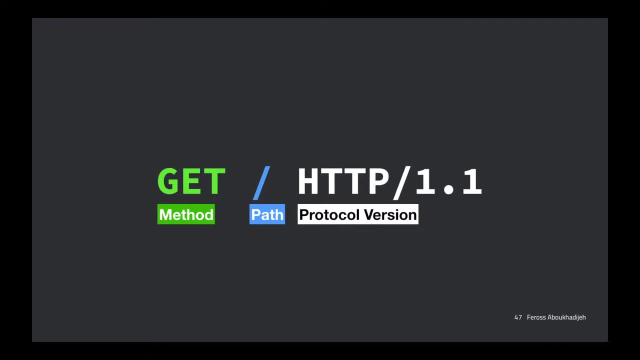 So the first bit is called the method. The method is often going to be get, but there's also a few other types: post put, delete. am I forgetting any? There's a few others, I think, And then we request a path. 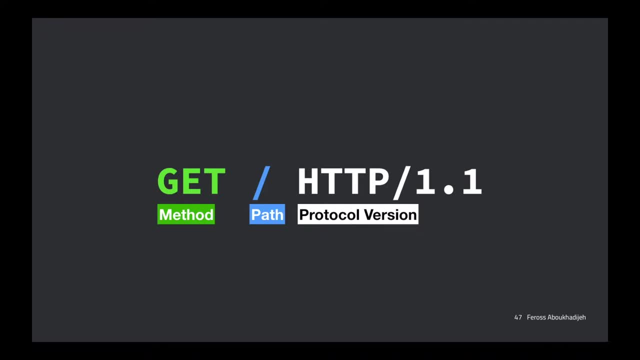 and then we say what protocol version we're using. It's usually just going to be 1.1.. There are newer versions of HTTP, like 2, and there's even 3, which is brand new, which is crazy, because 2 just came out. 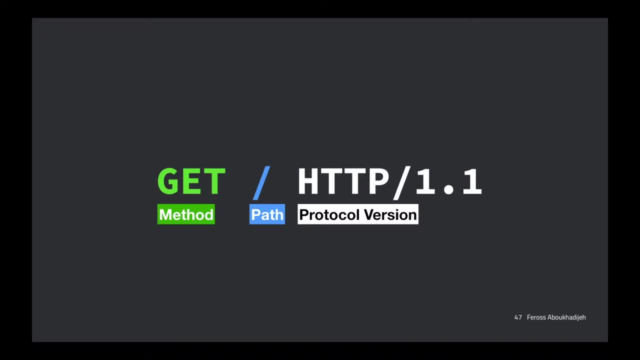 Before that we had 1 and 1.1 for like 15 or 20 years, and now, all of a sudden we have HTTP 2, and then, a couple years after that, 3, so the pace is picking up, But 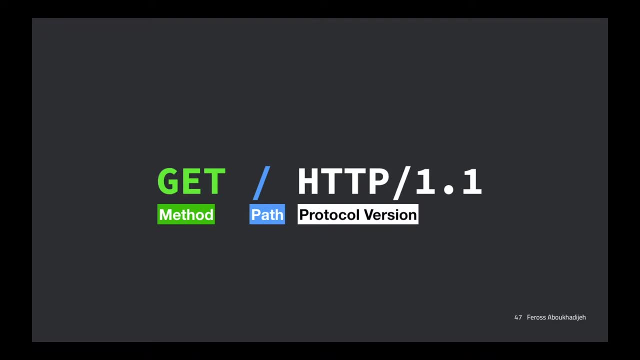 the good news is almost everything still supports HTTP 1.1., which is the version that is most widely deployed. and this is a really nice version because it's all plain text, so you can just type these requests out in textual form. They're very easy to read. 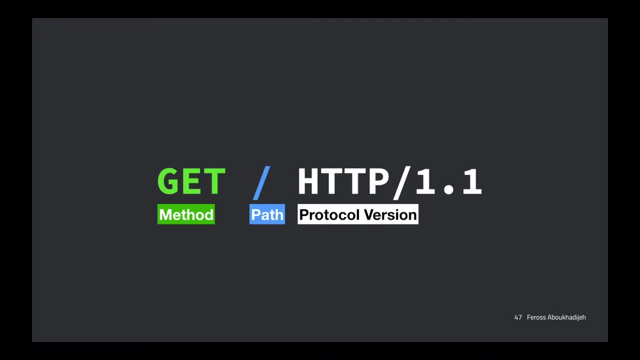 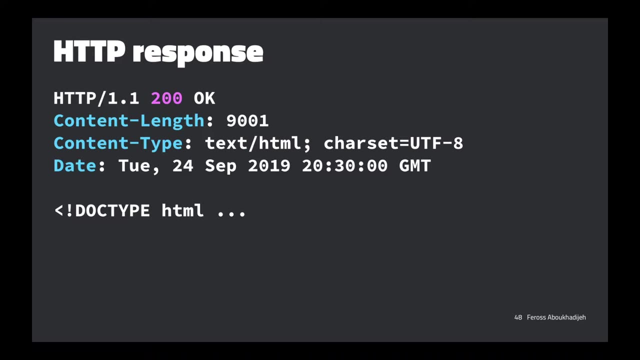 That's not the case for the later versions. Cool, and then, once we send this to the server, the server's going to send us back a response, and our response is going to be a file that we actually want to view. In this case, it's this HTML here: 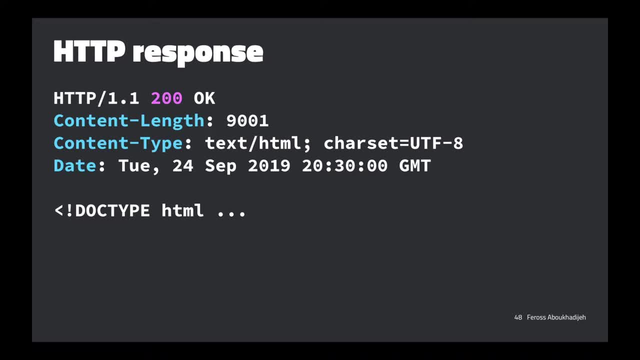 that I cut off, but it's also going to be prepended with some information, some metadata And yeah. so let's talk a little bit about the yeah. so this is just the first line, so again, just confirming that it's speaking the same protocol. 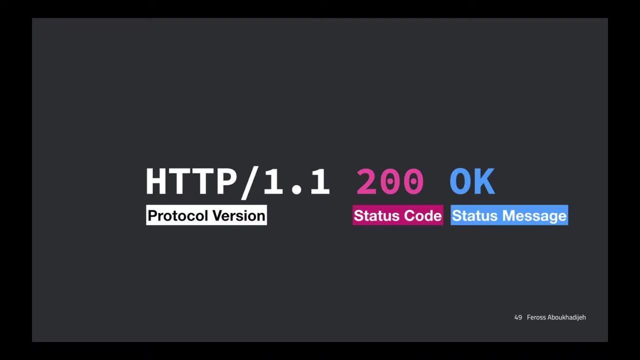 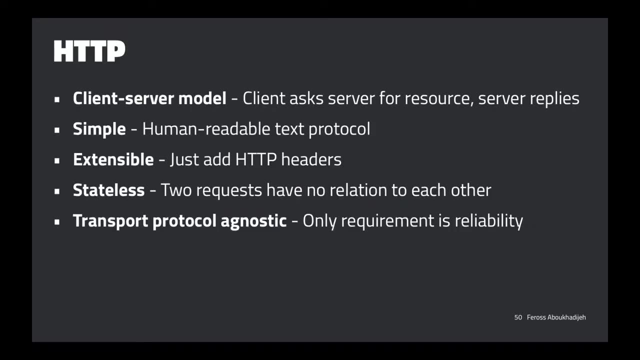 and then there's this thing called a status code. This is probably a review for all of you, because you've all hopefully taken web class, but we have these status codes and these messages and yeah, so let's talk a little bit about HTTP. Why? 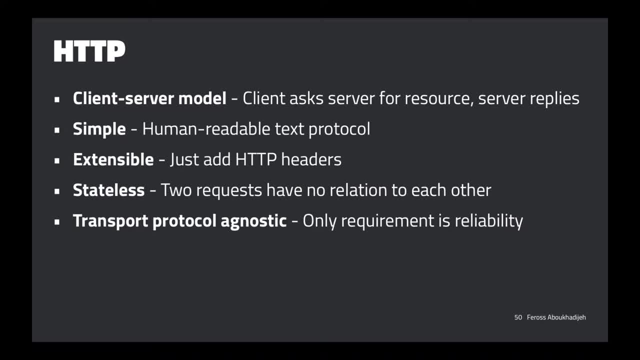 is it cool. So we have the client-server model. We have a client asks for requests from a server and the server applies. It's nice and simple and, like I mentioned, you have this simple textual protocol. so it's very sort of. 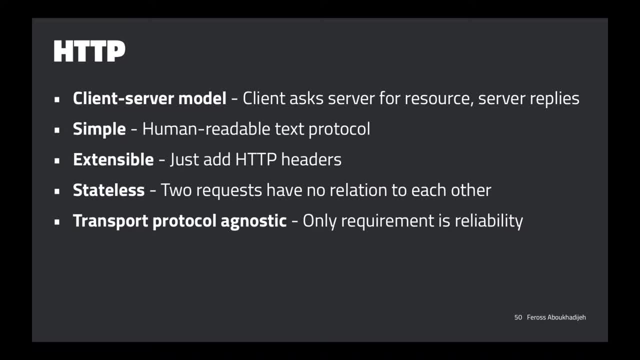 easy to read and the headers are really cool because they enable HTTP to be extensible so you can add new features without having to change. you know, get everybody to agree on a new addition to the protocol. You just sort of add a new key and value and if the server 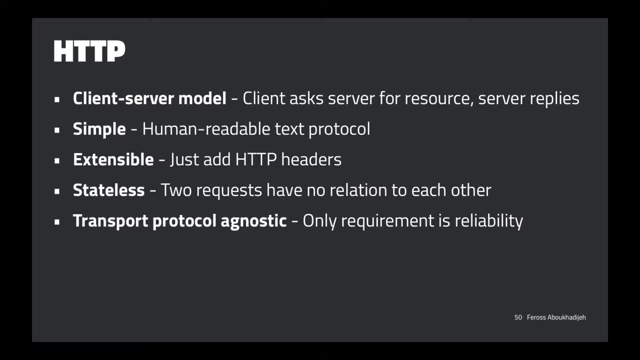 doesn't understand it, it just ignores it. right? That's pretty cool And it's also stateless. So two requests that you make, one after the other, have no relation to each other. And last thing is, it's technically transport protocol. 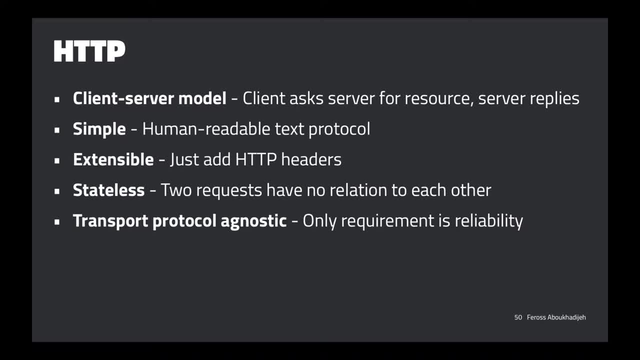 agnostic. What that means is basically that you can do HTTP over any kind of communication channel that you have. It doesn't have to be TCP, although TCP is what we typically use, because that gives us like a reliable connection between two nodes on the internet. 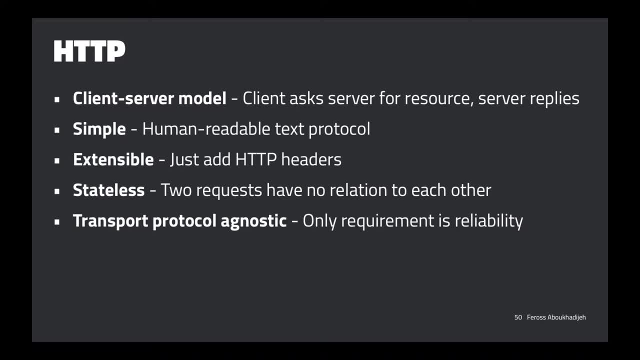 Cool. so any questions about this? Yeah, So isn't the property of being stateless kind of like up to the server to enforce? Does it have a server that I don't know that doesn't expect stateless requests? Yeah, that's right. So if you wanted to, you could. 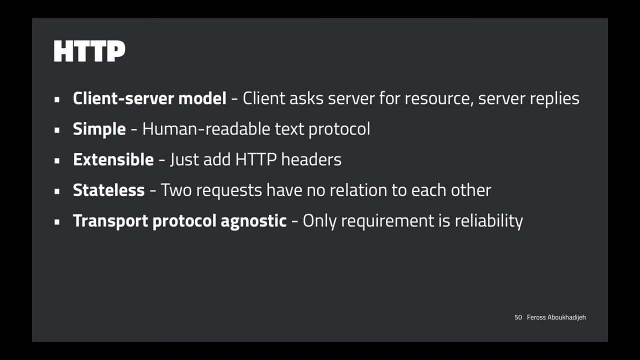 make your requests. you could make the order matter, or something. You could have a server which is like: okay, every tenth visitor is going to win a free prize or something, and I'm going to count the requests, and then, of course, now there's some state that the server's 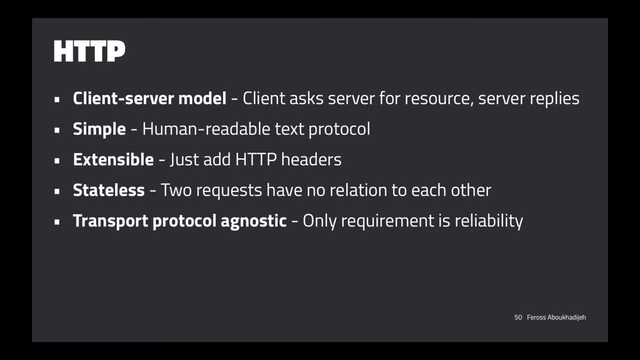 keeping. But the way I would think about it is that you're building that as sort of on top of the HTTP protocol. The protocol itself isn't keeping any state. So if you just say, give me HTTP, you're not going to have any. 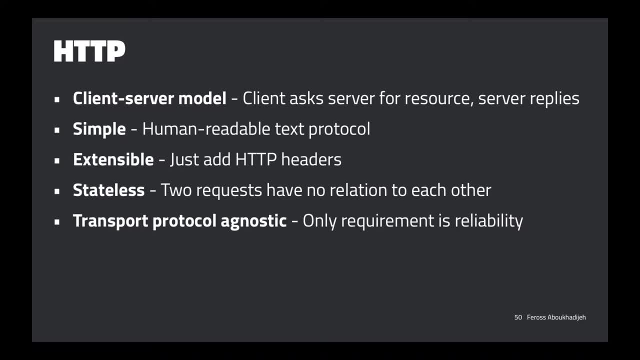 kind of state that's being kept by the server. It's all sort of discarded, And if you want to like, sort of, on top of that, keep state, you can. Yeah, that's a good question though, Because typically, when we interact, 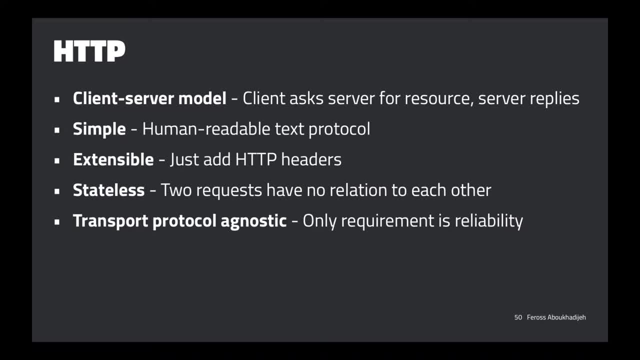 with web services there's some state. I mean, when I click a link, when I log into a website and then I start clicking links, those later links that I click, I'm still logged in, right? So clearly the server remembered something about me. 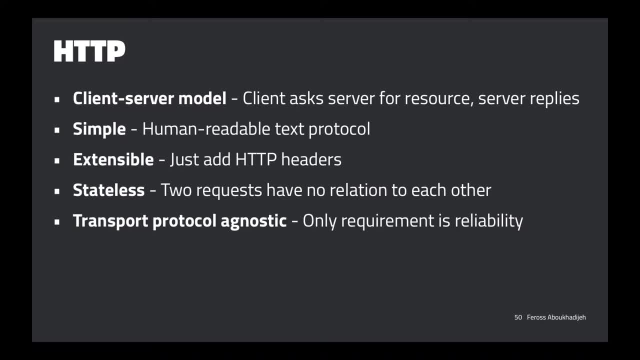 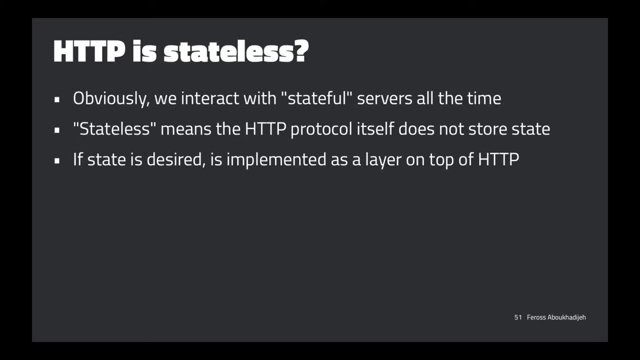 so that I could continue to view different pages and still be logged in. So we'll talk about that at the end here. That's cookies, Cool, Oh yeah, so here There's a slide for that. Yeah, so HTTP is stateless. 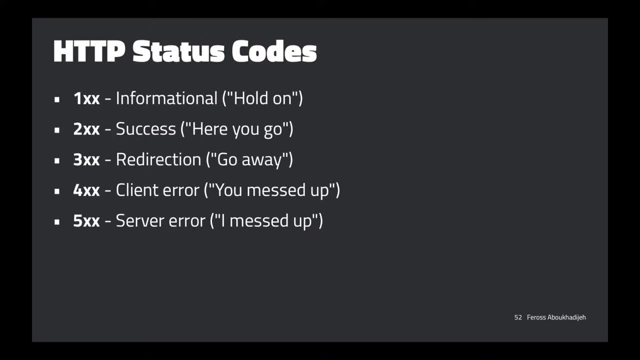 We implement state on top- Cool, So just this is probably again a little bit more review. but we have these different categories of status codes, So everything in 200 is what you're going to see. a lot of That's basically. 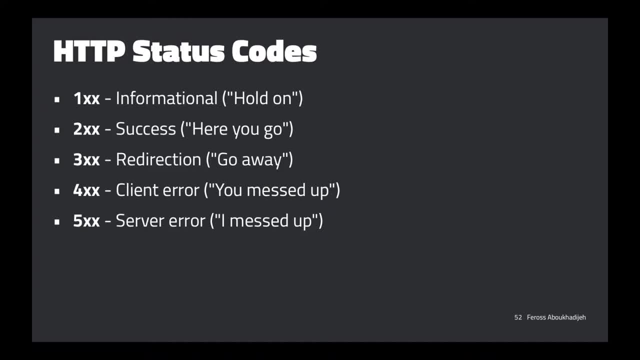 the server saying that your request that you made succeeded. Anything in 300 means that we're redirecting the server's redirecting you to another destination. 400 means that you messed up And then 500 means that the server messed up. That's the best way. 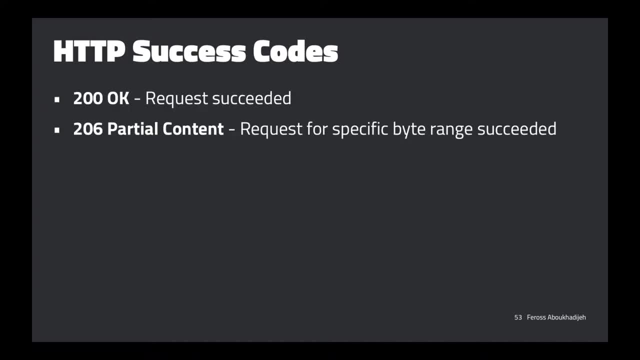 to think about it. So yeah, just a few highlights of the most important status code that you'll see. Something fun. It's just a less censored version of your last slide. I saw on Reddit the other day- Oh really, And I just saved a picture for it. Oh, is it like you effed up? 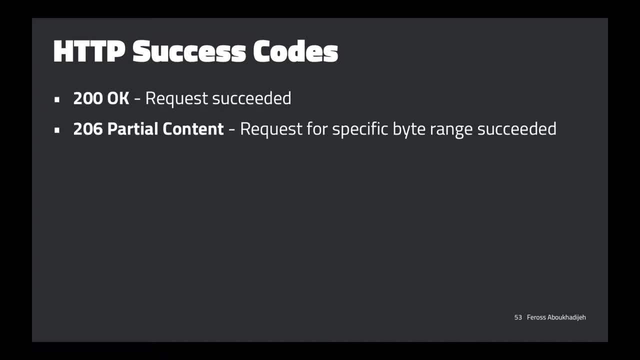 or something. Yeah, I've not seen that one Anyway. So yeah, there's two main types of successes. So 200 is the most common, But there's this other one called 206, which is given in response to a range request, So you can make a. 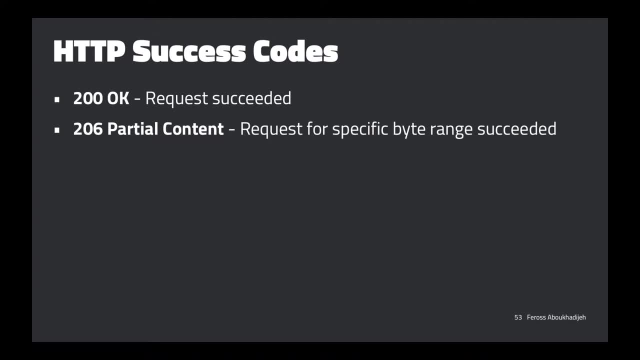 request for a partial subset of a resource And then the server can say, okay, I'll slice that part of the file off for you and give that to you. Can anyone think why that's useful? Where would that be used? Hmm? 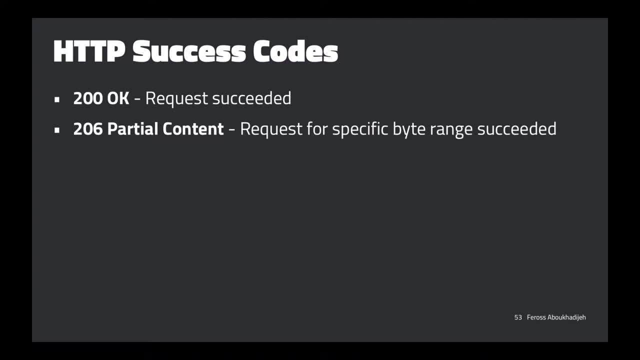 For parts of, to give you small parts of the song so you don't get the whole thing. Yeah, that's right. So say you wanted to seek to the middle of a video or a song and you just click in the middle before. 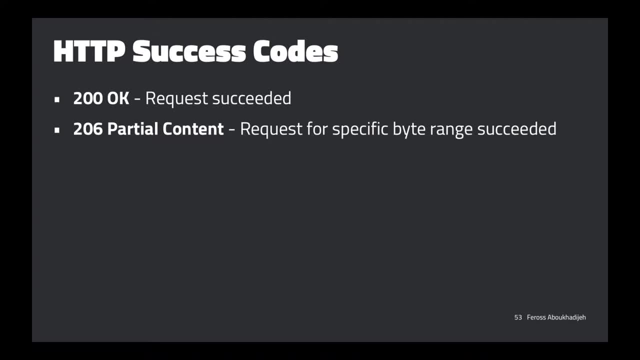 the browser's actually downloaded the whole video file. It would be nice if the browser could say: I know I want this file, starting at byte offset 100,000 or something, And then it can make that request to the server and the server can respond and say: okay, there's the piece. 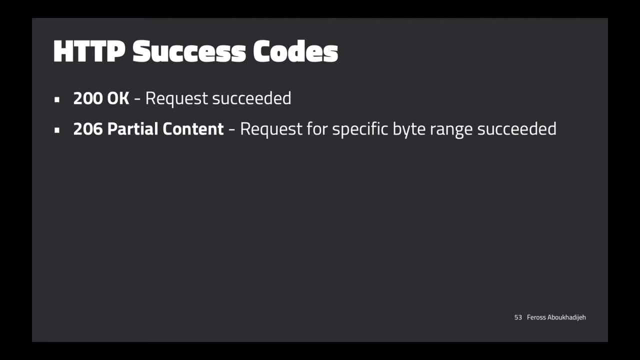 that you asked for, So you don't have to wait for the whole file to download sequentially. That's really useful. So that's called a range request. Yeah, and 206, the reason why we do 206 responses there is because say that you make a range request. 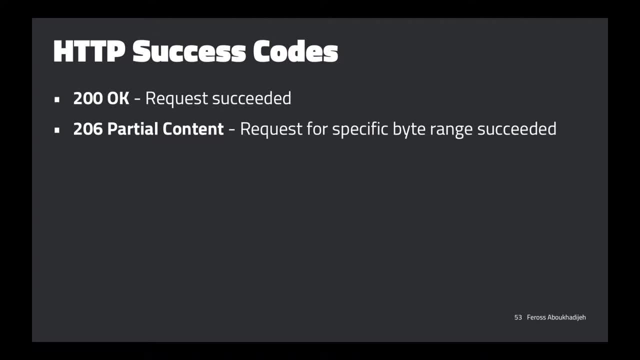 to a server and the server doesn't actually understand range requests Because, remember I mentioned, you can add these headers and the server might not know what the header means. It might be like a simpler server If a server doesn't understand this range header that you tacked on to your request. 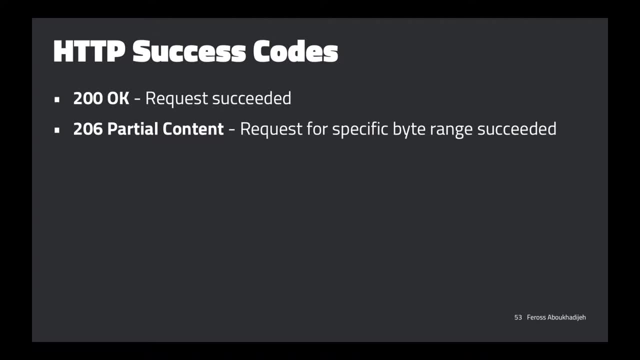 it will, just it won't know what to do with it. So it'll just respond with 200, and here's the whole file, And then your browser needs to be able to know. oh okay, I was not expecting a 200,, I was expecting a 206.. 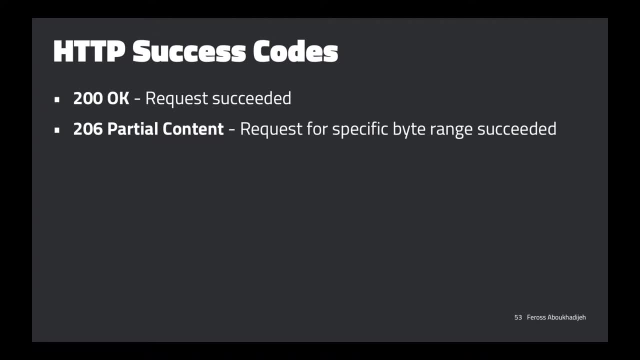 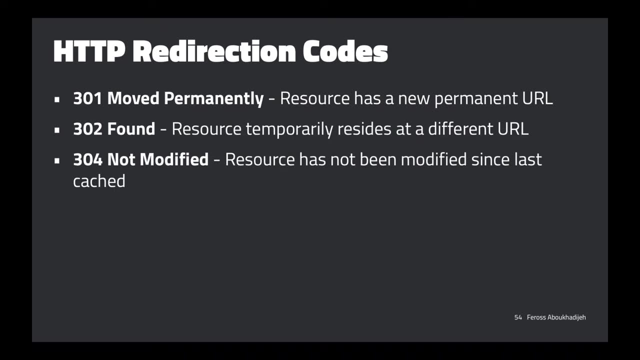 So this is clearly like a server that doesn't know what I asked it And you need to sort of adjust your behavior according to that. Cool, So then some 300s ones. so there's 301, 302, which basically are just a typical standard. 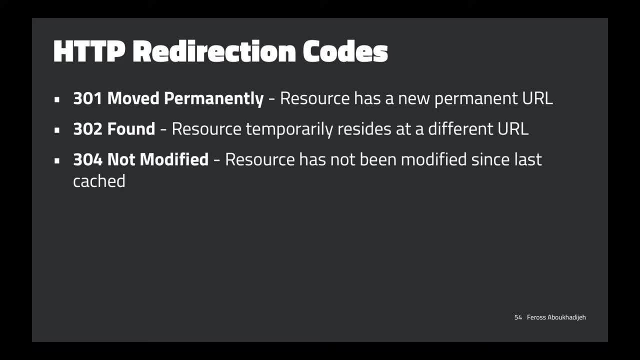 redirect to another URL. The difference between them is that if you do a 301, actually does anyone know the difference? I mean it says up there, but what is the actual behavior difference when your browser gets a 301 versus when it gets a 302?? 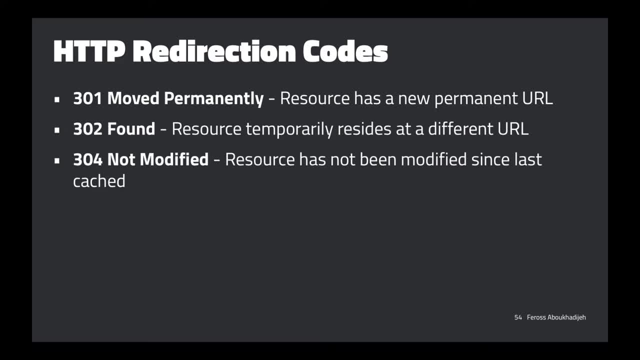 What is it going to do differently? I mean, can you just, maybe it's okay, you can just guess: Yeah in the back, Yeah, that's right. So it won't even bother checking the original URL. So, if you like, 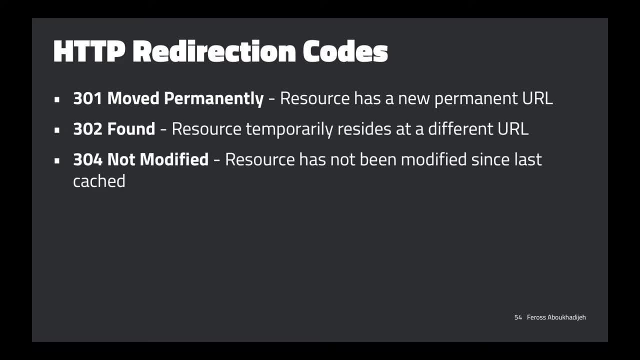 reload the page, or you? yeah, it's basically saving an association, Like when I see this URL. just don't even ask the server. The server told me it's permanently at this other place. I don't have to, but if it's temporary it's going to. 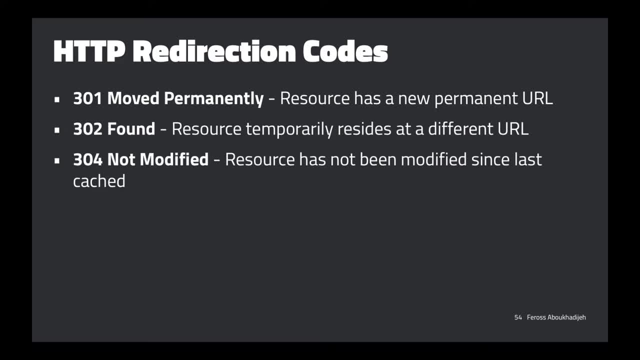 ask it again, because it could be that now it's in a different place and every time you ask it it's going to give you a different place. So actually, I implemented some random functionality on a website that I have, and if you do with a 301, it doesn't work. 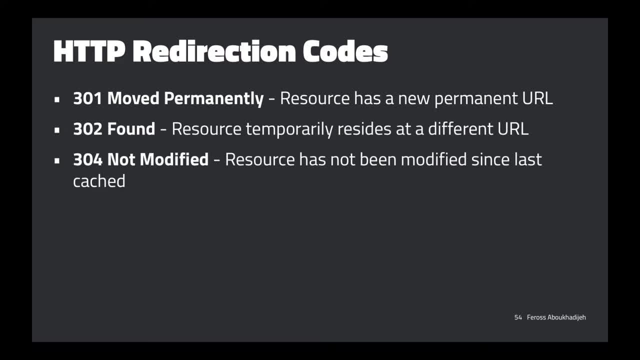 What you want is like every time the user goes to slash random, you want to send them to a random page of the website. If you do a 301,, then any time they click random, it's going to just take them to the first one. 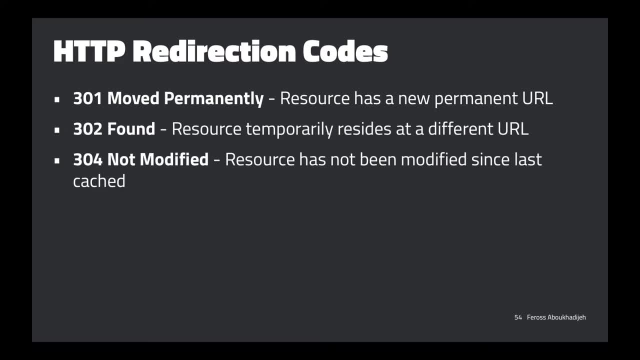 that they got sent to right. So that's an important difference. for that kind of functionality, Cool Yeah. and then for 304,. this one is: this is used when the browser has cached a resource and it wants to tell the server: hey, this is a. 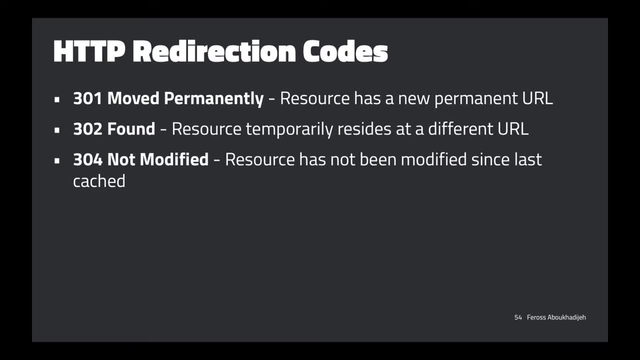 file that I already have, but this is the version of it that I have and tell me if only respond if it's changed, So you can make this sort of conditional request where you say you know, so you're either going to get back a 200, which means 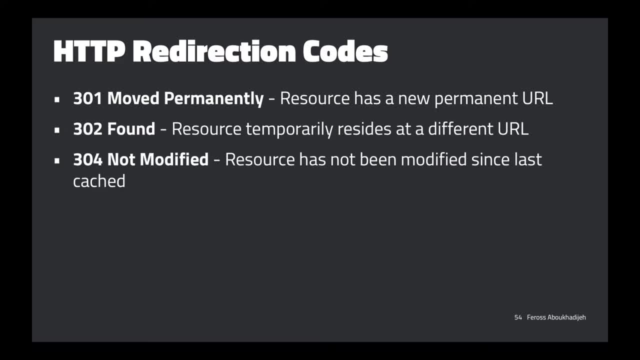 that the request has indeed changed and the server is giving it to you, right? Or if you have the current latest version, then it will respond with a 304 and say it hasn't been modified since you last got it. you do have the latest. 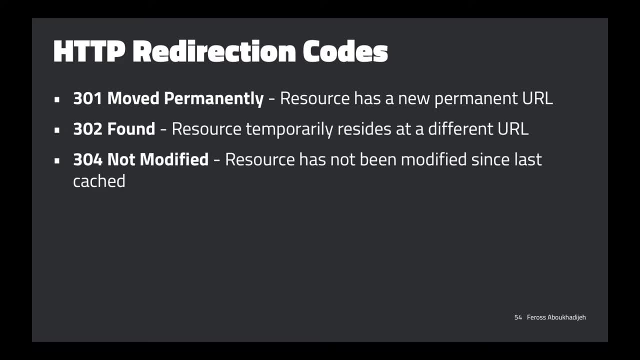 version and it won't actually send it down to the browser, which just saves some time and bandwidth for us. Cool, Any questions about these? Yeah? 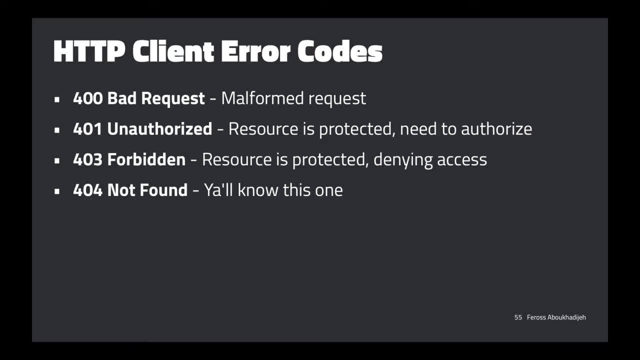 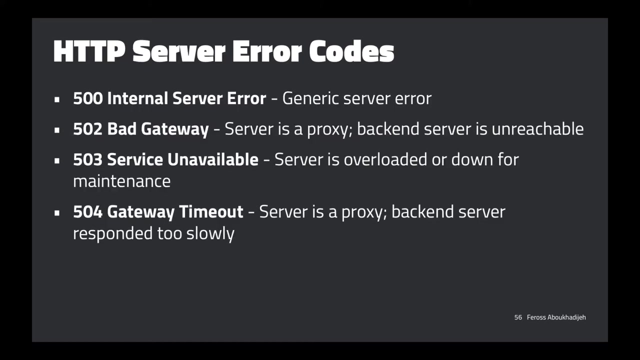 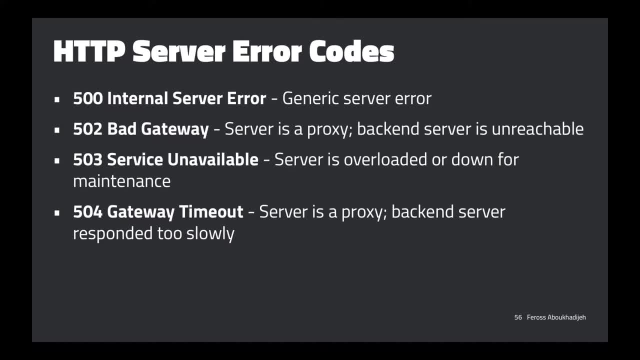 in between. um, i actually have a picture of it, i think, somewhere here. um, there it is, yeah, so, uh, yeah, so you can have a situation where back here you have potentially hundreds of different servers. 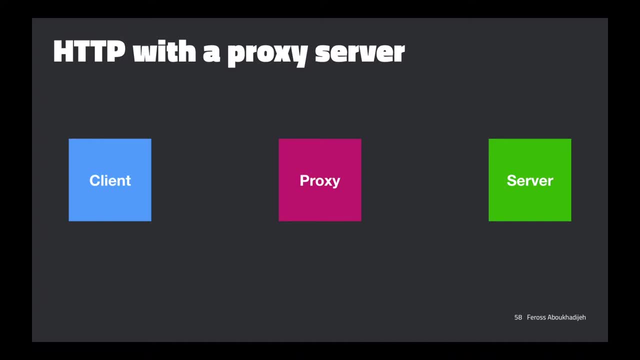 this is how big web services scale and then, um, the user doesn't know about like which particular server they're talking to, but they send a request to, to the main server and that server proxies, through the request to, to a back-end server. right, um, and you can imagine, a lot can go wrong at this. 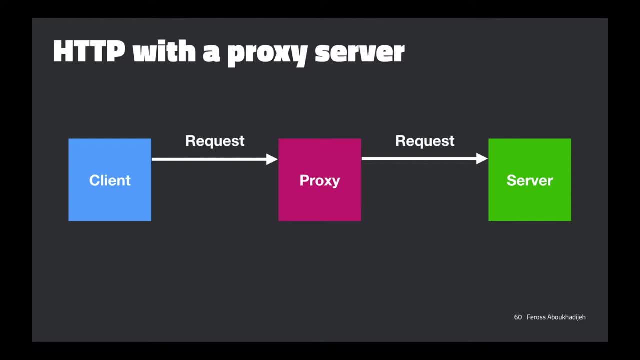 stage here, right? so what if the server that the proxy sends the request to is down? um, how long should this proxy wait for a response, right? what if, um, there's all kinds of different ways this can fail. what if, um, yeah, so it could be that the server is online, but it's- it's behaving poorly. 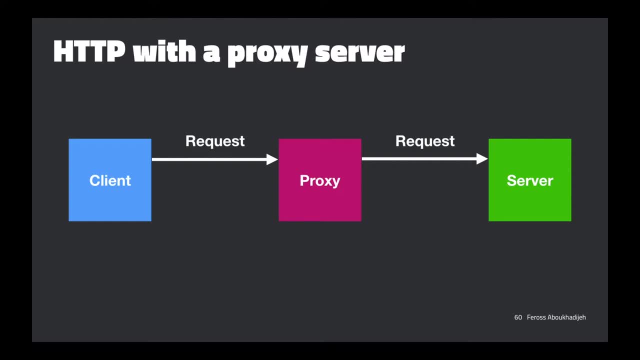 so it's like really slow, right, um, and maybe we want to configure the proxy so that, um, it has a timeout where it will just give up after a while because it doesn't want to waste one of its connections on this never-ending request, and so there's all kinds of ways it can fail, and that's that's why we get those different codes. 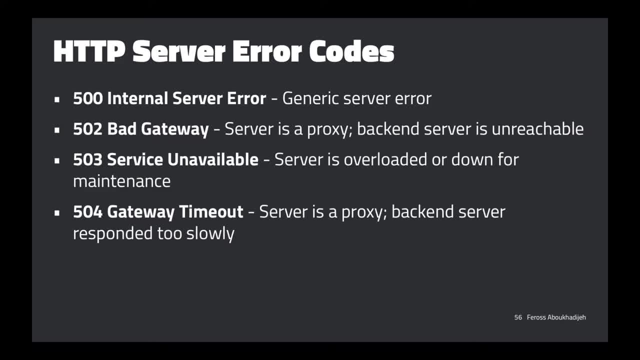 there. so, like bad gateway is um the server is down, service not available means it's it's um temporarily down or overloaded, and then timeout is it took too long, basically, and there's there's a bunch more of these, but so so why do we have these special codes, code numbers, what's the point? 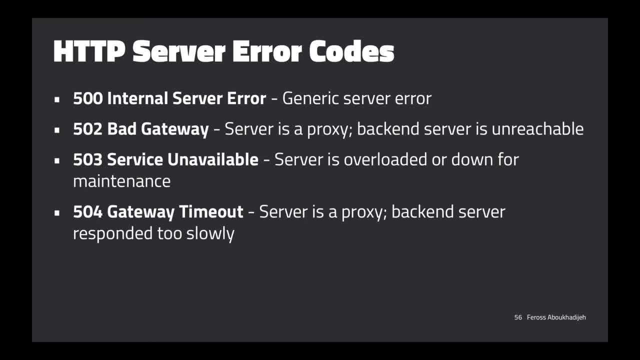 like: why can't we just put a message in the response that says what went, what went wrong? why are we also adding a number to the response? so it's easier for programmers to like code how to do it. so it's easier for programmers to like code: how to do it. so it's easier for programmers to like code how to. 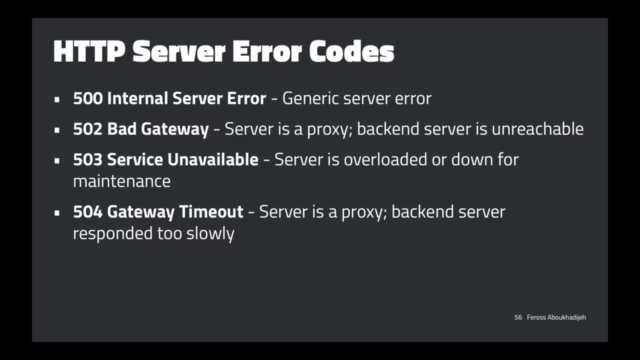 deal with these different things. it's kind of standardized so that like if one server says server is a proxy, like whatever, and another person says that, but with synonyms, you don't have to like do natural language processing exactly, exactly yeah. so like if i see that i got a 404, i won't. 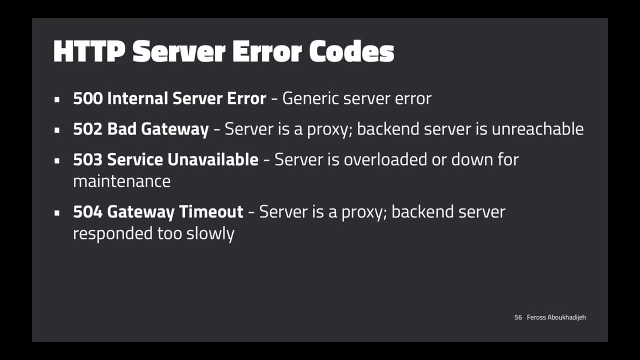 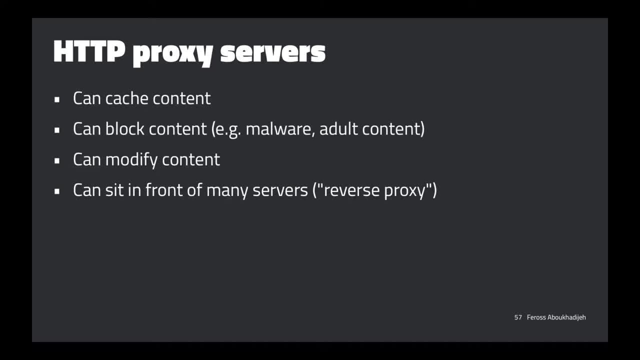 try that again. like it's, the resource is not there. if i get a 500, maybe i'll try that again. the server had an exception, i don't know. maybe maybe it'll work later, right, but um yeah, the errors tell you different things. cool, um yeah, and then these proxies are used for a lot of different situations. 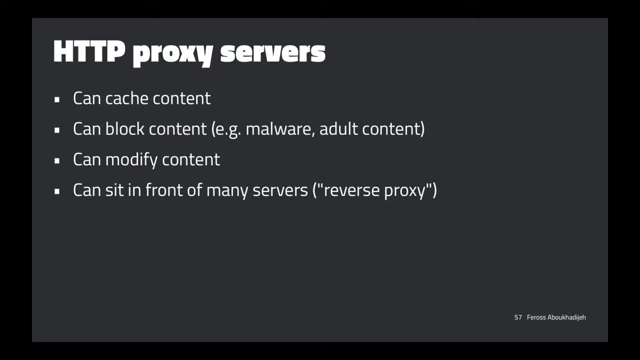 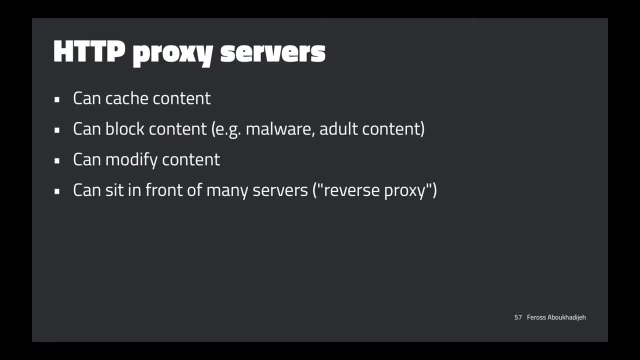 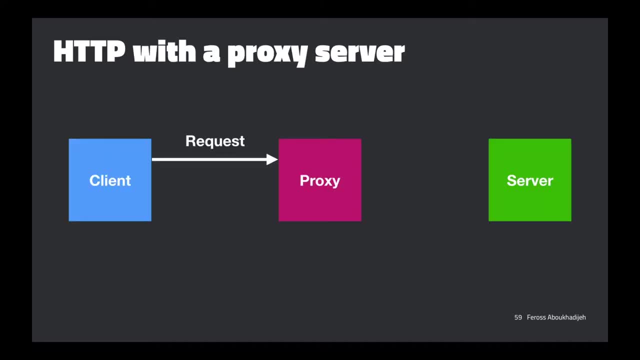 you all know about proxies, um, but the kind of proxy you did in 110 is a client-side proxy, so that was a server, that sort of um. uh, it does the exact same thing we saw there, but this is not. this proxy is not run by the company that owns all these these servers back here. 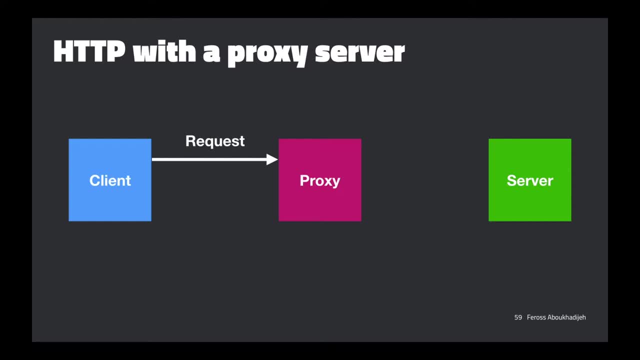 it's rather it's run by, um, like it's a program on your computer, or maybe it's run by your employer, so your employer can filter out certain types of websites so that you you can't get distracted at work or whatever. yeah, uh, leave it at that. 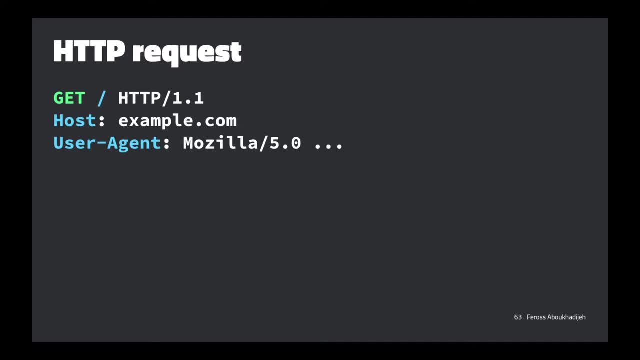 so okay, so back to http requests. um, yeah, so i want to talk about headers now. um, so, we have a couple here: the host and the user agent, but the general format is it's: it's a name and then a colon and then a value. um, that's how it. 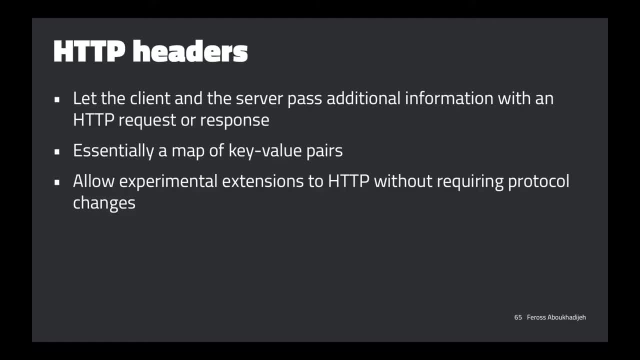 works. uh, so these look the. the client and the server pass additional information. that's not actually part of the. the rest of the server, that's not actually part of the, the rest of the server of the, the response, um, and it's basically a map of keys and values and, like i said before, it's 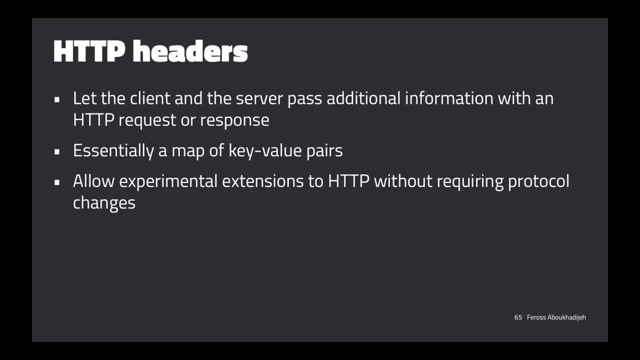 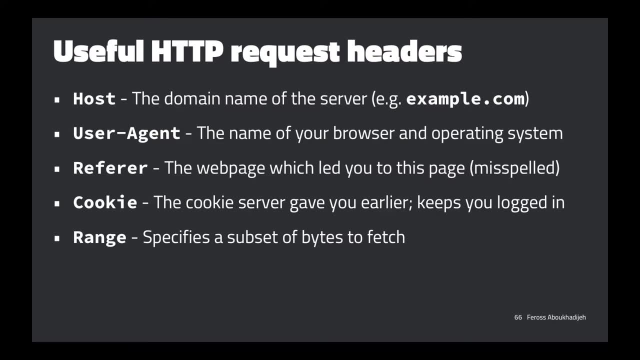 really cool because it lets you just sort of throw in additional headers in there without getting all the browsers and everybody to agree on on changing http. so just a few um highlights of useful ones that you're going to run into that you should know. the first one is host. that's the. 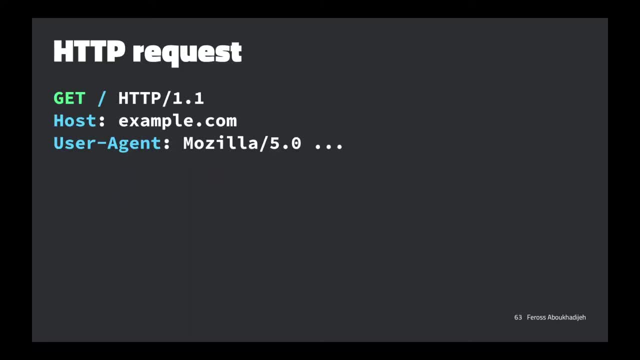 one we saw before. that was the one that was right there saying host examplecom. that one's really important. most servers won't even respond to you if you don't include that. so that's just the name of the host examplecom. that's the one that's really important. most servers won't even respond to you if you don't include that. um, so that's just the name of the. 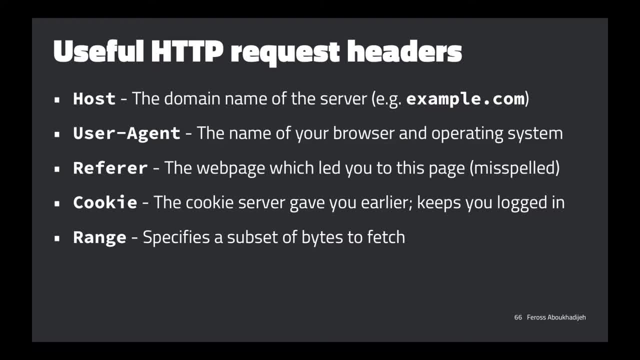 uh server that you're trying to talk to, uh, and then there's user agent that is the, the name of your browser and operating system, so that lets the server know who is uh, who's a call-in basically at the server. um, uh, this is actually really useful for um detecting, like when someone is, when a 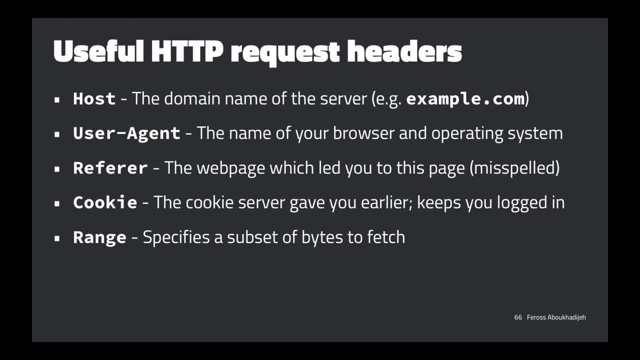 visitor is a search engine. so like, for example, when google requests a website, it'll say: you know, i'm googlebot, it's actually what it's called googlebot- and then the server can know: okay, that's google crawling my website. i can see they're visiting that url and that url and that url and 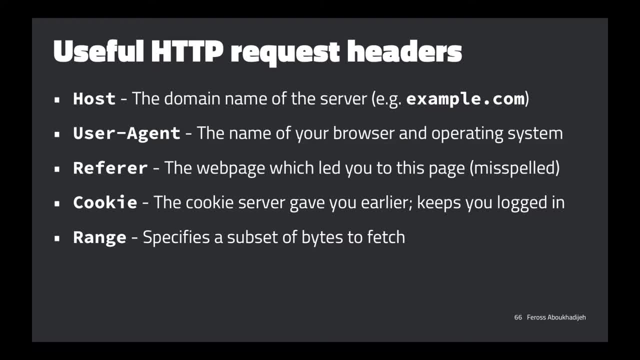 um, uh, and that's pretty interesting. um, you can. just, if you ever have a server, you can just look at those requests coming through and it's fascinating to see the different user agents that are that are visiting your site. you know, you can. really just there's lots of random startups. 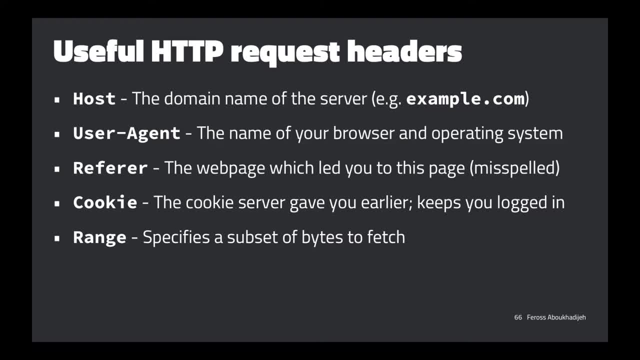 that have like really weird names, that are like trying to build google competitors, and you can see them crawling your website trying to download pages. um, you can see when someone's using curl, like i just did, right, um, and you can actually sometimes use this to to block requests that. 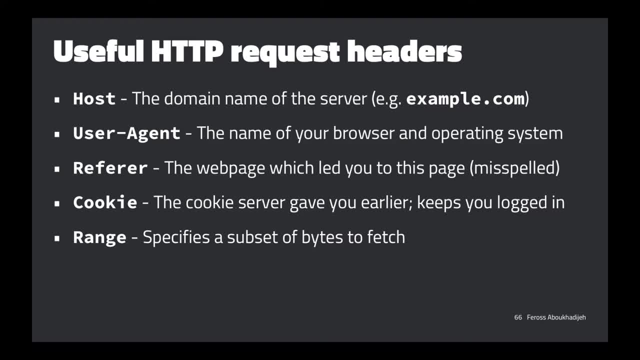 are that? are that look malicious? or if someone's misbehaving? you know, like the other day someone was uh running a thing called like site slurper, trying to download, like my whole, one of my websites, entirely just slurping all the pages down and i just 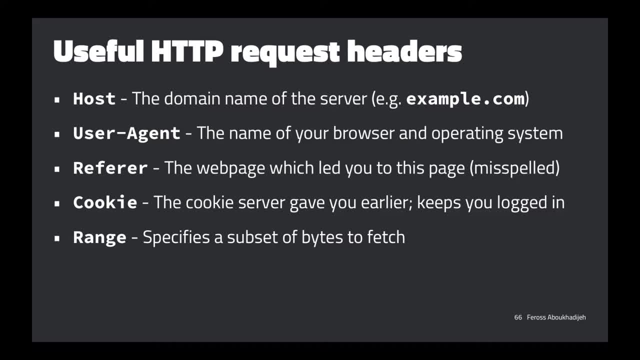 i just said, okay, if user agent is includes site slurper, like no, just, but yeah, anyway, there's some stuff you can do now, obviously, but they can control that user agent header. so it's not that good of a of a defense, but it's, it's something at least. 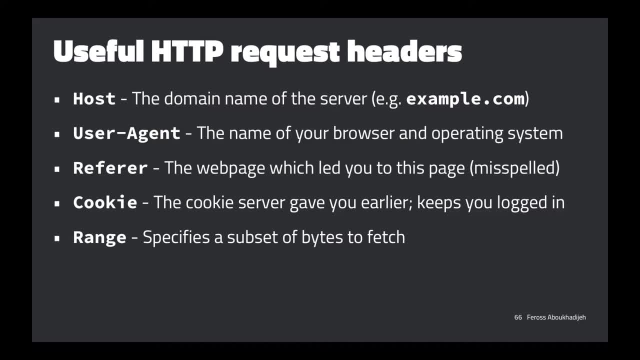 if they're that obvious. um, yeah, okay, and then refer is cool because, um, that tells you basically the page that the user was on before they requested this page, right? um, so that's really interesting that that's how you can figure out, um, like, how a visitor got to your website, um, who? 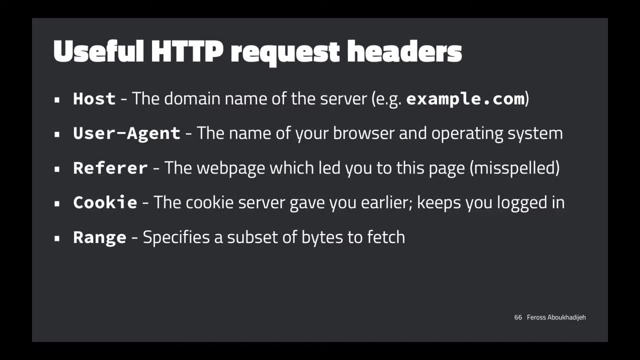 linked them there, basically, and you can see how many people are are coming to your site from from that other destination, um, and then, like obviously notice i mentioned here, it's misspelled- um, so the time when they were making this, uh, the spell checker on, like unix or whatever system, the person 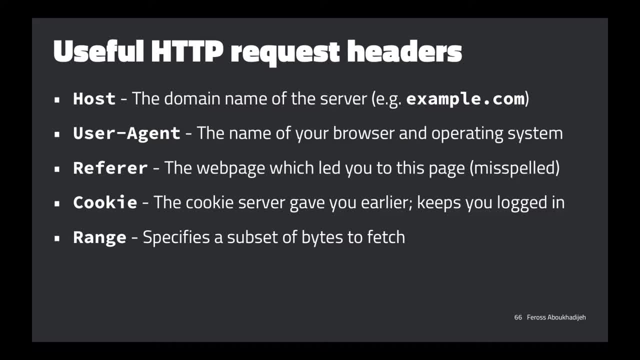 had didn't have, uh, either this spelling or the other spelling in it at all, like it just didn't know about the word refer, so so the person just spelled it wrong and then from then on everybody was like we could change it. but then we all have to change all of our code and we'll just leave it. so now, if you, 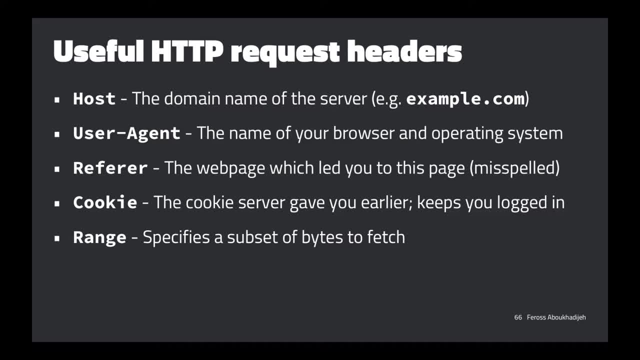 read about http, like all the specs and everything, just just have it misspelled. that's just what it is in http in the http world. that's how refers spelt. yeah, yeah, what was that? uh, that someone said something anyway, but yeah, so it's like um. 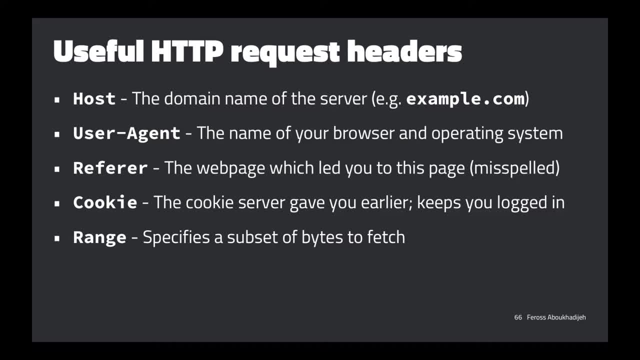 sometimes it's just not worth. it's just not worth the cost, the pain, you know, just for some aesthetic thing. and that's actually the story of the web, honestly, is like anytime they can make a decision to like do things right or do things like easiest, they choose easiest right because it's. 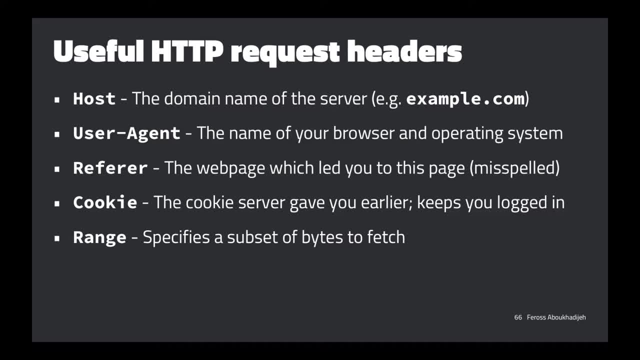 it's. it's better for compatibility, it's better for, you know, not breaking old websites and stuff like that, so yeah, so there's good arguments for it, um, but yeah, it's also kind of kind of gross, okay, and then there's cookies, so we're going to talk. 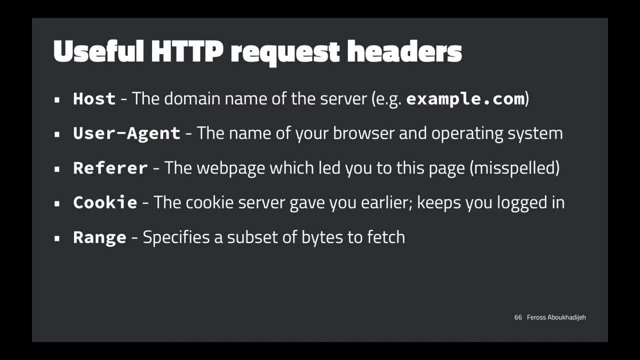 about this, uh, if we have time, hopefully. um, but yeah, so, cookie is basically: it's a, it's a header that you attach to your request and it's basically um, you just it's, the server gives it to you in a, in a response, and then the idea is: once you've gotten that, you just tack it on. 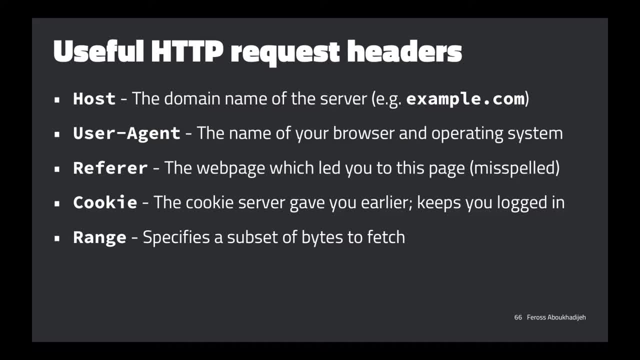 to every request you make in the future, right? um, so we'll see the corresponding one that goes with this. so there's a header that the server can give you that's called set cookie, and then some value, and then when you get that, you basically save that on your machine and then anytime you go to that. 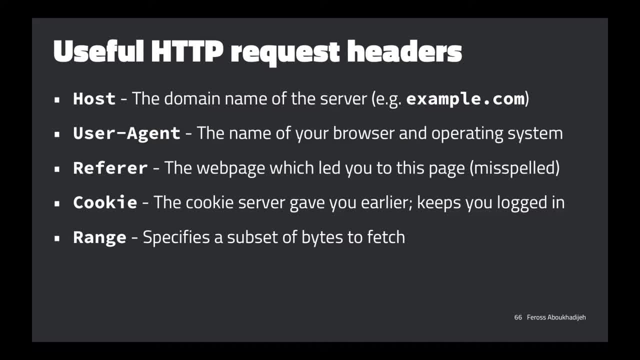 and your browser will just attack it onto the request and say: this is what you gave me before. here's the cookie. okay, and that's how you stay logged in. um, the server gives you some kind of a token and then you tack that onto your requests and then the server's like: oh, okay, that's you. 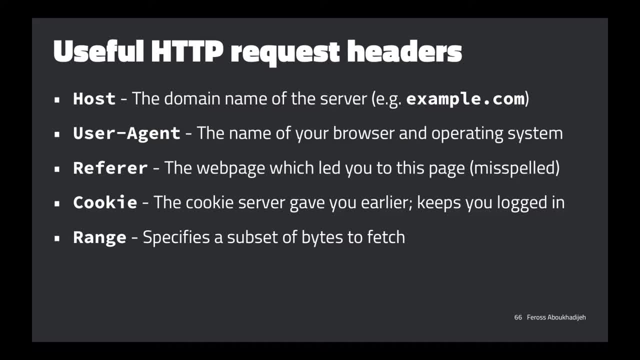 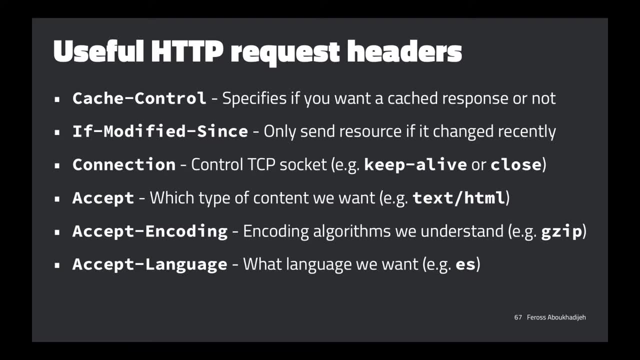 right, uh, and then range. i mentioned that before. so that's how you subset, uh, a request, and then there's a whole bunch more here. um, you know, you can control the cache. you can say, if only give me a response- if it's, if it's been modified since this date when i got it before. um, you can control. 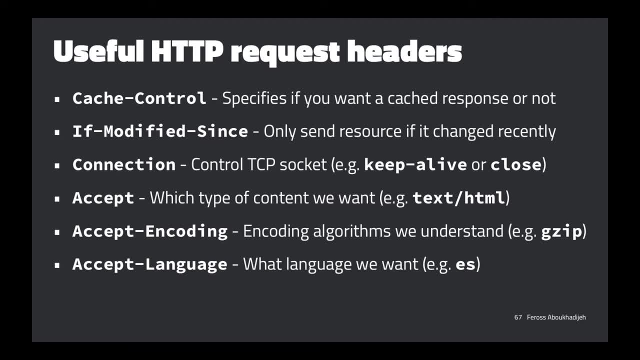 it with a gcp socket. that's kind of crazy. you can say, like when this request is, uh, is finished and i've gotten the response, don't actually close the connection to the server. keep it open, because i might send more requests over that connection. that's a performance thing, um, and then you can. 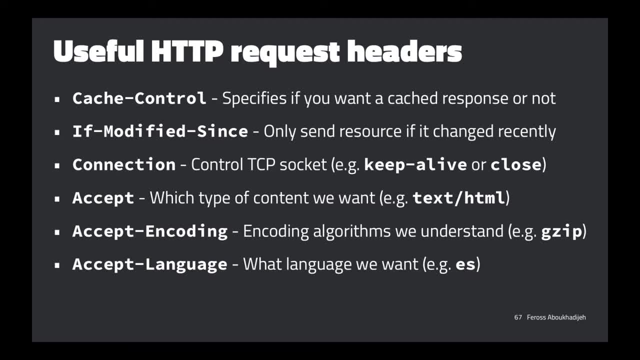 also say like, what kinds of response you can accept. so you might say like: i only want html back, please. or like: if you want, you can gzip the response, which will compress it. you can tell the server, like i understand how to un-gzip it, so feel free to gzip it. 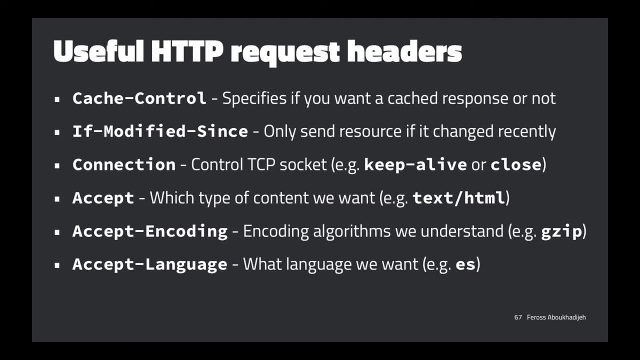 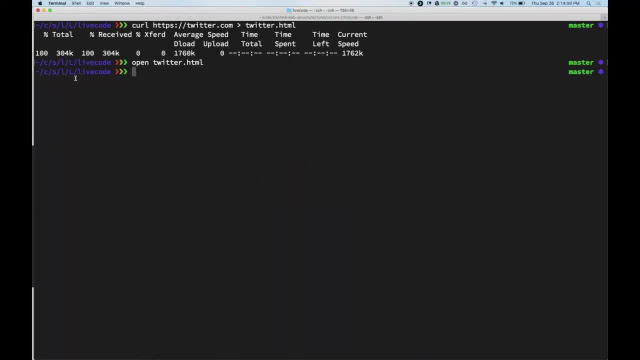 but you can also say: i want a language, a particular language, back and it'll um, it'll, you know, change the paper based on that. so cool, i'm going to show just uh, just doing that really quick so we can actually just curl has a nice um way of doing that. you just say curl um, you say curl uh. twittercom. 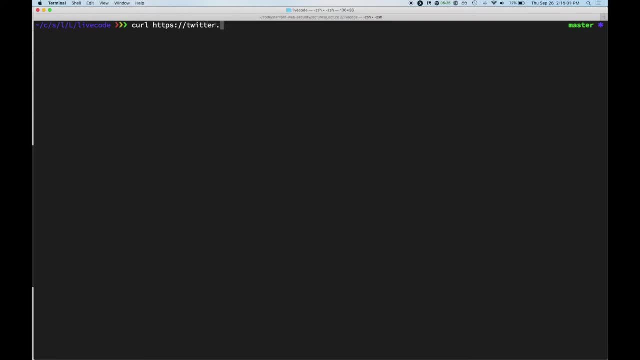 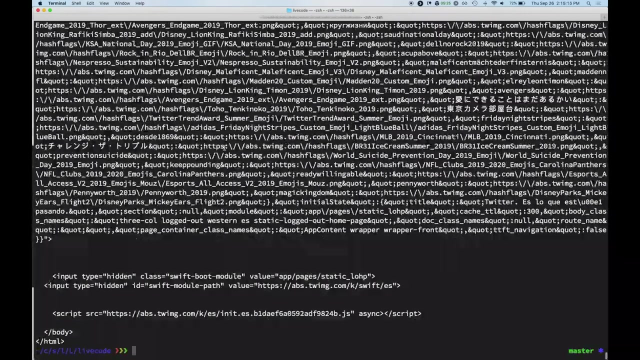 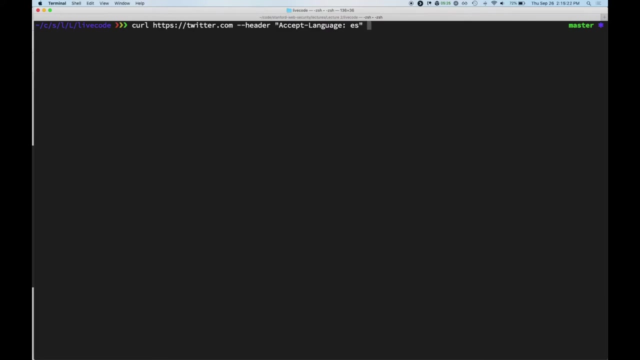 can't type twitter, oh my gosh. okay, twittercom. and then we say header, we can say accept language. so if i do that, um the the the problem is there's all these tags, like all the trending hashtags are here, so like lion, king or something. but um, what i want to do is i want to just filter this out. 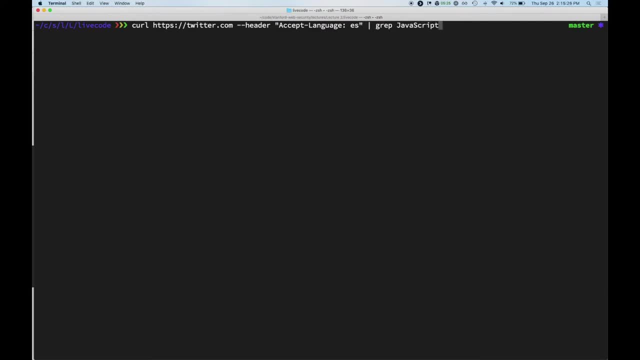 and just look for a particular phrase that i happen to know is in there called javascript, and i can also add silent here to get rid of the the output with the downloading. so now, if we do that, we just get this little part here that's telling you, uh, who knows spanish? does someone? 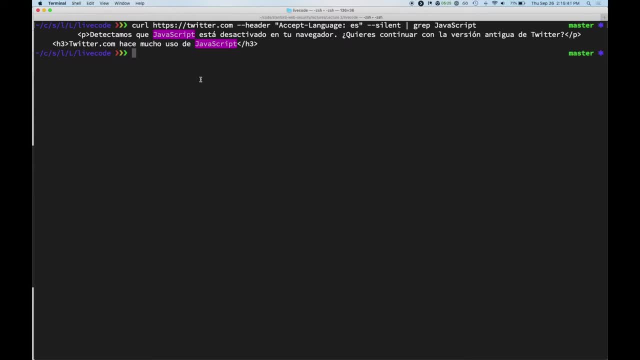 translate this for us. what does this say? say, uh, okay, so it's giving them a link to click to go to the old old twitter that doesn't need javascript, cool, so oops, oops. so now, if i, if i change this to like ar for arabic, we'll get some. 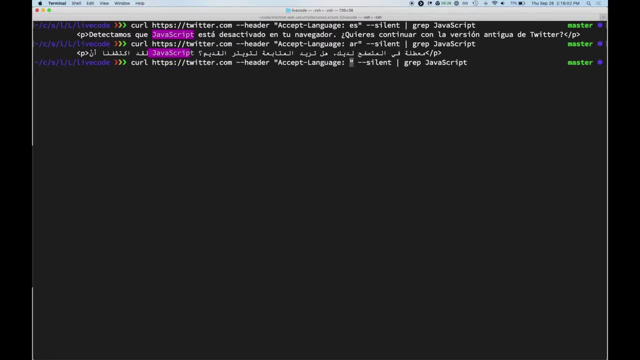 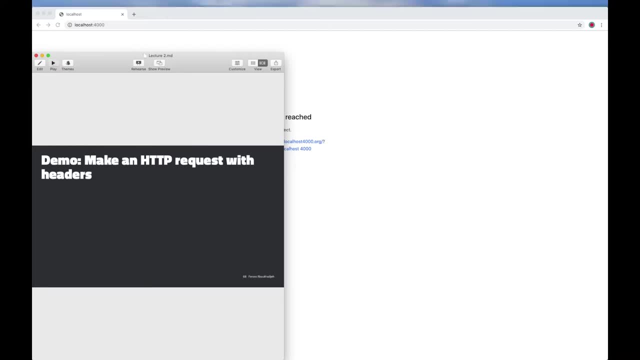 cool arabic script: uh, yeah, and you can just put anything there, but yeah, that's, that's kind of cool. so it's just that easy to attach headers. um cool, um cool. now let's uh talk about the response headers. um, so the server can tell you a bunch of useful. 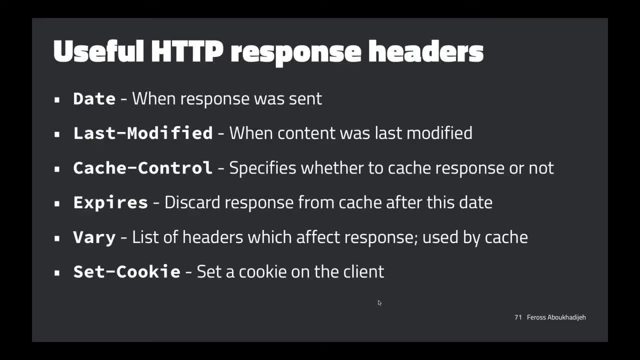 things in the response, um, one thing so. so here's a few we'll go over. so date is just when the response is coming back. um. last modified is like when the file was last changed. according to the server, you can use that um in your in your future requests to say: only give me if it's changed since. 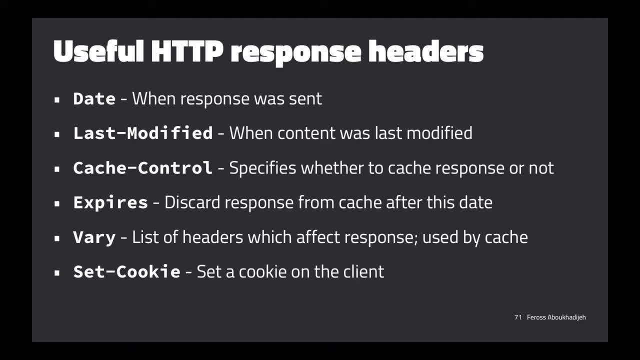 then um, and then again you can control caching behavior so you can say, like, please never cache this. that might be something you would want to say if it's some information that you don't want to say, you don't want to be saved onto the user's machine. um, and then expires is a way of saying. 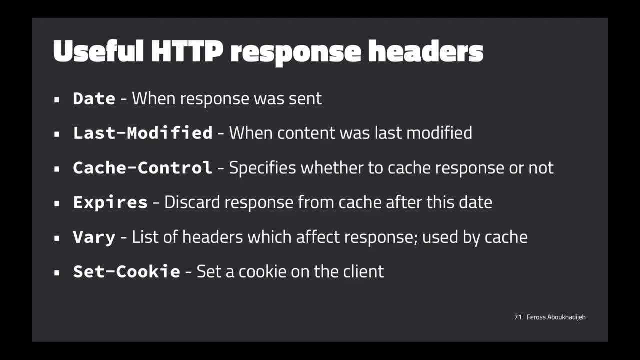 um, please delete it from your cache after this date, because i know that i'm gonna have a new version then, so just don't save it after that date. um, very is interesting. so, um, let's see so very. who's had even seen various before like or know what it is it's? it's really interesting. 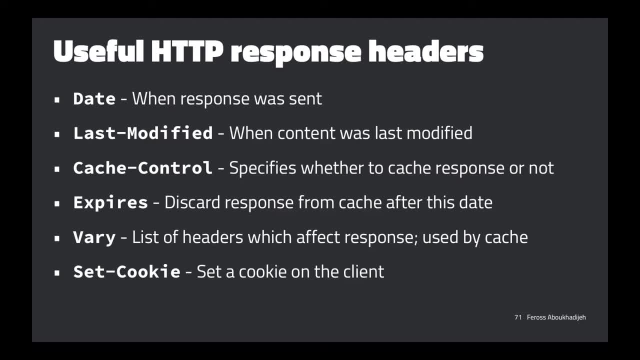 so it's, it's um, so can you think of any problems with caching stuff like say: okay, so say that, uh, say that i visit twitter, right, and i am, i set my language to spanish, um, and uh, and twitter sends down like a, a page, and they say like go ahead and cash this for a day, like we know it's not going to. 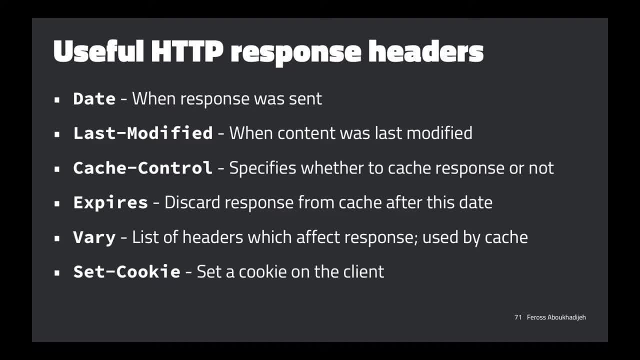 change, the site will be faster. so just cache it, keep it, keep it, keep cash per day, and then, um, i log out and somebody else uses my browser and logs in and they- they have arabic as their language, set um, and now they make a request for that page, right? the issue there is that now that request might 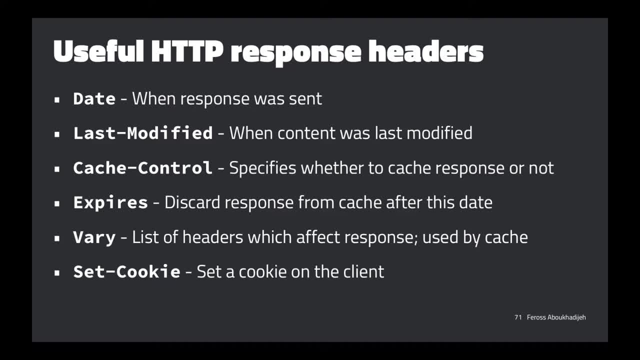 match that page. that's already set up for that page, so that's why it's not going to change the site. it's already in my cache that that is is in spanish right, and they're making the exact same request. they're requesting, say, the home page right, and so how does the browser know that it? 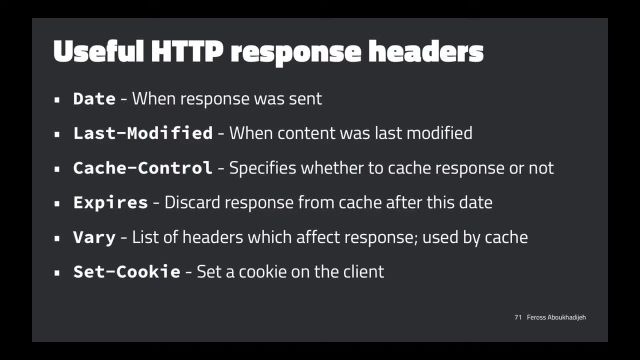 shouldn't reuse that cached version- that's in spanish for the arabic page request. right, so that's what the very header is for. so what would you do? well, how would you? how would you use the very header to to fix things? anyone think how you do that? 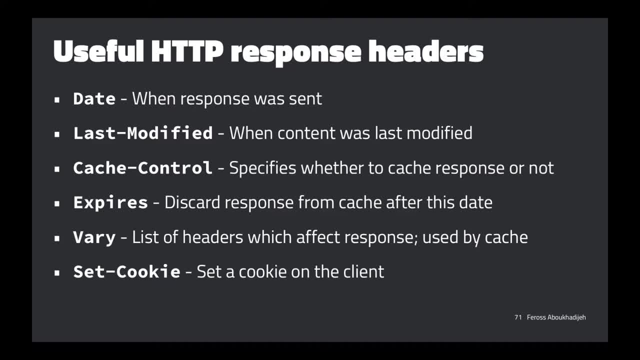 yeah, so you say here which headers are- um, how are? let's see how to word it. basically, yeah, which headers affect the response? that's what it says here. so you'd say like, basically, if so, when you save this, when you save this and cache it, remember to look at that list of headers that are in here. 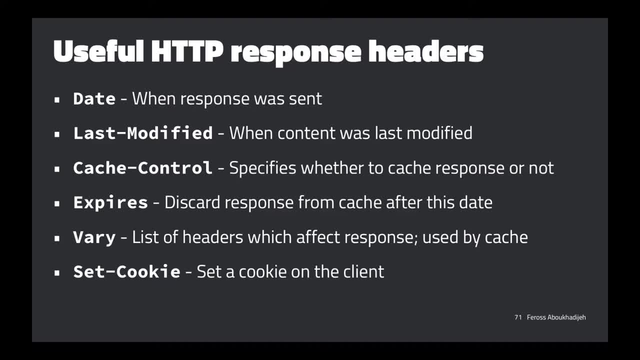 and save that along with it. and next time you make a request, compare and see if there, if the headers aren't exactly the same, then you need to not use the cache version, right, does that make sense? yeah, cool, cool. and then, um, then set cookie. that just lets you set a cookie, so you know. 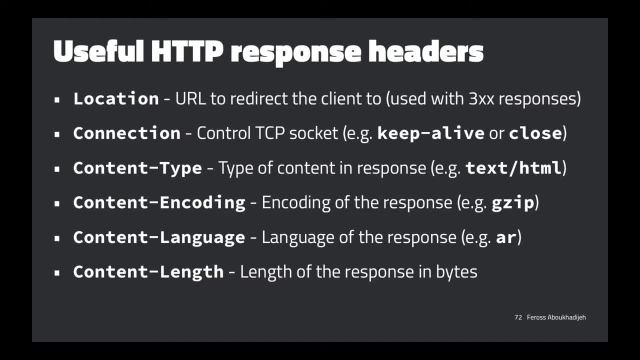 the value is the cookie that the browser saves, and we'll talk about more about that in a second. uh, and then we have location, so that's useful. if you're giving back a 300 response and you're going to tell the user to go somewhere, you do that by setting the location header. so when you 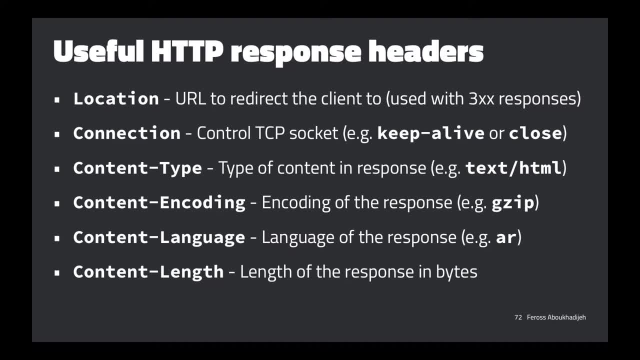 get back to 300, the client looks at the location and then it goes to that destination and then these are all, um, these are all just, uh, the sort of corresponding ones that match the things in their requests. so if you said i want html, the server can respond and say: confirm, here's html, right. or if you said: 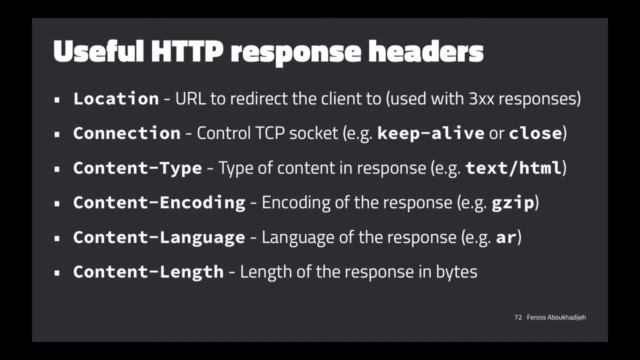 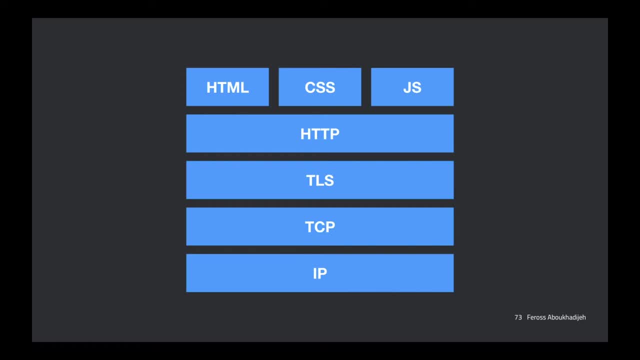 i want gzips response. it can confirm to you. okay, here you go. here's a gzip response, so you should make sure you know. use this to basically figure out what to do with the response. cool, and so diving in here. this is just sort of the protocol stack, um, so i'll just expand the names there. so 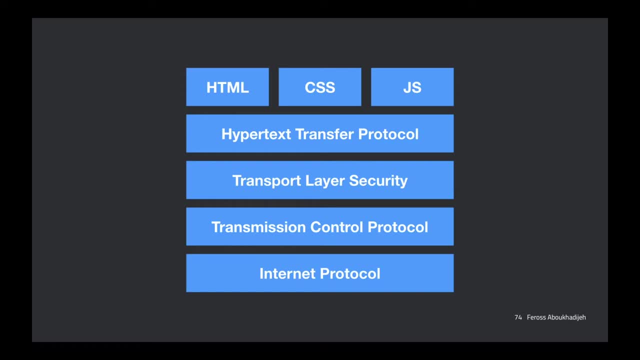 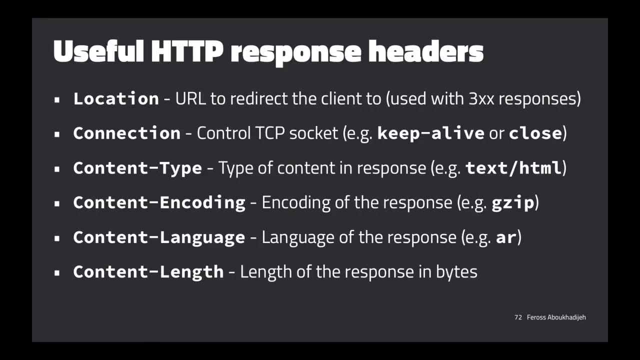 so, um, everything is on is built on top of ip. that's just the way we connect to computers to each other. oh yeah Yeah, so they're not required. I mean, you could write your own HTTP client. In fact, we might do that in a future assignment. 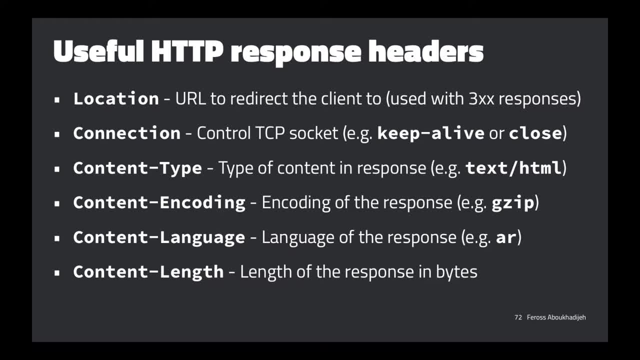 You can just do whatever you want. Yeah, you don't have to follow it. There's no enforcement of this. This is just sort of the yeah, the server's telling you. if you want correct behavior, basically you should do this. 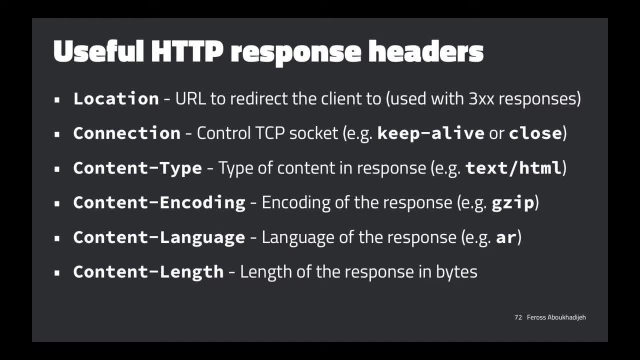 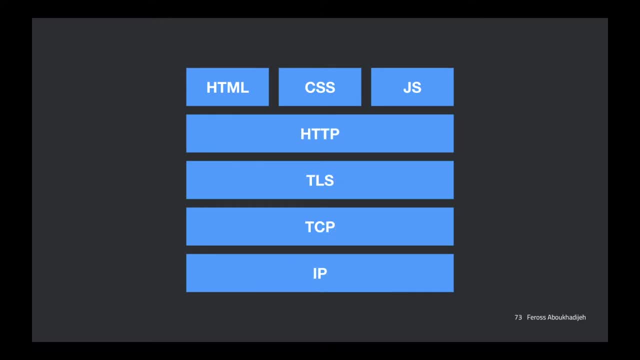 Yeah, yeah, cool Yeah. so anyway, the important point here in this diagram is just to know that HTTP is built on top of a stack of other protocols, So the first step is you have to know the IP you're trying to talk to. 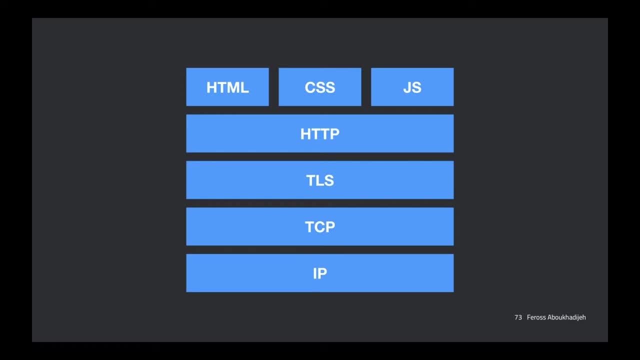 and that's what we use DNS for. Once we figure out the IP address, we open a connection, use TCP for actually ensuring reliable and ordered delivery of our messages. And then so this, this one here: TLS, this is encryption. 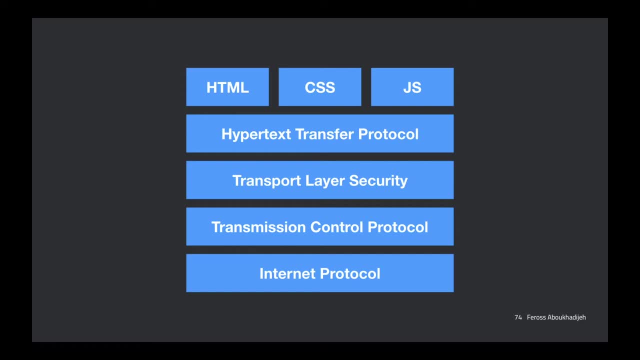 So we're going to talk about that later, But note this is optional right. You don't need to actually use TLS And then HTTP is what you actually send over this. this socket that you created with TCP And then HTTP is typically used to transfer website stuff. 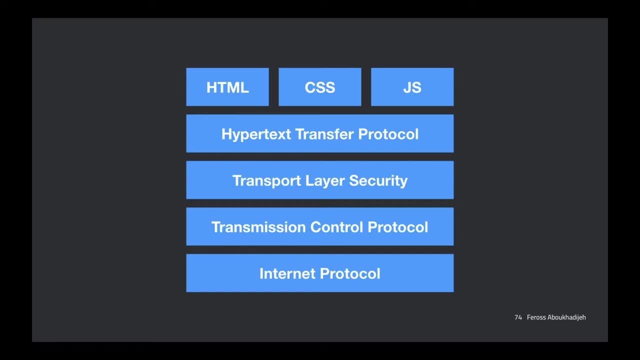 So that's HTML, CSS and JavaScript, Although you can transfer anything with it, but typically that's what we're sending to our browsers. Cool, so what I want to show you now is just really a little bit of a bit of a tip. 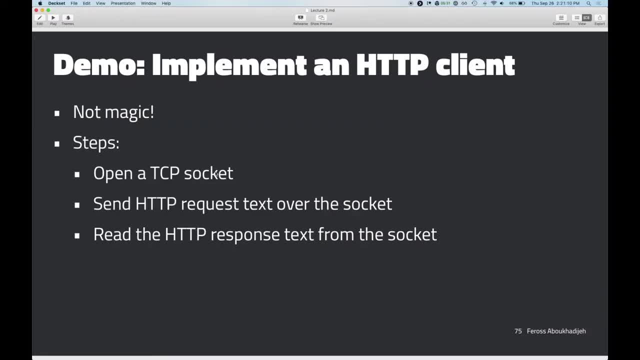 a fun demo. It's basically what we're going to do here. I have the stuff up here. Basically, we're just going to make an HTTP client from scratch. So it's not magic, It's really not that crazy of a thing to do. You just make a socket to a server. You know the server's. 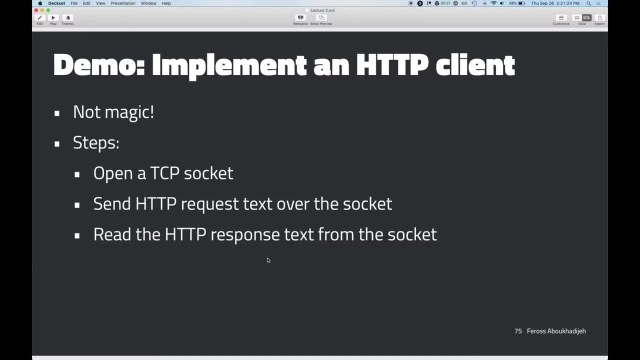 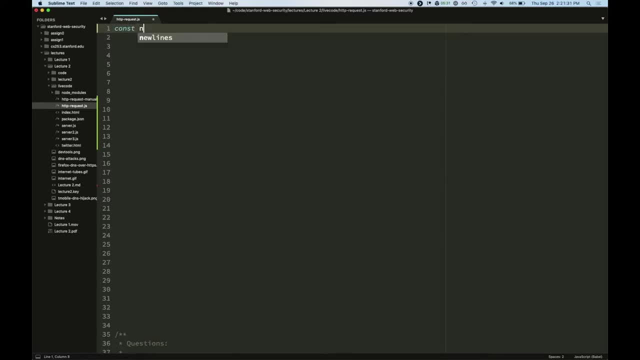 IP address right. You connect to it and then you just send this text over it and then you get back this response. And it's not magic, So it's kind of cool. So this is what we're going to do. This might be useful to you if you're not familiar with Node, But 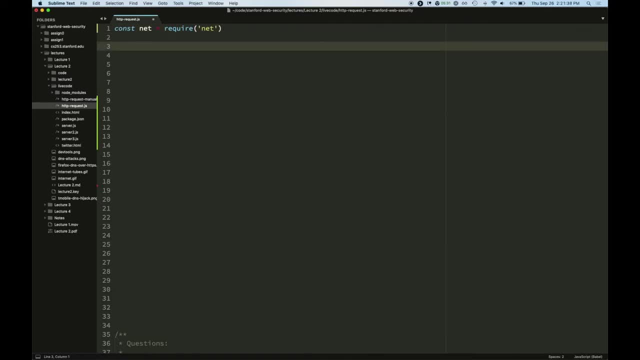 this is a package that we're going to just import And what it lets us do is create TCP sockets. So we use it by doing netcreateConnection And it's going to take in an object. Host is the IP address, Or, if we want to be lazy, we can just put in the domain name and it. 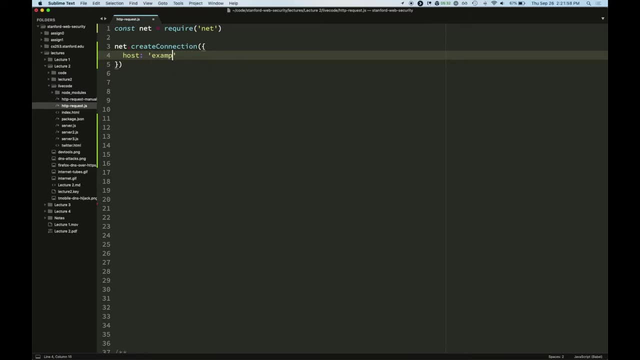 will do the DNS step for us. So I'll put in examplecom here And the port I'm going to put in is: does anyone know the port I'm supposed to put in here? 80.. Yeah, so 80 is just the port for HTTP. That's just what it is. Yeah, so we're going. 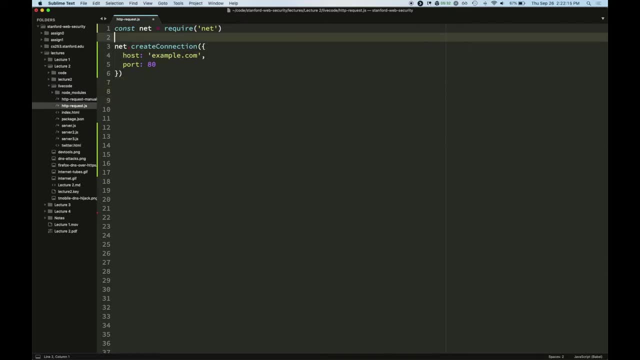 to connect to port 80 of examplecom. So then this thing gives me back a socket And I'm going to take the socket and I'm going to write something into it. So let's write in a request. So I'll define a request here And I'm going to use this weird string syntax. 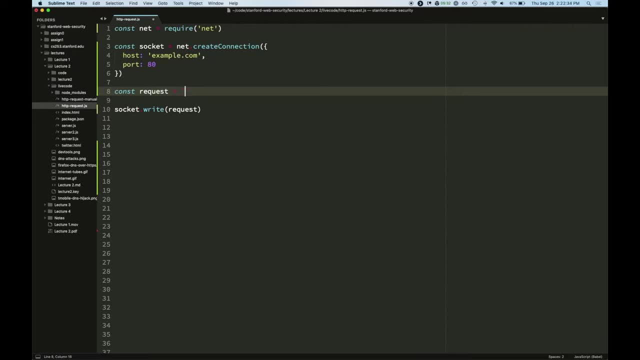 that you may not have seen before, but this is called a template string And we're not even going to use any of the templating features that it gives us. We're just going to use it because it lets us do multi-line strings, So I can use new lines. 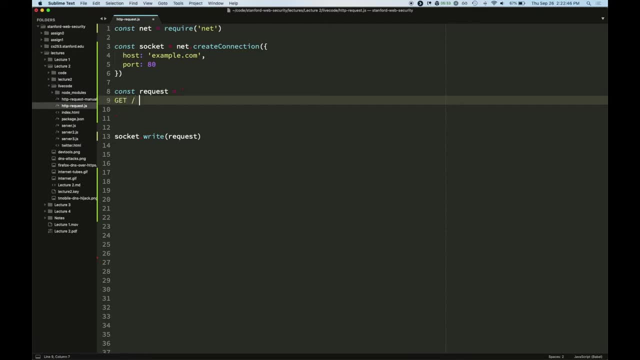 in my string. So I'm going to type here: get slash. that's the home page. I'm going to get the home page And I need to include a host header, Otherwise the server won't know what we're asking, And then I'm going to add an extra new line here. So I'm going to do. 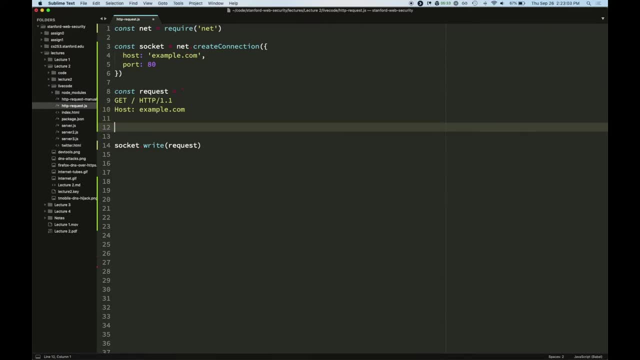 one, two new lines, Right Cool. There's something wrong with this, though. Does anyone see something wrong with the way I've defined this string? What A new line where At the beginning- yeah, There's a new line here. I hit enter here. So really I should do that, But I'm just going. 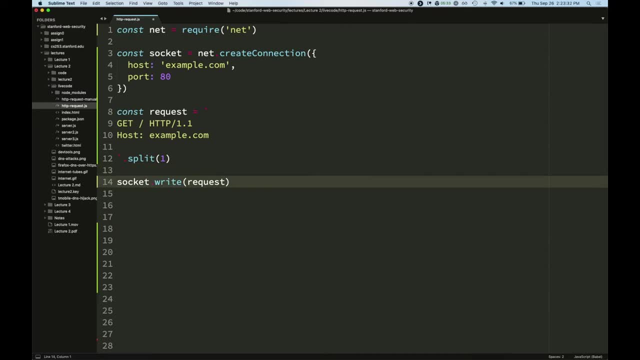 to be fancy and I'm going to just cut off the first new line. That way I can keep my requests like that. No, I can't tab here either, because those tabs are going to be included in there, So it's kind of weird. 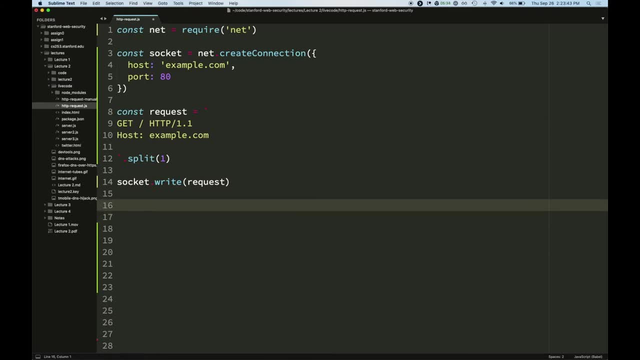 It looks weird, but there we go. That's a request. Okay, now how do I get the answer out? So the easiest way is so this object here, socket, is something called a node stream. So this is an object which will, over time, emit data that it's received from the server that it's talking to. 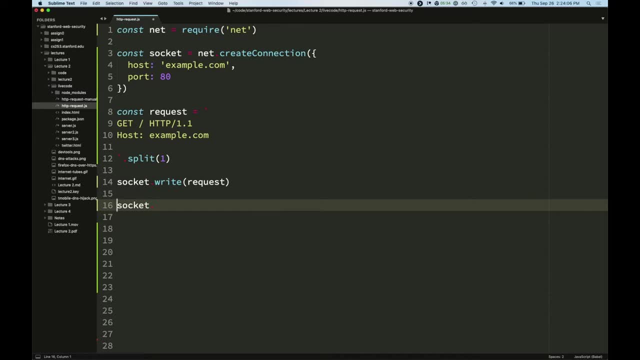 So do you want to see what's going on here? The right call. what we're doing here is we're sending data across the socket to the server And now to actually read the data out. what we could do is we could listen to. 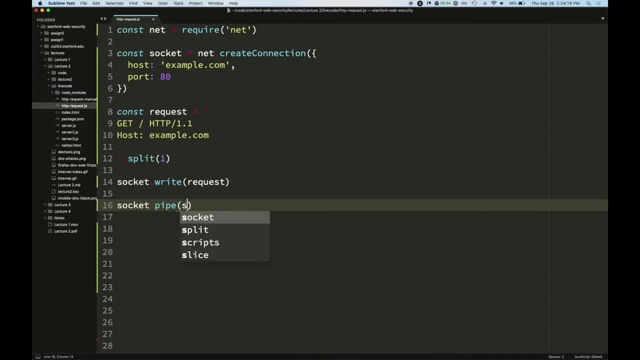 I'll just do it this way: We'll pipe And what we do is we have to tell it a destination where we want the response to go, And we can just do standard out. That's the easiest thing to do. So what we're saying is just print what you get from the server out, just like that. 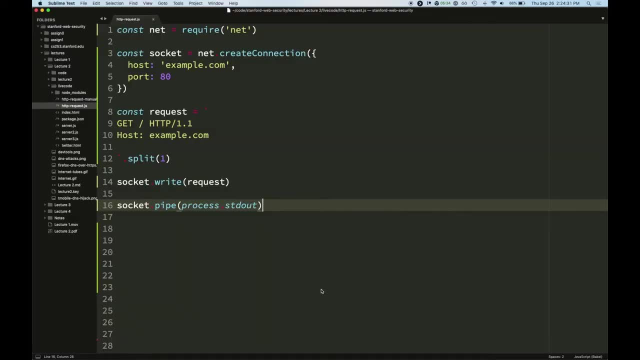 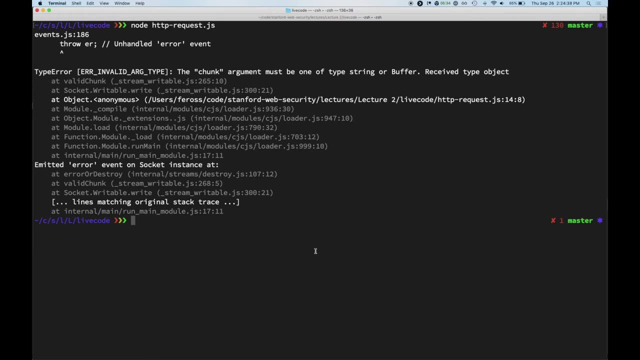 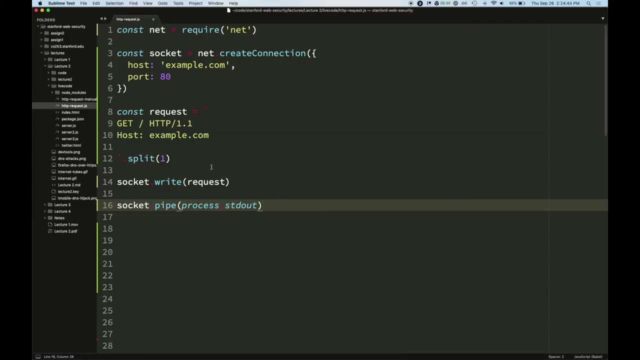 Cool. so now let's run this. What was it called? HTTP request, Cool? Oh no, The chunk argument must be one of type string or buffer Receive: type object. Does anyone see what I did wrong here? I wrote the string and then I piped it to standard out. 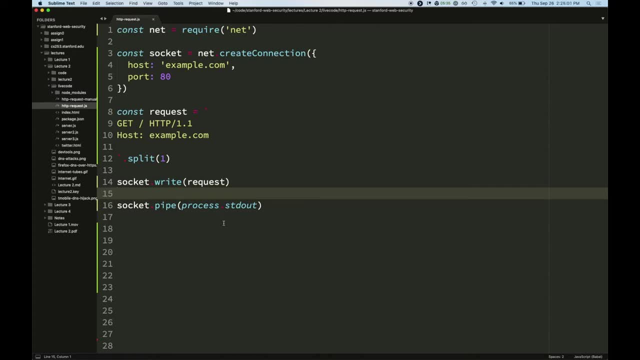 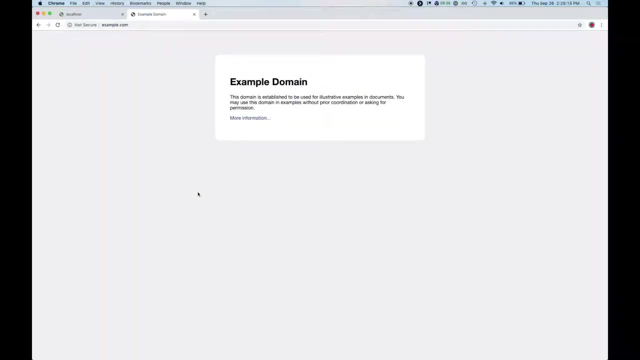 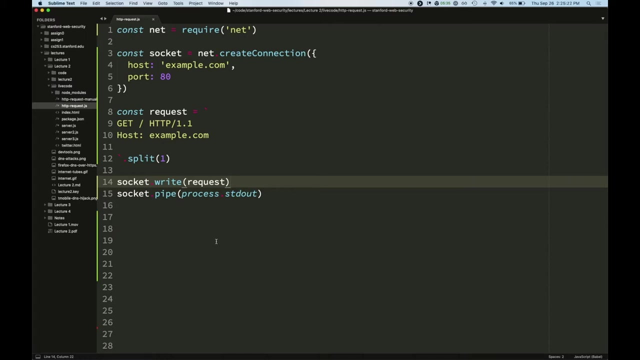 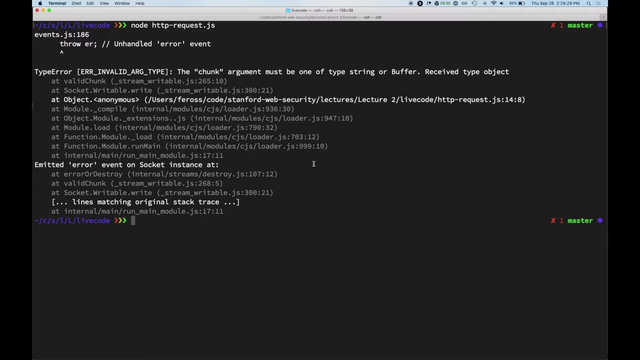 Hmm, Standard out write request. Does that look? do I not have internet? Could that be it? Nope, I have internet. Hmm, Oh yeah, let's look at the error. yeah, Unhandle error. The chunk argument must be one of type string or buffer. 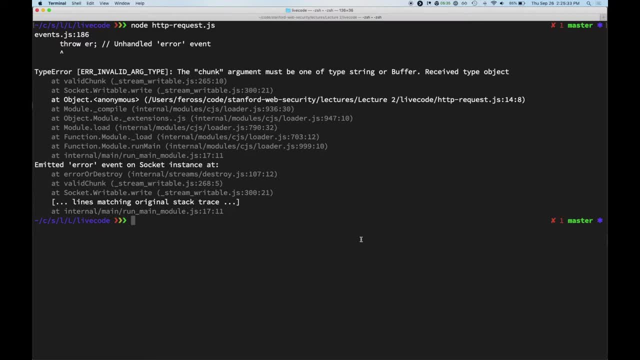 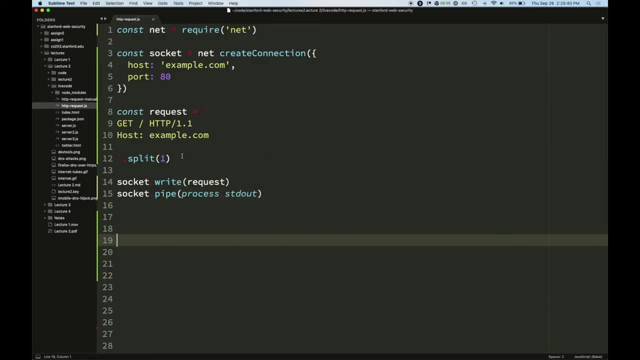 Receive type object. Uh, that is, that is some kind of a stream error. Uh, why would I What? what does? Oh, sorry, I meant slice. Sorry, I used the wrong function. Thank you, Yeah, I wanted to slice off the. yeah, sorry. 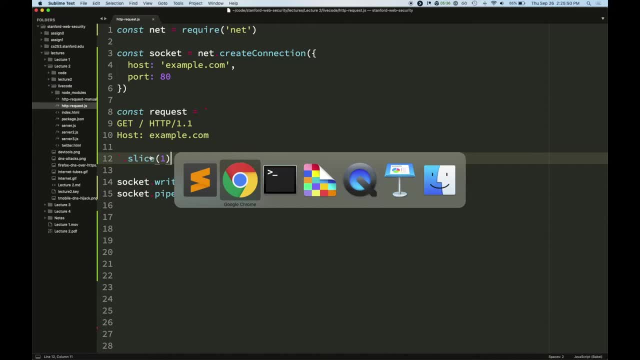 Good catch. Who, who? who caught that? I appreciate it. Yeah, thank you. Yeah, cool. So now let's try it. Uh, no, not that command, This command, Okay, cool. So what did we get back? 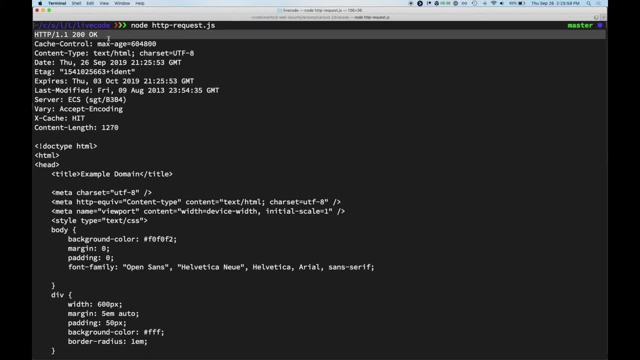 We got back notice. we got back the first line which tells us that our response, uh, that was 200, it was successful. Got a bunch of headers, Uh, and then we got, uh, a, a, a new line and a new line. 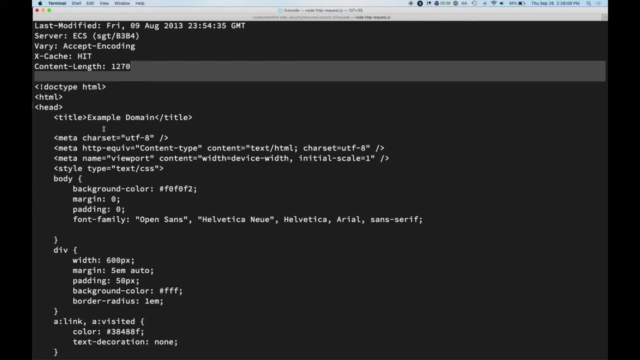 And that delimits the, uh, the headers and the and the body. And then this is our body right here. This is our response. It's HTML Cool. Does anyone know why? does anyone know why it's hanging though? 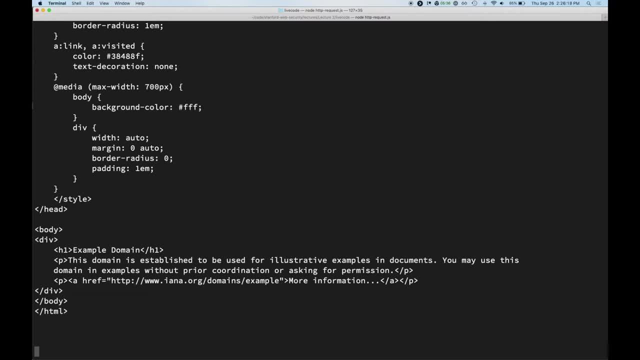 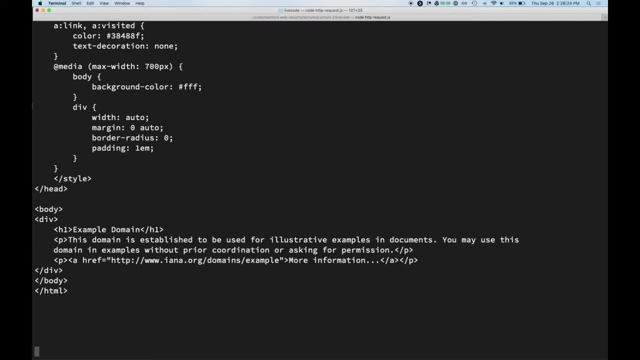 Like: why hasn't it? most scripts will end when you when there, when there's nothing left to do, right, Why is it? why is it hung? Socket's still open. Yeah, I didn't close it. Yeah, Um, so I could close it if I wanted to, but um, or the server could have told me. 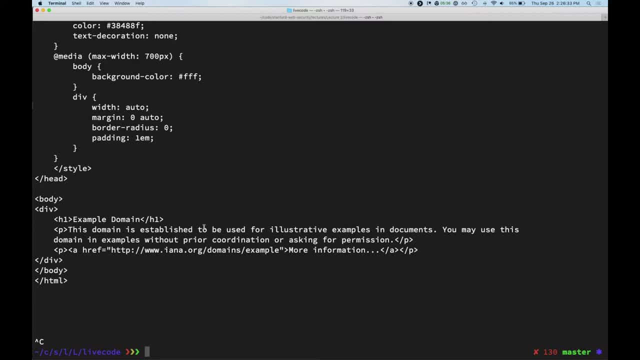 to close it if it would added that that, Okay, Okay, Uh, connection closed then then um, actually I don't know if node will will read that and close it for you or if you have to do it, but anyway, yeah. 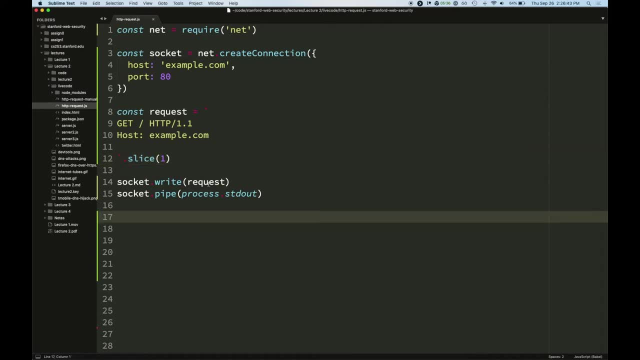 it's not. it's not getting closed. So that's, that's the issue. Um, cool. So one thing I want to point out is like, if I remove this host header, what, what, what's going to happen? 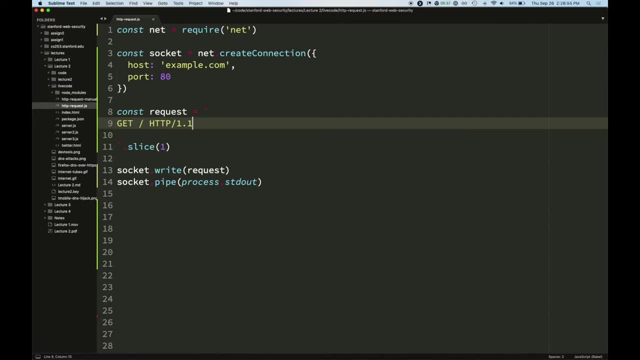 You'd think the server would know what to do, right, Like I connected- I literally connected to the server with the socket. I sent it this request saying: give me the homepage, right. Why wouldn't it just give me the homepage, for examplecom? 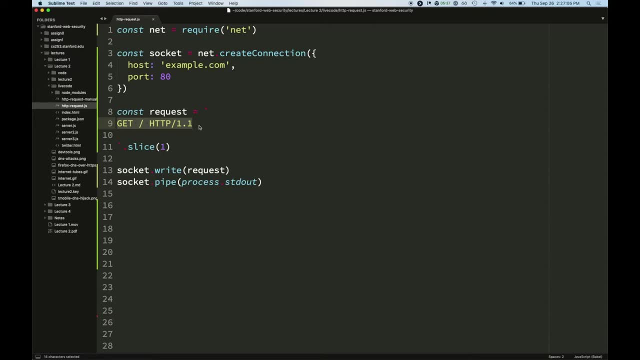 Like it's the. it's the examplecom server, right? Shouldn't it? shouldn't it know? Yeah, that's right, So that. so, just to repeat: um, it's possible that one IP address is hosting many domains, right? 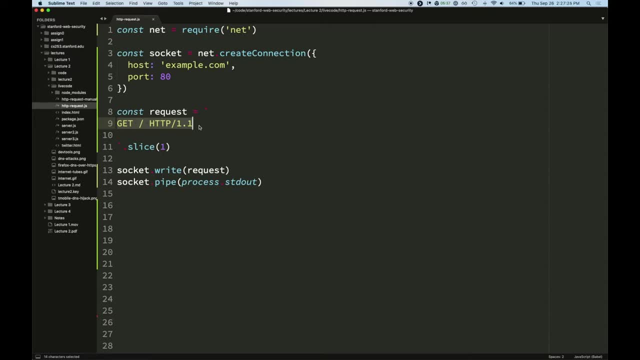 Um, in fact that's very common right. You might have a server that can serve your, your, your blog, and then this other side project thing you're doing, and whatever. You might have four or five sites all in one server. 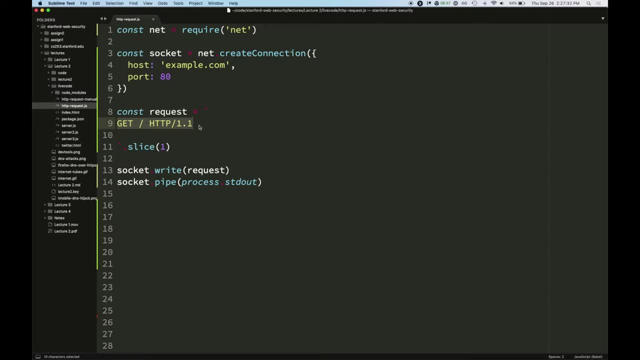 They all have the same IP address. So if you don't tell the server what uh host you're interested in, um, typically it'll just error Um. it might also just pick one and send you back a random one. 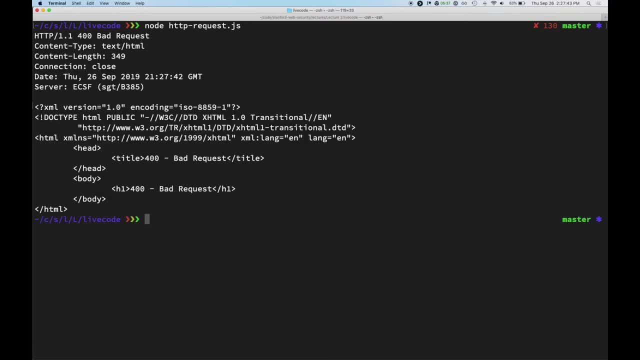 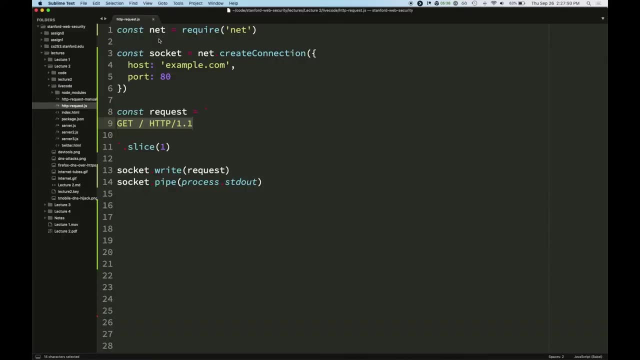 Um, but uh, look, I think in this case what's going to happen is it will just tell us it's unhappy with us. See, it'll give us a 400 bad request, and 400 means it was our fault. So yeah, we'll add that in there. 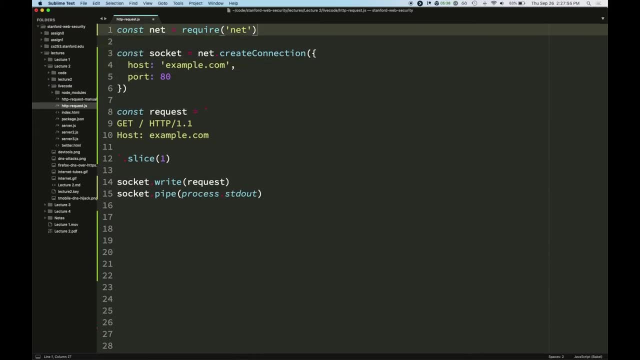 Cool, So um and then. so just one thing I want to point out too is if we want to not rely on um, on this module, to do the DNS lookup for us, I think it becomes even clearer why we need hosts. 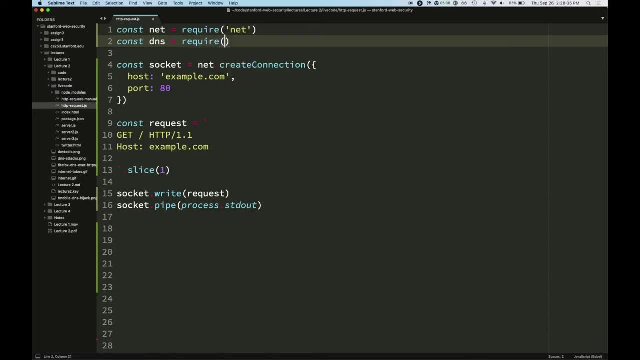 So if I were to do DNS, you know require the DNS package. here we can do dnslookup on examplecom and that will give us um. has everyone seen this syntax before? Um? this is basically me defining a function and these are arguments and this is the body of the function. 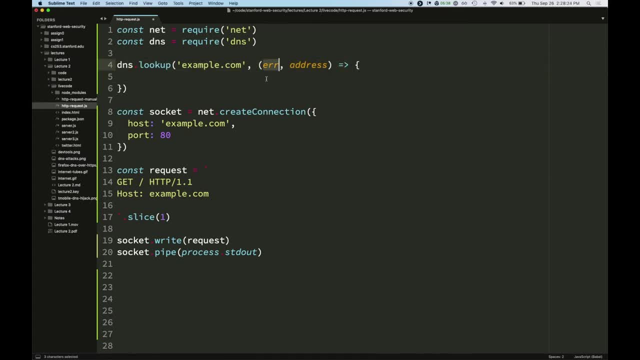 So I'm saying is a lookup examplecom. uh, tell me if there was an error, and so I'll do. if there was an error, I'm just gonna crash the whole process. Um, honestly, it's better than ignoring it, Like at least you know there was an error, uh, uh, and then what do I want to do here? 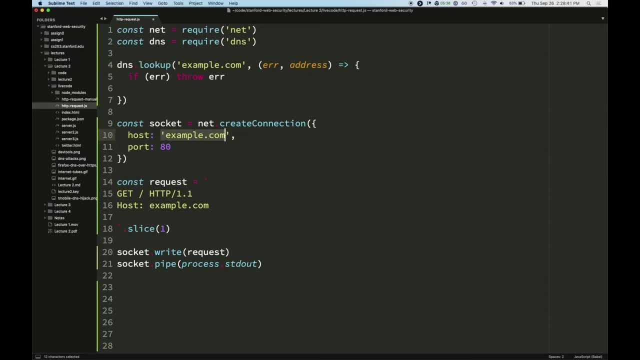 Um, so I want to take. this is the IP address, So what I want to do is actually use that in here. Um, I need to actually copy all this code and paste it in here. Uh, there we go. So, oops, wow. 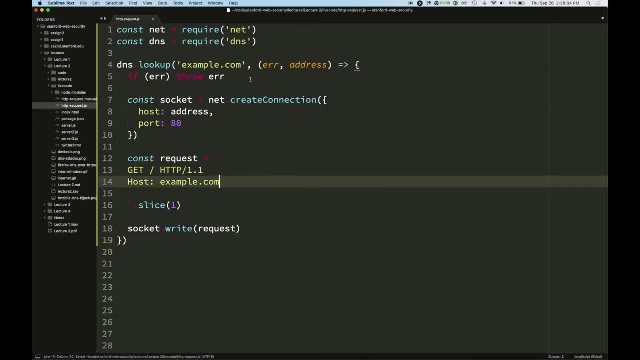 I have some really weird shortcuts, Okay, So, uh, yeah, so what we're going to do is look up this examplecom. We're going to get back an IP address and then we're going to connect to that IP address. This is an IP address. 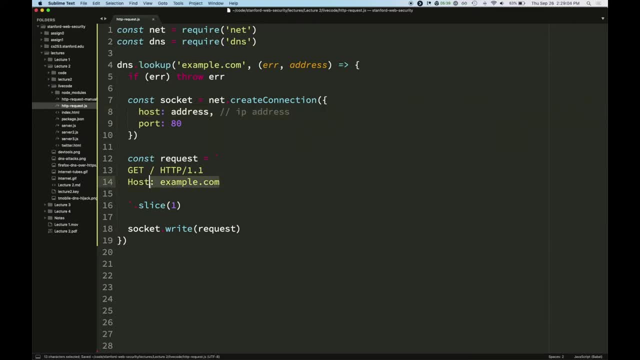 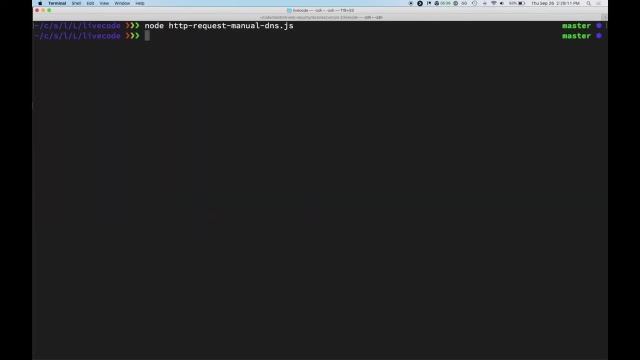 And then, um, now, hopefully it's a little clear why we also have to tell it like what, what domain we're interested in here. So let's see if this could actually works. Uh no, Oh, I put it in a different file. 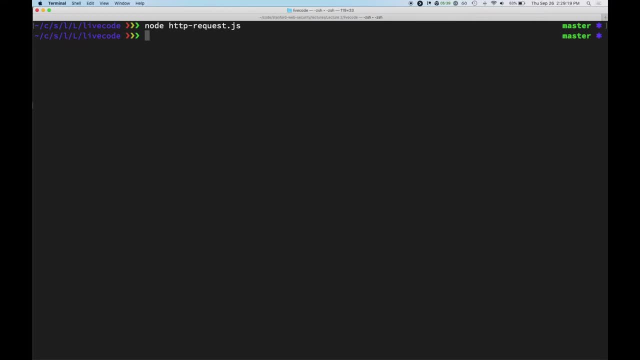 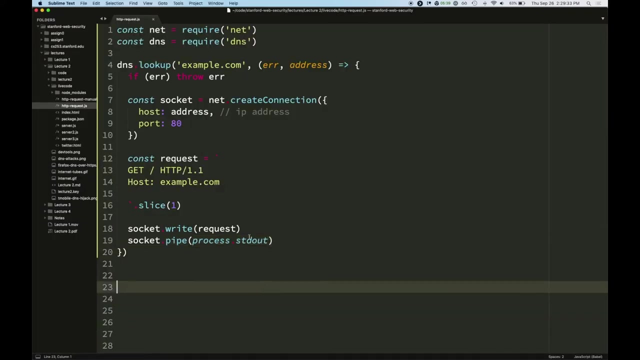 Right, Sorry, I've been just doing it in the same file, That's fine. Yeah, we'll do that. The socket pipe. Oh, thank you Cool. Uh, that's interesting. Oh yeah, now there's spaces here. 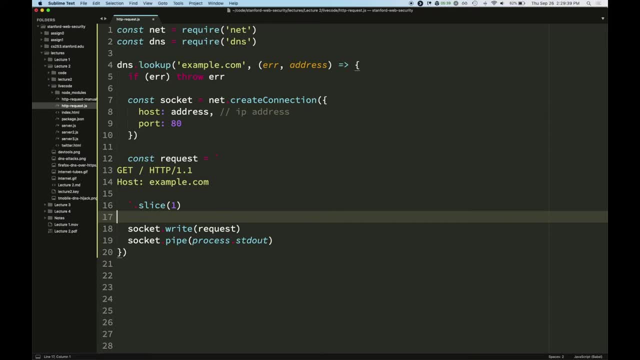 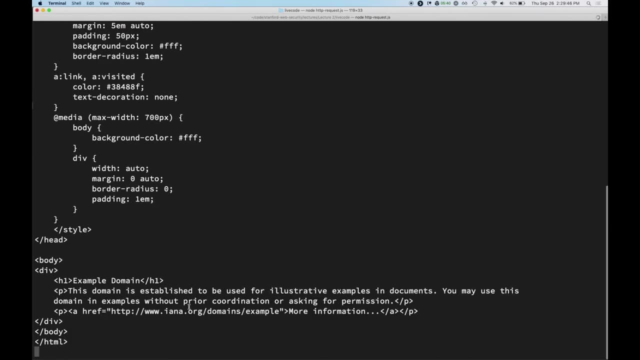 Yeah, I just mentioned that you can't have spaces there. Uh, yeah, so that's the problem. Uh, that's nice, That's a nice problem to have. Okay, There we go. Cool, Got my response again, So that's cool. 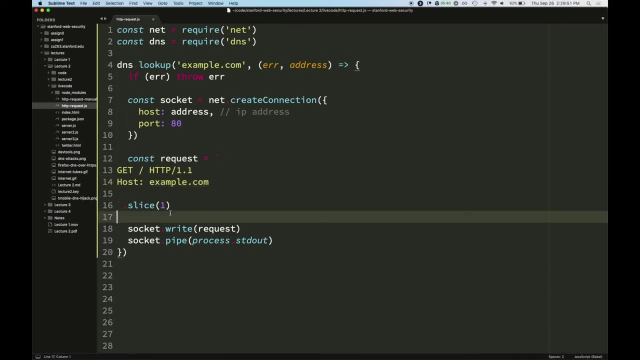 Yeah, So you connect with an IP and then you you tell it the domain you're interested in. Any questions about this? Cool, Yeah, So HTTP is not magical. It's pretty. it's pretty cool And and and it's really nice how you can just- uh, you can just play with this stuff. 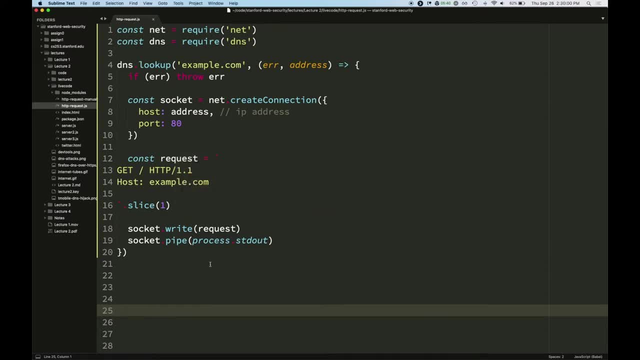 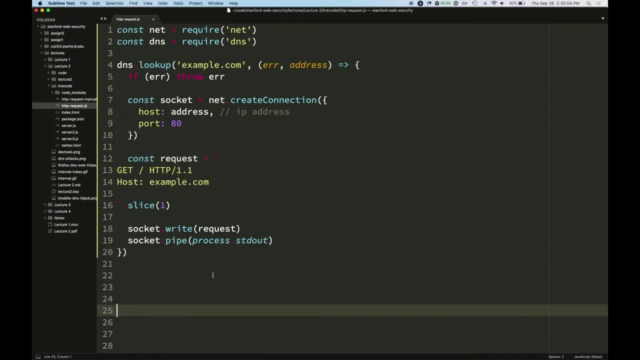 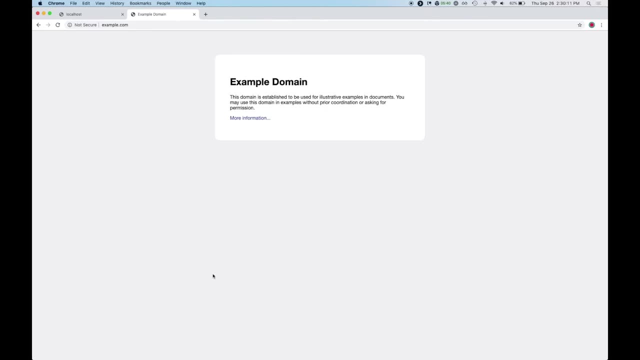 You can just jump in there and do this stuff. Um, any questions? All right, Go on, Okay, So. so one other thing I want to show you is the developer tools. This is obviously a really handy thing to know about. 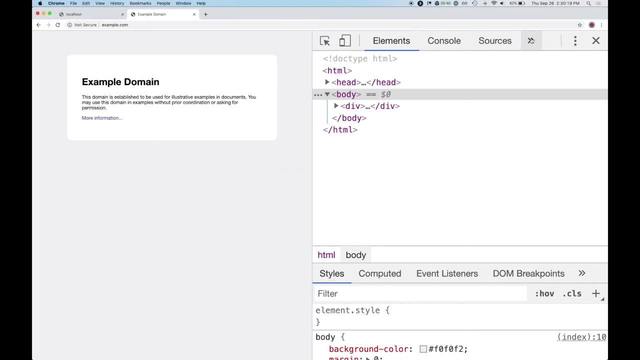 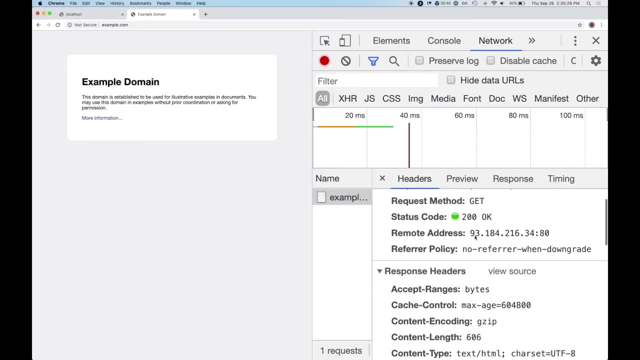 So you can, on any page, you can right click, inspect and pull this up and, um, you can go to this network tab and we can just see the same exact thing we just saw. So if I refresh this, we'll see that, uh, we got these header, we sent these headers. 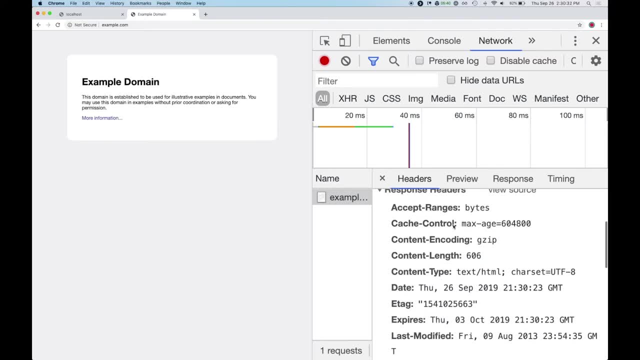 and we got back. you know these, you know these, you know the, the, the, these, you, these other headers here in response. So this is just something to know that you can do this. It's really useful, for it's gonna be useful. 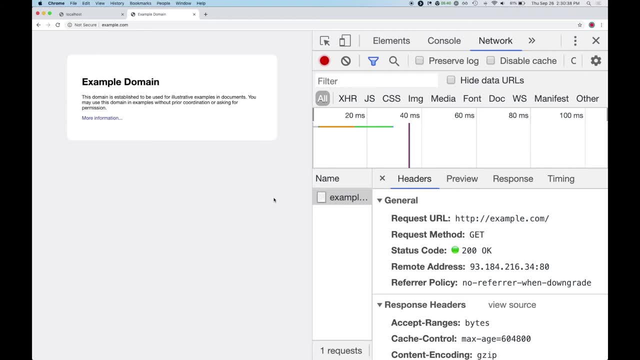 on the next assignment, You can just jump in and look exactly what request the browser is making. So one thing I wanna do here is I wanna go to like a slightly more complicated website than examplecom- If I go to Twitter here really quick. 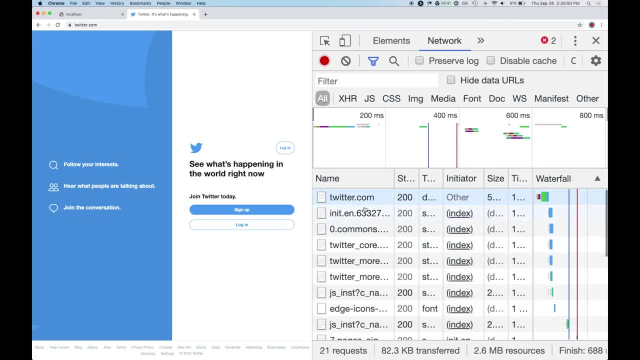 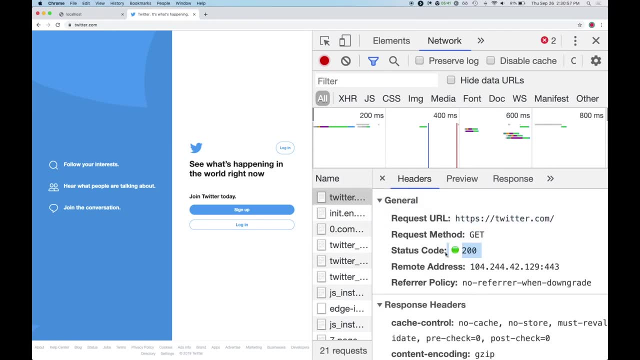 not logged in, am I Okay? good, So if I go to Twitter, you'll notice that this first request here was made to twittercom got back at 200, and then a bunch of these other requests were made afterwards. right, 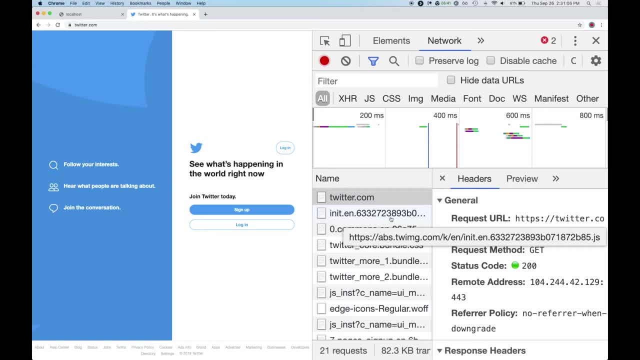 Why did that happen? Mm-hmm, Could it be like this code in the Twitter page, like asking for more resources from other places, like ads and stuff? Yeah, exactly, So the browser doesn't just make the one request you ask for. 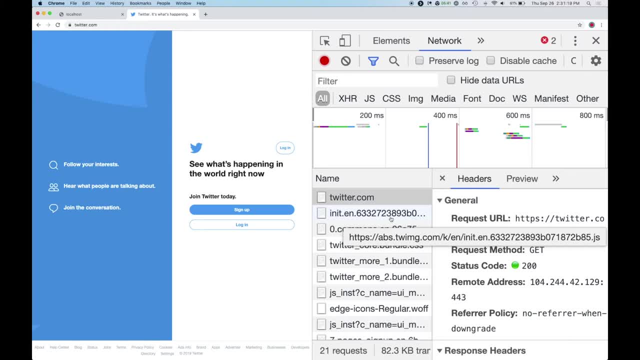 It gets back the HTML and then that contains within it more requests for sub-resources, right, And so that's gonna happen and there's this sort of a bunch of round trips that could happen, right. So it's really important actually for site performance. 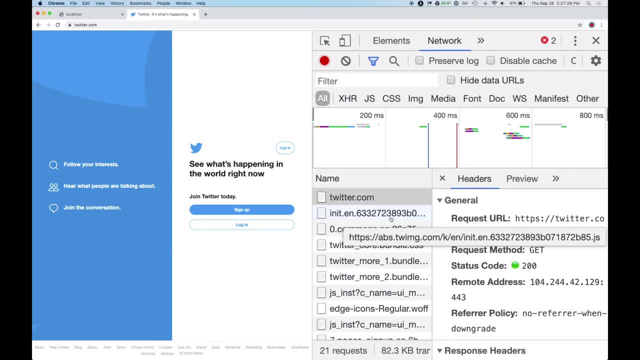 that you sort of minimize the number of round trips, but there's gonna be at least like two, because you're gonna request the HTML and then you're gonna get a whole bunch of stuff like images and CSS files and JavaScript files that you're gonna have to follow up with. 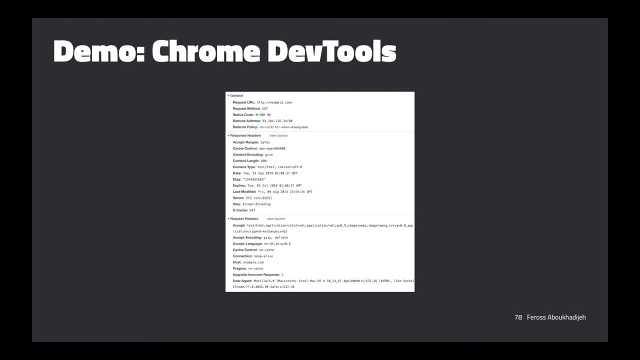 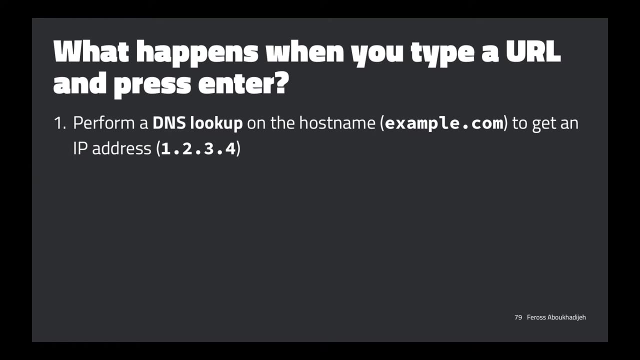 So yeah, just know that. Yeah, so yeah, we can review. now, What do we know about what happens when you type a URL and then press enter? So the first step is the DNS lookup. We're condensing it down into one line here. 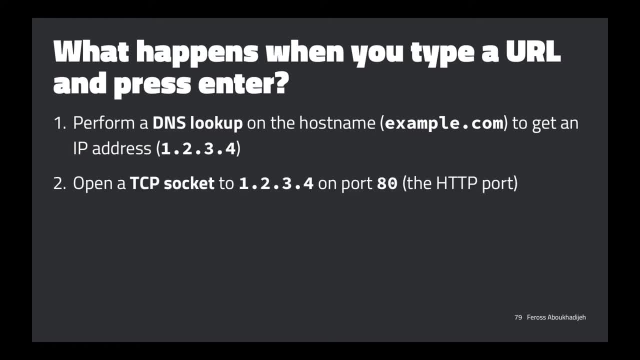 because we know there's the whole recursive part that it has to do. You open a socket to an IP on port 80. You send your request and you get back your response and then you display the response. Except, we just said we don't do that right. 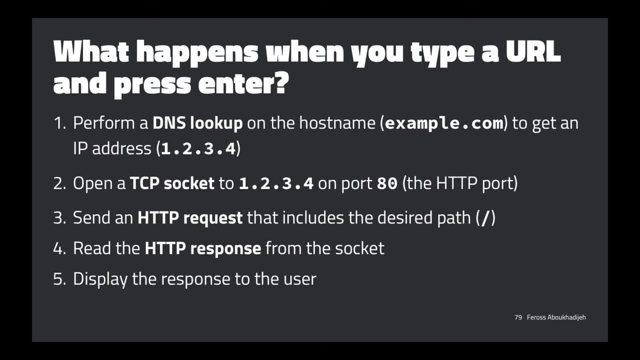 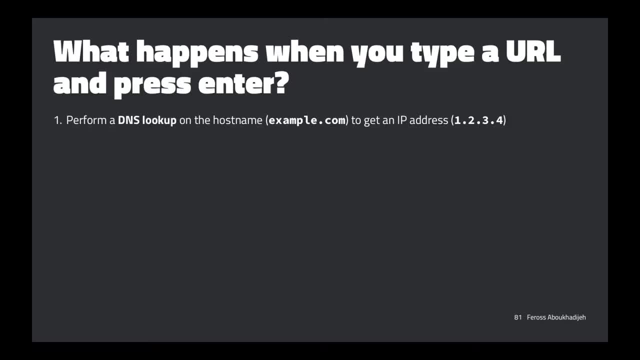 Because the response is gonna be just one HTML page and we know there's all these other resources, So we actually have to do follow up requests, So that's what. so this is what the full picture looks like. We read the response. We parse the HTML to figure out what it contains. 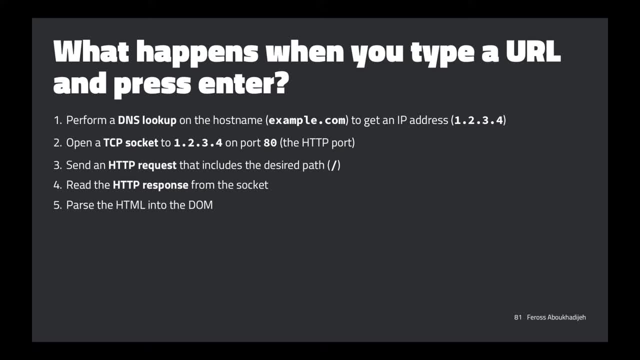 and we construct the DOM, which is the document object model, which is all the nodes that make up the page, And then we render the page based on this initial DOM. It might be missing some information, It might be missing some images, So there might be placeholders and things like that. 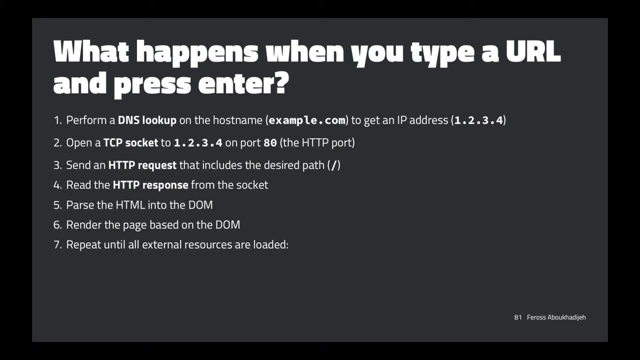 But then we look at all the missing resources and we fire out a bunch of requests for those And then we just keep repeating that We wait for the because the responses from those might generate more requests and we just need to keep waiting until they're all done. 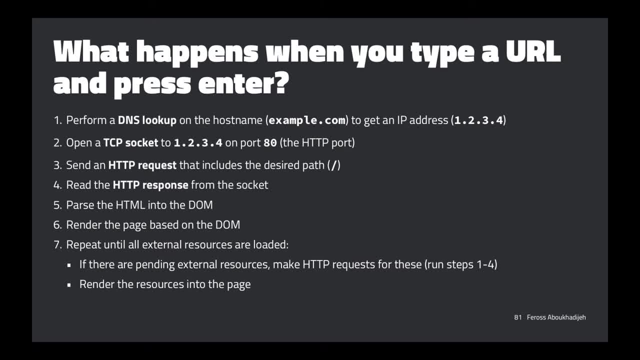 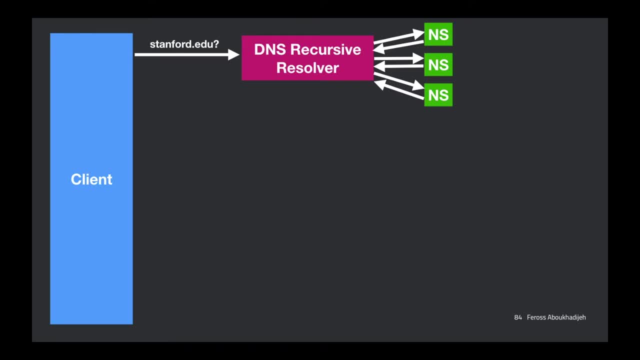 And then, as they come back, we continue to render them into the page. That's the full process, And so there's like a full picture here of how that all works. So there's your DNS Recursive step. you get back your IP of your server. 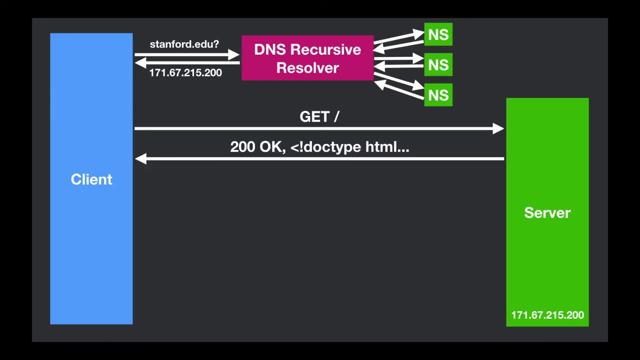 You now know which server to contact, So you send your get request to the server and you get back your HTML for the first page. And then now you've discovered a whole bunch of additional resources that you need in order to render the page, So you fire off requests for those. 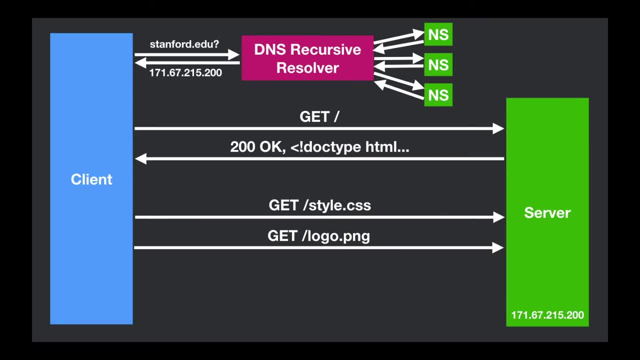 In this case, let's just say there's a CSS file and a logo And then you get back responses for those at some point in the future. And hot pink is a real color in CSS- It actually is. There's a whole bunch of 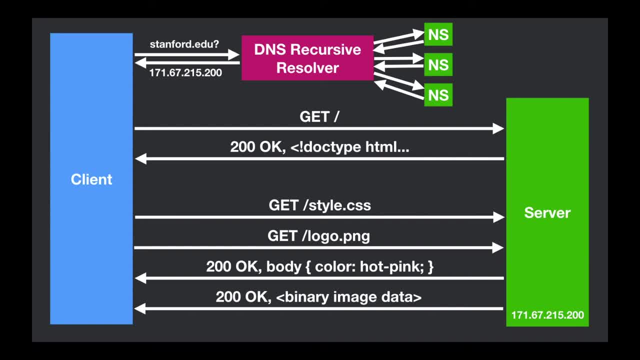 like names of CSS colors which are just like really wild. Yeah, just like completely random names. It's pretty fun to look through the list. Okay, cool. So we have like 15 minutes left Before we go on to cookies. is there any questions? 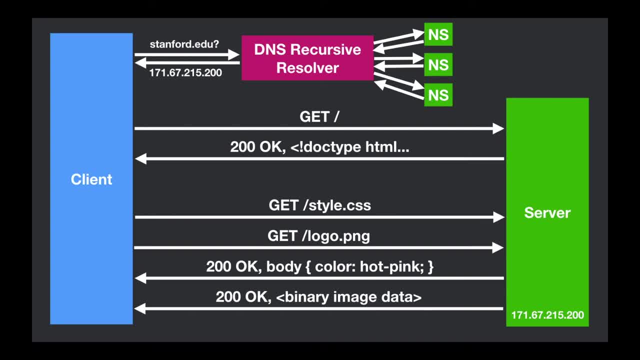 about anything HTTP related or DNS related. Okay, so we're not gonna have time to get too much into cookies, but I'm gonna give you a little preview and we're gonna get into the rest of it next time. But so cookies, the cookies are really cool. 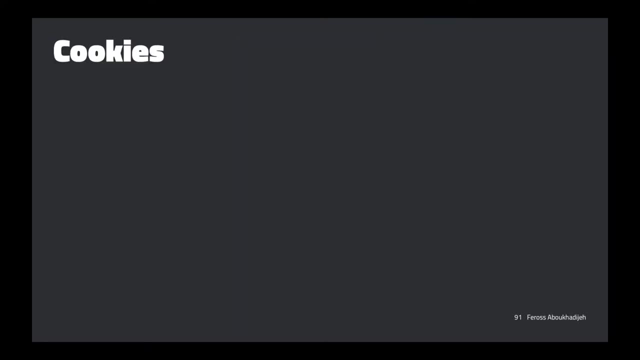 So they let you do like I mentioned before. they let you do authentication and like login and stuff like that, And there's all kinds of ways to attack cookies that are really fun and exciting. So this is how the server sets a cookie. 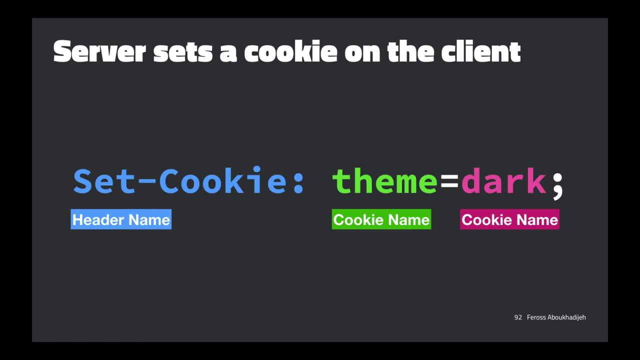 It includes the setCookie header, and then there's this key value thing with an equals between it, You can set whatever cookies you want, that you want the browser to basically remember and tell you going forward, So you can use it for things like preferences that the user has. 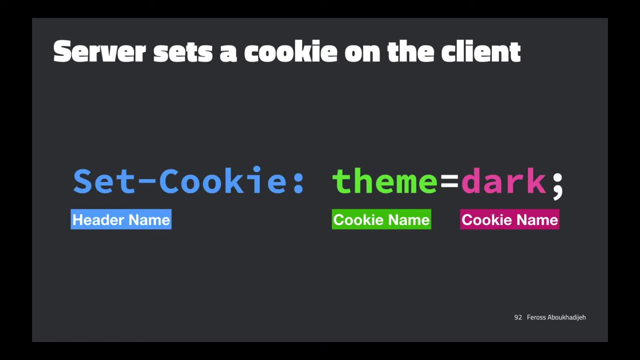 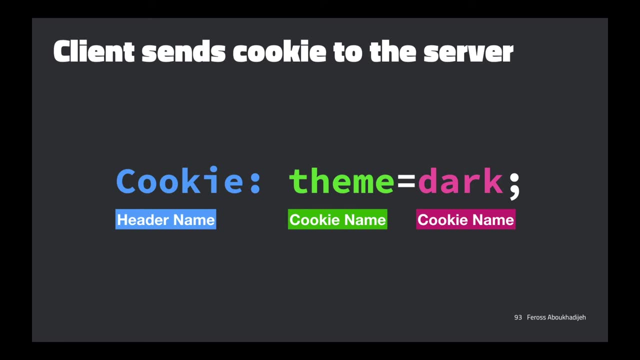 Maybe you wanna remember that the user asked you to give them a dark theme on the website or whatever, And this will just get sent by the client. Now every single request to the same server is gonna get. this is gonna get tacked on to that request. 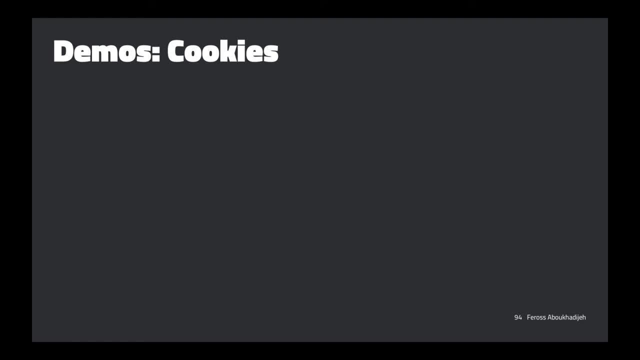 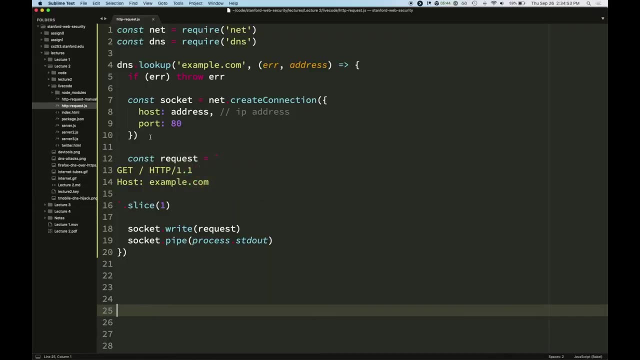 So let's actually let's actually look at this. So we're gonna actually implement a server and see how this works. So the first thing I wanna actually do is I'm gonna make an HTML file for a web page that we're gonna serve to our user. 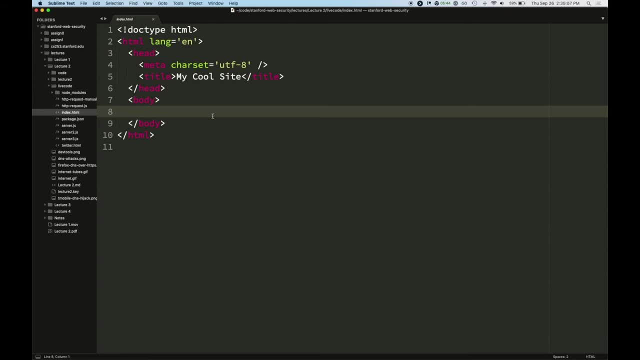 What we're gonna do here is we're gonna implement basically a login system using cookies. You can see how to do that. Hopefully we have time to do it. I can code fast. I think we can do it. Okay, so this page is gonna just be. 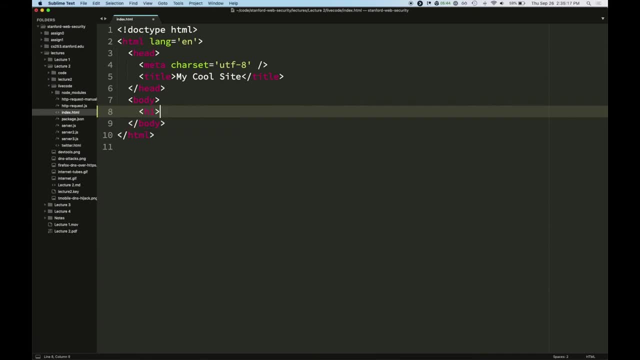 it's gonna be pretty simple. It's just gonna say, oh yeah, and we need to have a thing that we're building. So what kind of a site is this? Let's make it a bank. Okay, this is a bank login. 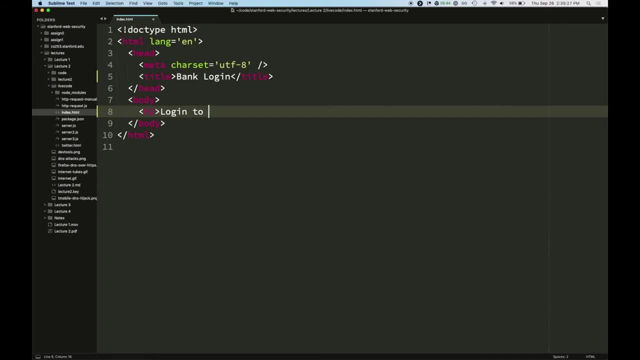 So I better do good here. Okay, So we're gonna say: login to your bank account, All right, And so we're gonna make a form. The form is going to post its response to a URL when the user submits it. And let's make. 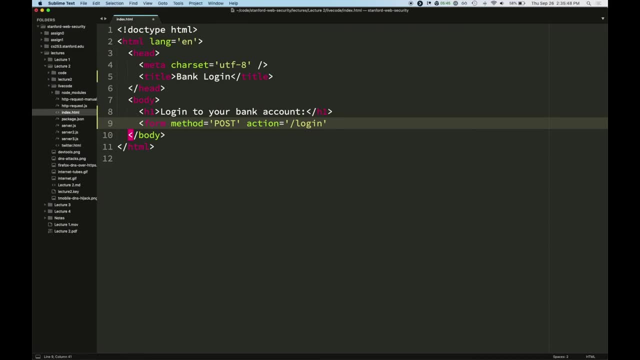 we'll say we're gonna make a login endpoint, So this is just gonna be a URL that we'll log the user in. Cool, so now in the form let's put an input for the username, Just like that, And we'll put another input in for password. 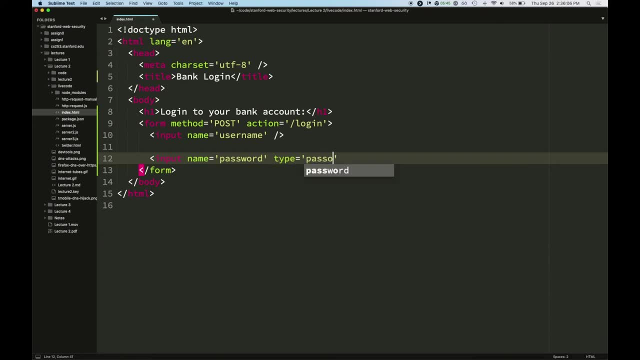 Now, one thing that we can do with the password is we can make the type of the form actually password, so that the letters they type show up as circles. Unless you guys don't wanna do that, You wanna see my password, but we can do that. 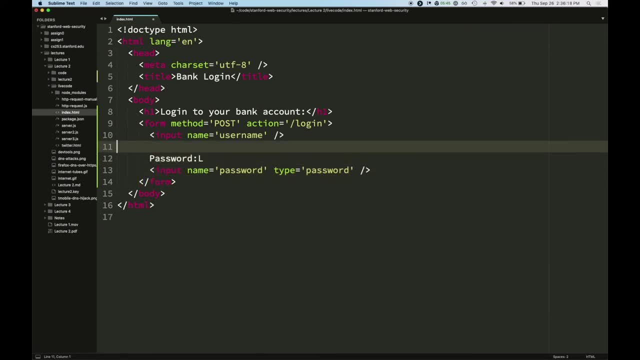 Okay, Okay, so let's label these. This is not the nicest way to label these. There's a nicer way, but we'll just. we need to go fast. So you know, ship it, Do it longer, Do it live. 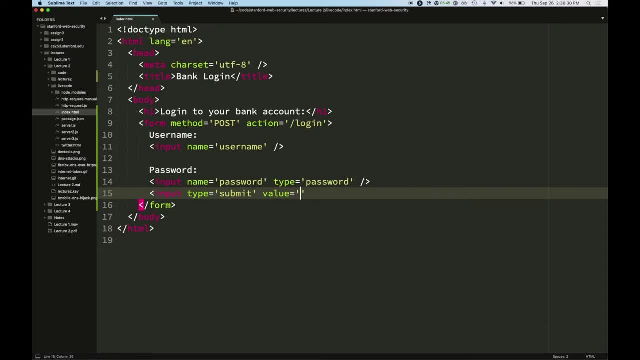 A lean startup. you know This is a lean bank, All right, so we have a submit button here for that actually logs the user in, and we named it login, Okay. so let's see what this looks like. I'm just gonna, I'm just gonna- open the index file really quickly. 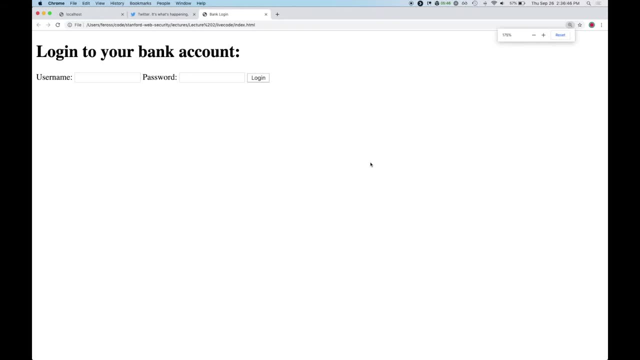 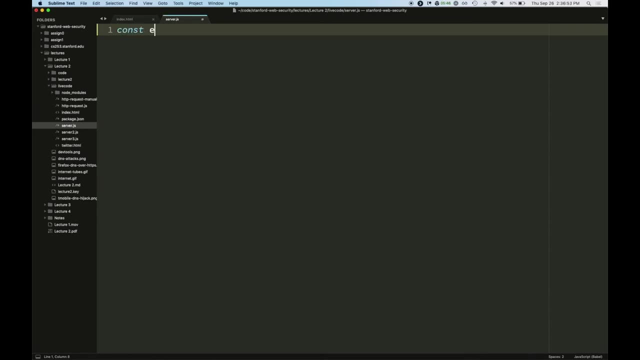 just to see what we, what we've built Beautiful, Ship it. It's good enough to ship right. I love it. Okay, all right, So now. now let's actually make the server component. So to do that, I'm gonna use- see, we could use- the HTTP module. 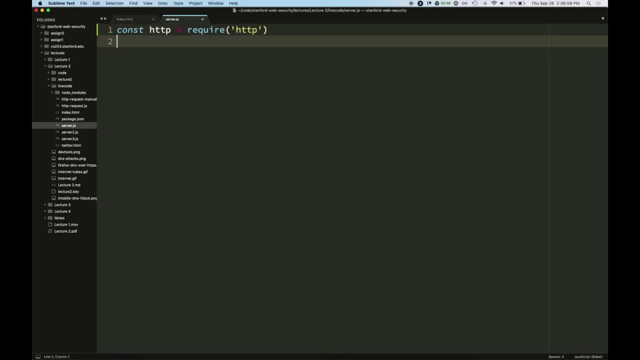 which is built into Node. It's just a little bit low level, You know. I know we just implemented our own HTTP server with TCP sockets. but let's, let's say we, we, we wanna go a little faster here, So we're gonna. I'll use this package called Express. 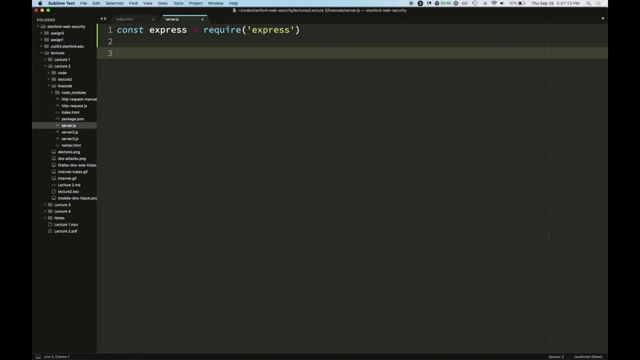 This is just a cert, a little sort of lightweight set of additions onto the Node HTTP package that like makes things like dealing with cookies slightly easier than having to make the headers ourselves and stuff like that. But it's really not. there's not too much magic going on here. 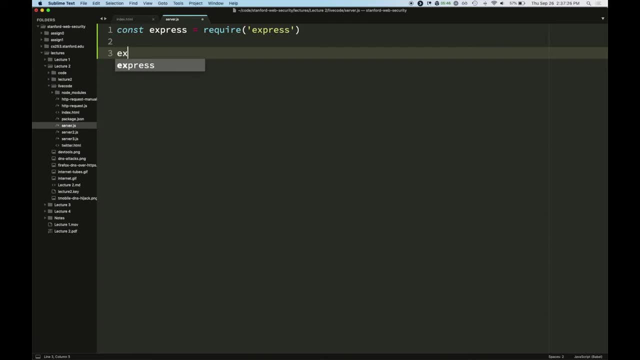 So the idea with with Express is we need to. we're basically gonna make a server And you do that by just instantiating an instance of Express And then you actually have to tell it what port to listen on. So we'll just say, like, start listening on port 4,000.. 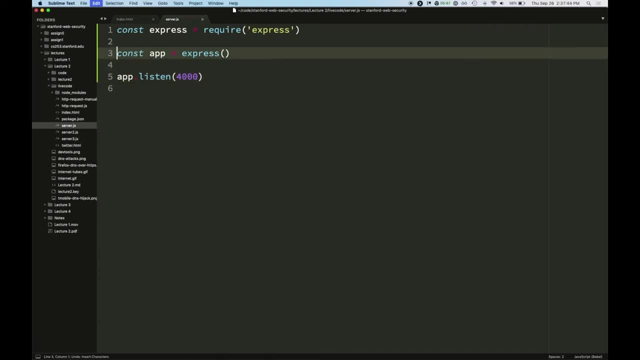 And now we have- we just made an HTTP server. Great, Let's, let's test it out and see if it works. So the way we do that is we need to make what's called a route. This is basically just a fancy like. 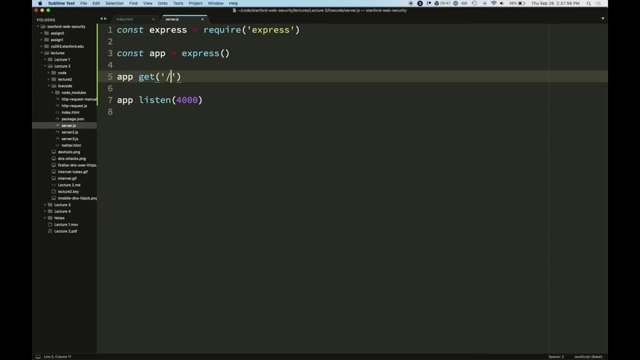 it's like a bunch of you have a bunch of switch cases And you're saying, if the URL that the user's visiting matches this right here, then I want this function to run okay, And so I can add a bunch of these. 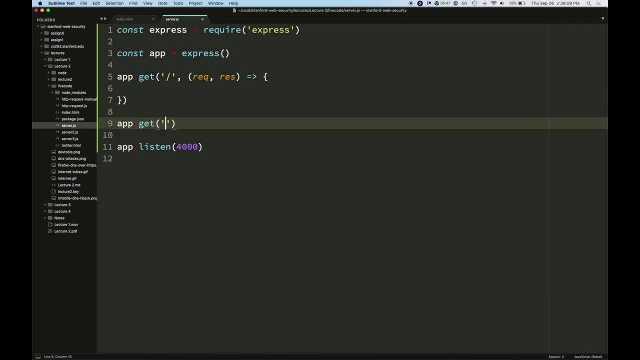 I could say: you know we're gonna later on, we know we're gonna need a login one right, Because we want the user to be able to go to login. But there's one thing I need to add here, which is: didn't we say we were gonna post to login, not get? 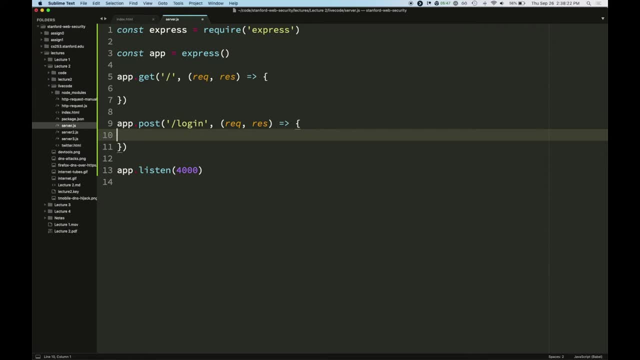 So we have to change this to post. So the server's gonna say, if if somebody po makes a post request And it matches slash login, then go ahead and run this function here to respond to them. Okay, Now we need to talk about what is a rec and a res. 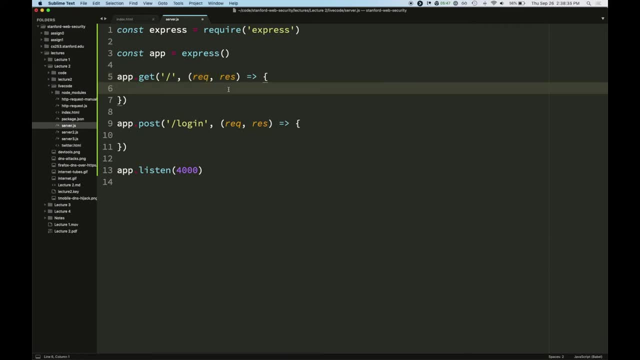 So rec is the request and res is our, is gonna be our response. So with rec we can learn things like what is the URL the user's on- Although that I guess that's kind of obvious because it matched this- But you can also look up like other things about the request. 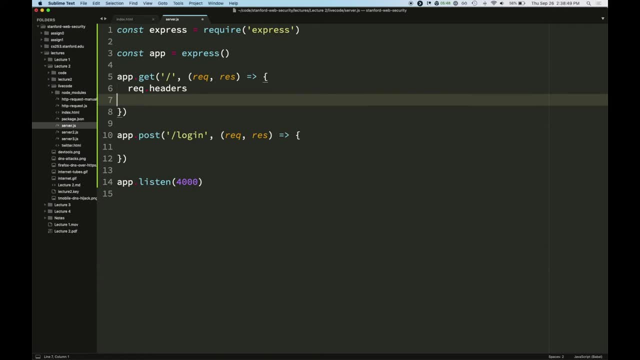 like the headers, for example, that's on there, stuff like that. Okay, so let's do. let's see what do we need to do. Let's see what do we need to do here. What I want to do is I want to load the home page. 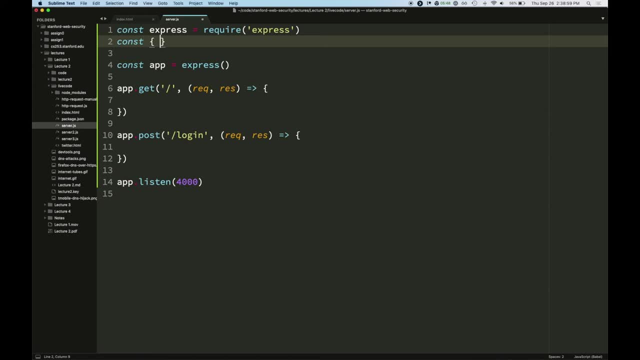 So let's, let's import this thing called fs- This is the file system module- and I'm going to import a function called create read stream. This is one of those streams like we had from before, And what what's cool about this is I can actually so. 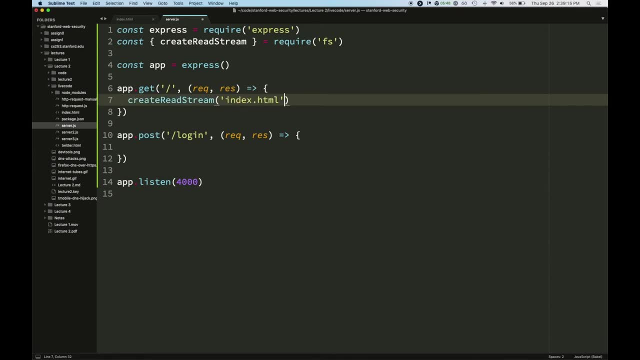 the. what this is gonna do is open up a file called open up the indexhtml file, And I'm going to send it out to the response. So the only the only reason why we're doing this is what I could do here is I. 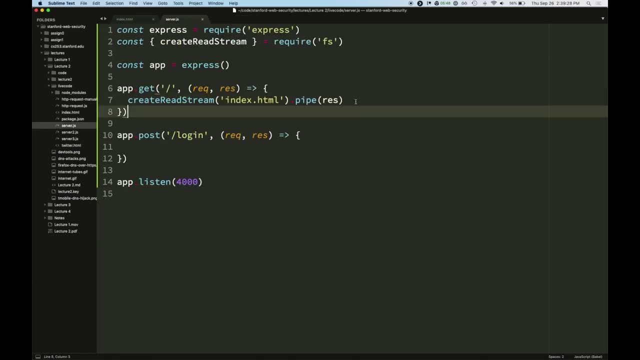 could. oops, what I could do here is I could just open up this file and read it in to like a string, and then I could write it out over the sockets, And that would work totally fine. Reason why I'm doing this is because this is just a slightly better way to do it. 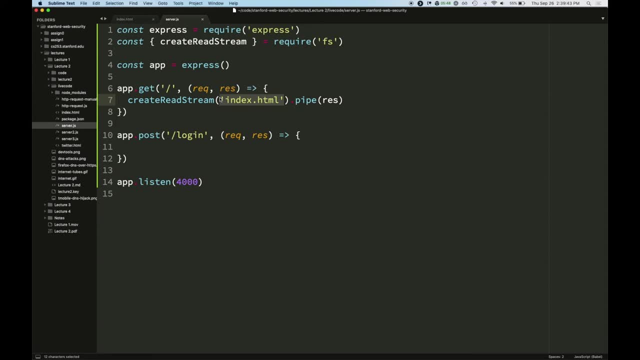 It means that what I'm doing instead is I'm as I read pieces of it out, I send them across the socket as soon as I get them, And so if this were, say, like a one gigabyte file, a ginormous file, right. 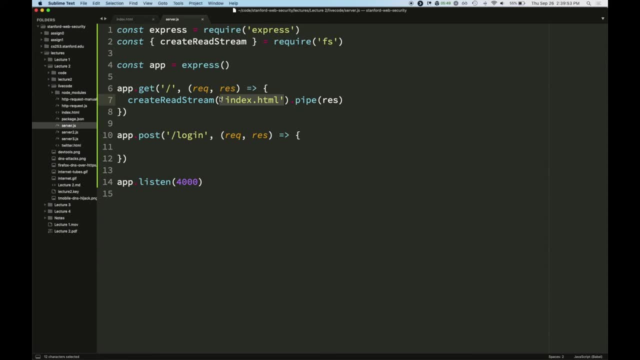 I wouldn't want to like tell the, the user, like, hey, please wait, I'm like reading this into memory, Using, using up, use up a gig of RAM, And then start to like proceed to send it to them once I've done that. 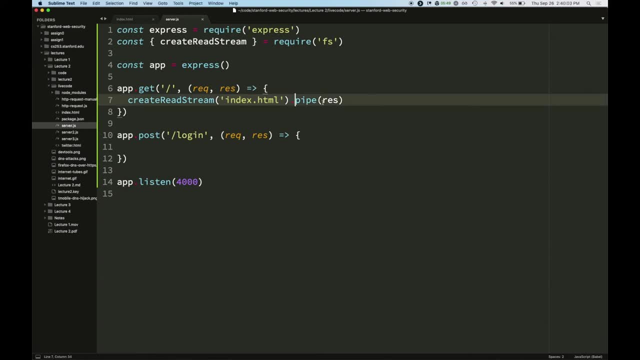 So it's just easier to sort of send it along as you go. And that's what this is doing: It's piping it to the. to the response object. I have a question. Yeah, What is the curly braces on your second line? 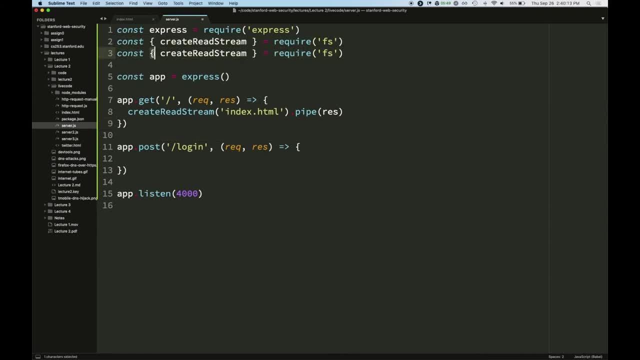 This one. Oh okay, so this is the equivalent of me writing this. It's equivalent of me writing that. So I'm saying, I'm basically saying, get requirefs and then pull this property Off of it and then make it available. 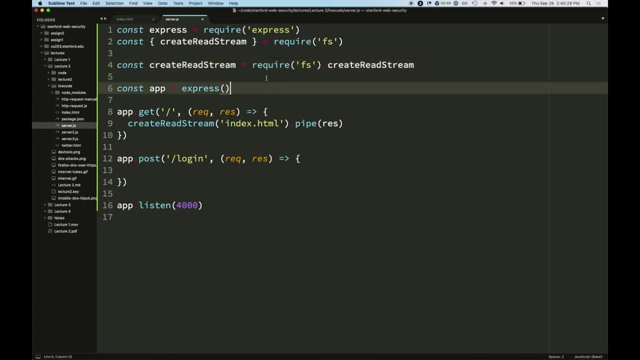 It's literally the same as this line. Does that make sense to everybody? It's just a fancy, a little bit fancy way of doing that, So I'll leave this here. I'll comment it out so you can see that. Okay, so now we, now we should, we should- have a home page. 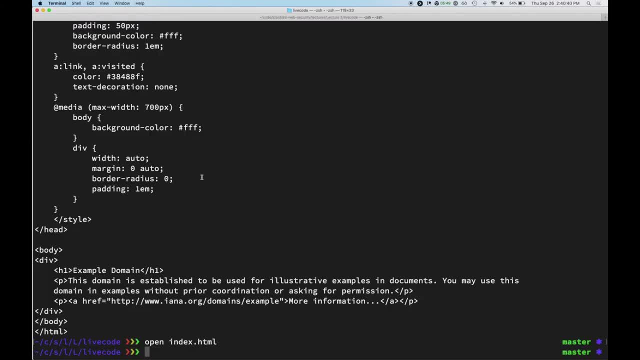 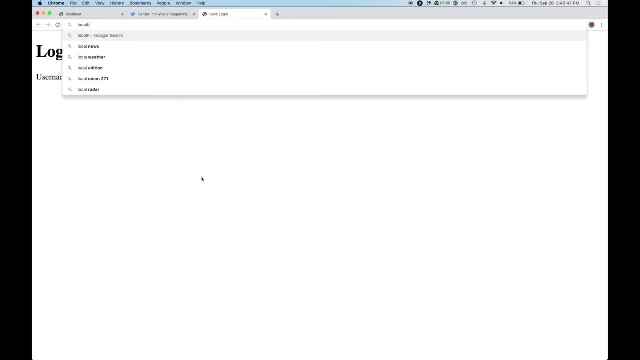 So let me save this and let's actually start up the server. So I'll do node server. I could do serverjs, Yeah. so now if I go to my browser on port 4000, I should actually have a real server serving me- the same page as before. 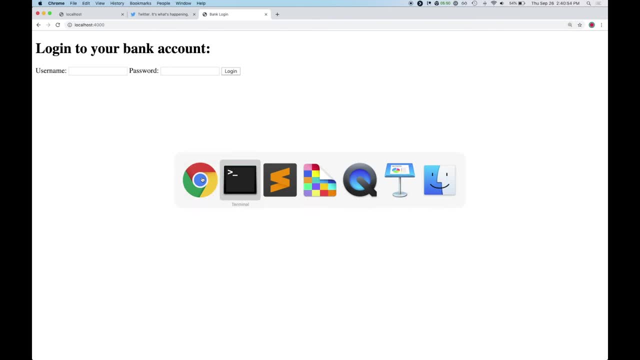 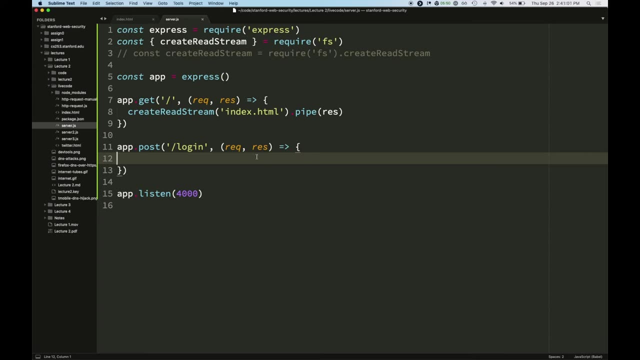 Okay, cool. Now what? what should we do? Well, we need to implement the login endpoint, right. Let's try to do that. So let's, first of all, let's. we're going to need to do one thing. 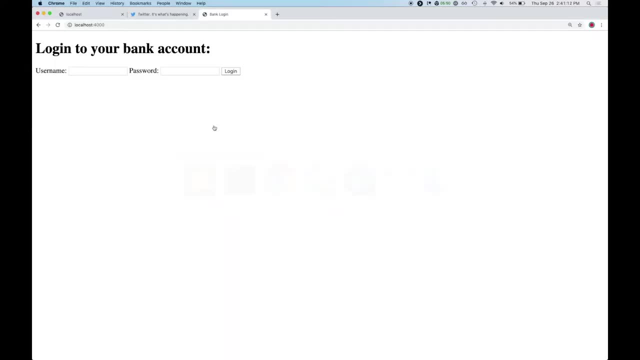 So so I want to make it slightly easier to read in this, this, this, whatever I submit here. So if I let's actually see what happens when I type in a username here, I'll type in Alice and password. So if I log in- ooh, I should have done that before I. 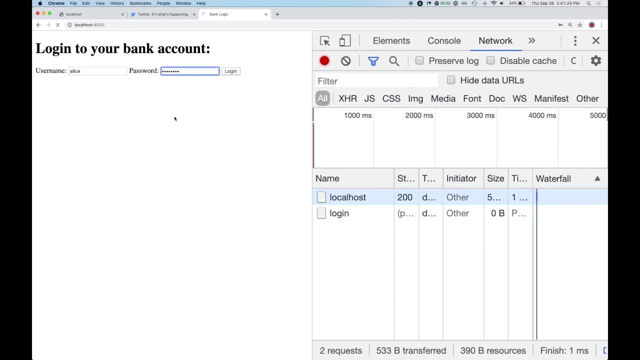 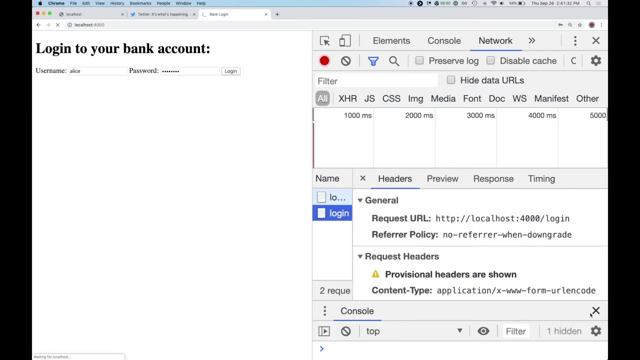 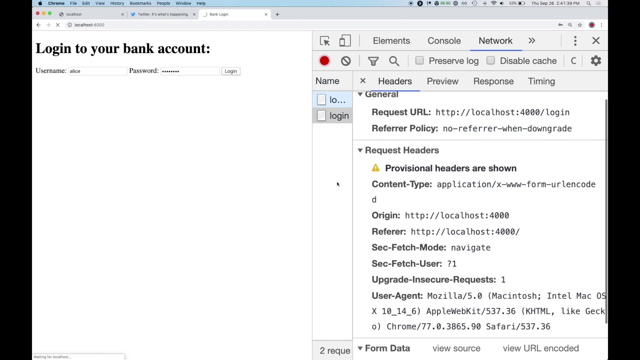 okay, let me refresh and I'll do it again. Alice password. So what happened here is I posted. this is hard to see. let me close some things here. Okay, so can everyone see what I did. So I posted to this URL and the form data is right here. 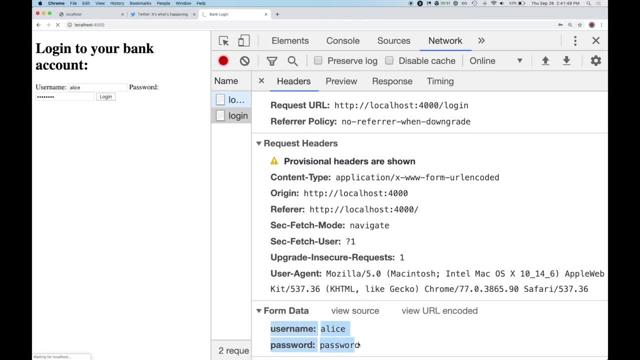 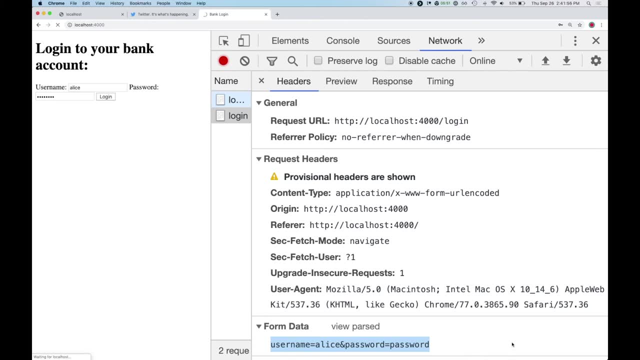 It's this username and Alice got posted Now. unfortunately it's not nicely formatted like this. It's more like this: That's what actually got sent to the server. Does everyone see that? That's a little bit annoying? I don't want to parse that myself. 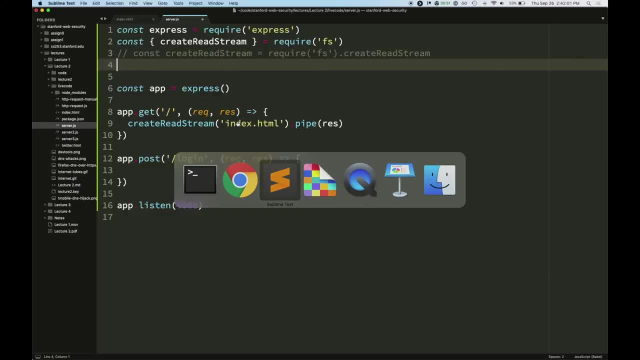 I could, we could, but but why So? so, to make it slightly easier, I'm going to import this thing called body parser. This is part of part of Express that is shipped as a separate module, And so all that I do now is up here. I'm going to tell Express to use the body parser. 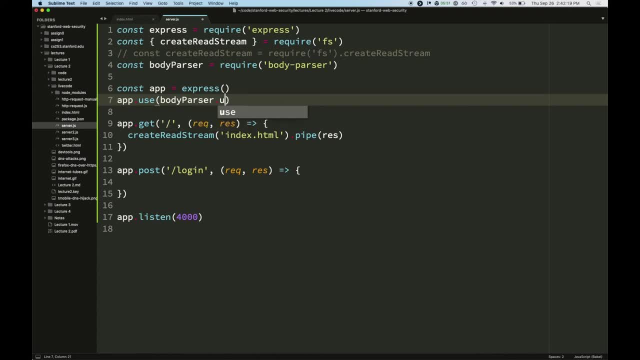 So let's- and there's just one thing I can do here. I can do this, I can do this. There's just one option I'm going to pass here, so it doesn't yell at me, It's not really important what that does. 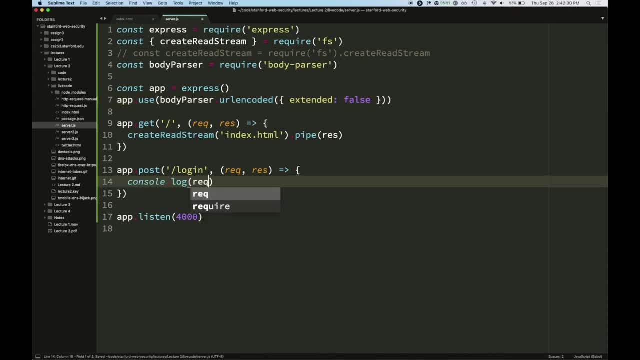 But now what I can do is in here I can actually, let's like, console log out request body. So now there's this magical body property that got added to the request. That's going to be a nice object with the, with the key and value, username and password. 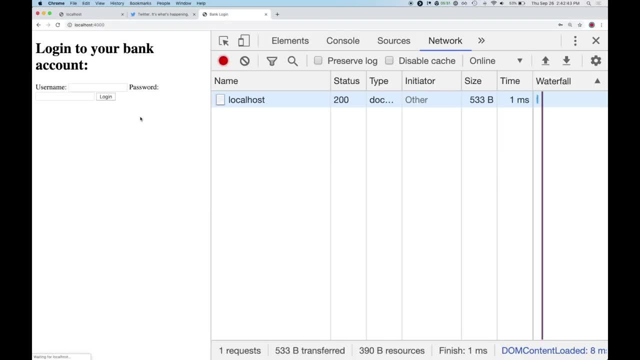 that the user posted to that URL. Okay, so now, if I go back to my browser and I actually I need to restart the server too. So one trick I'm going to do here is I'm going to use this thing called nodemon, which will 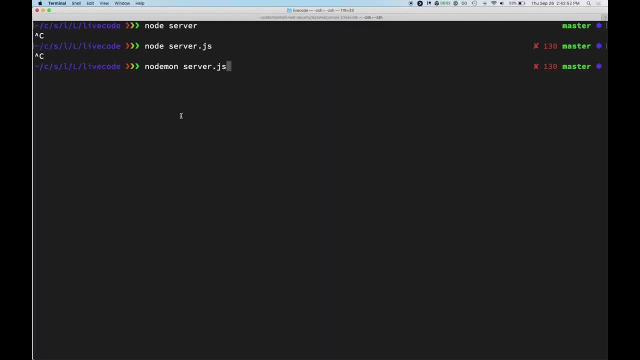 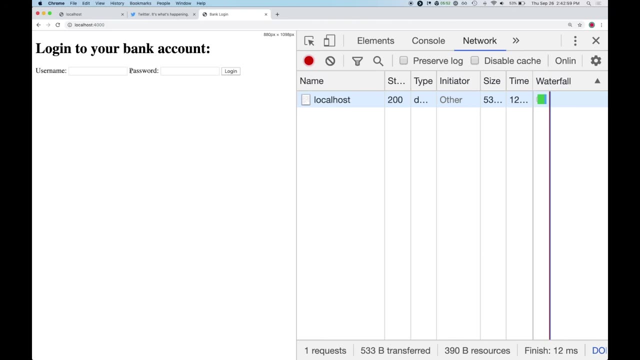 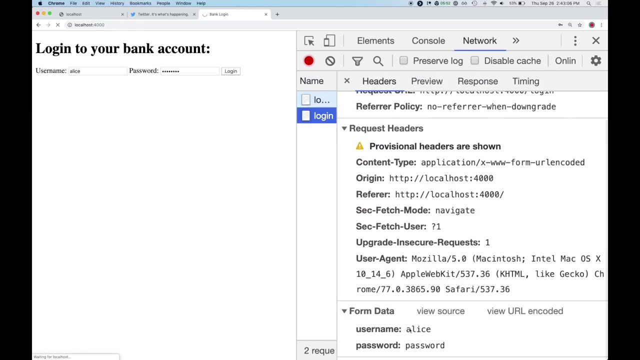 automatically restart the server any time Any files change in the folder that I'm currently in. So if we run that now, the server should have started up and now I can go ahead and try that again. So I'll type Alice, and I'm not going to tell you what I'm typing for my password. 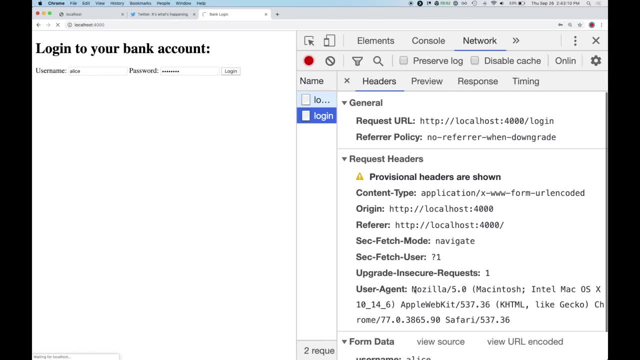 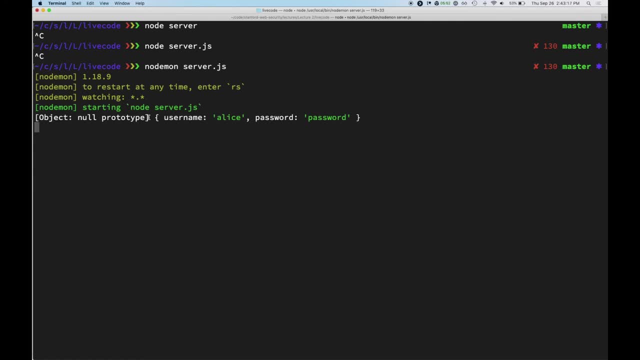 Okay, so that looks like it's submitted. Oh, okay, Dang, it Got to be careful, Okay so. so now we can see here what happened. is it printed out? I guess that was from before when I reloaded the page, or something. 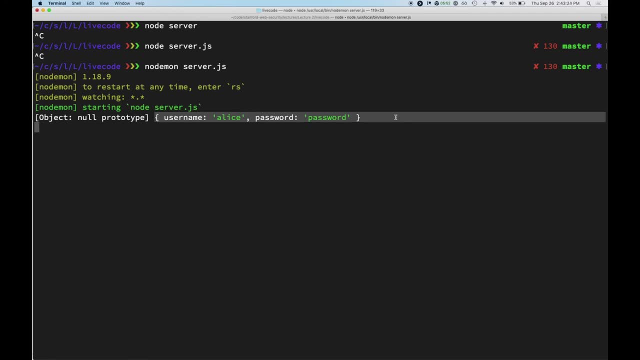 I don't know why, Why that got printed, But this is what was. this is what actually the request body is right. So now I have this nice object that can just get the username and password. So what should I do with this? 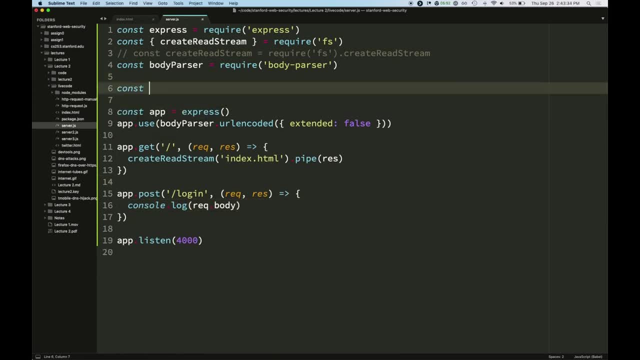 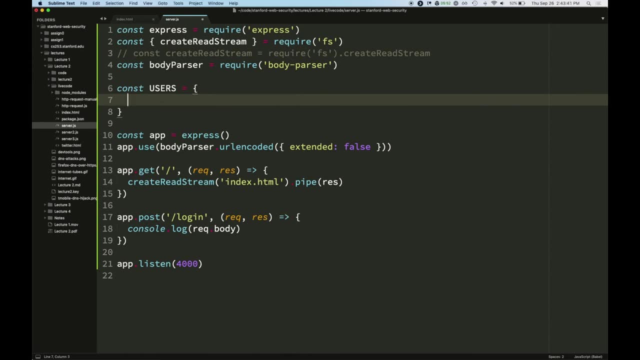 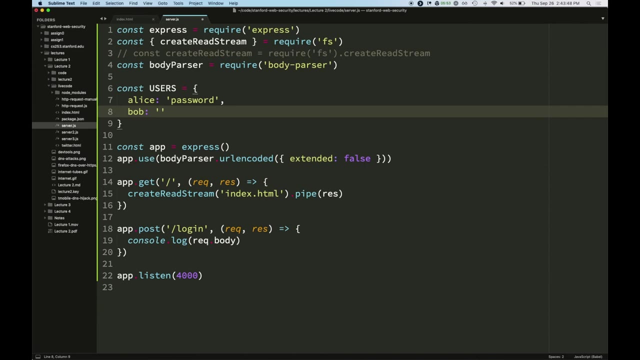 Well, one thing we can do is we can, let's make a user database. So this is really fancy technology. It's called objectdb. So here's my, my database of users. Okay, what should? what should Bob's password be? 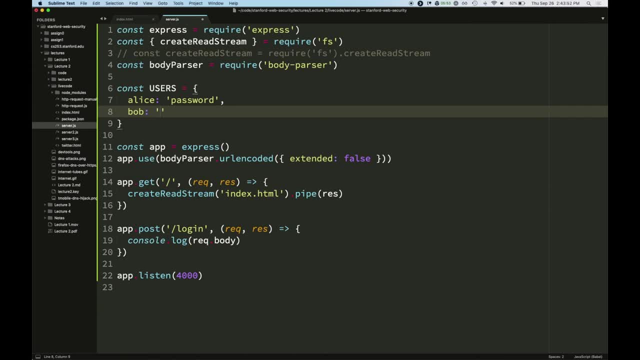 What's your favorite weak password? Don't leave it: Hunter 2. Hunter 2. Hunter 2.. Okay, Yes, Yeah, that's a good one too. Okay, so now we have two users. Now what I'm going to do is, when the user goes to log in, I'm going to get the username. 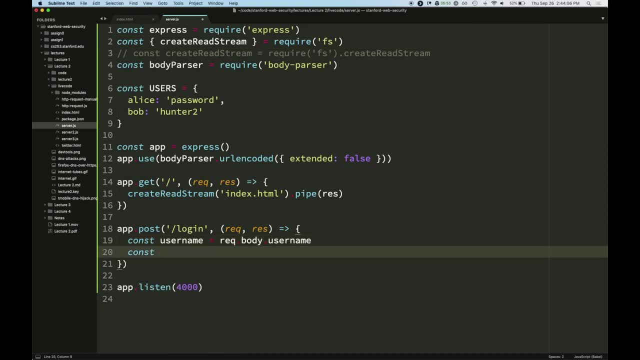 off of the body and I'm going to say, okay, so that's, that's the user you're trying to log in, as Okay, What's their actual password? Well, I looked that up in the user's object and now I know, okay, the user they're trying. 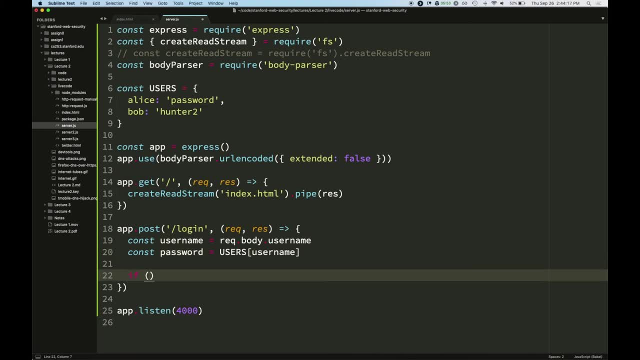 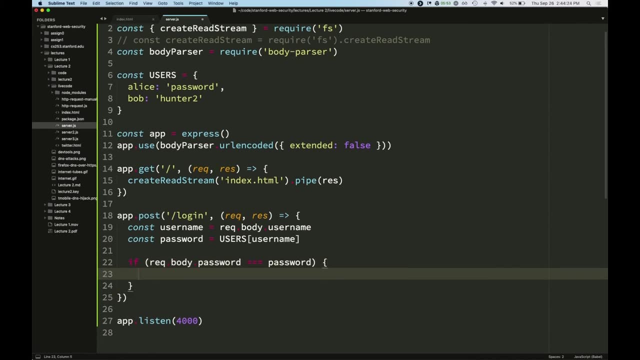 to log in and what the real password is, and then I'm going to say if the request body's password matches, If it is a password that it's supposed to match, then I'm going to, on the response: add a header. 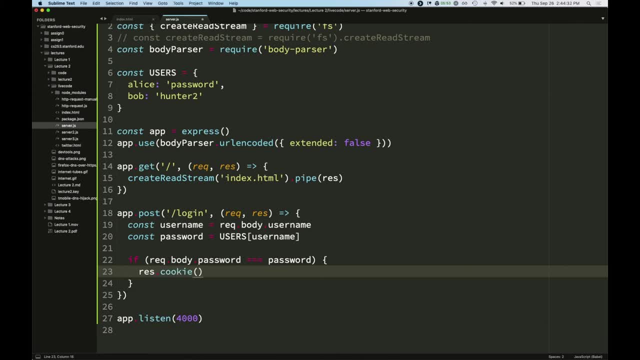 Actually, how about? instead of doing that, I use the cookie function. it'll do it for us. It'll add the set cookie header. Now all I have to do is give it a cookie name and a cookie value. So what should we set here as the the cookie name and value? 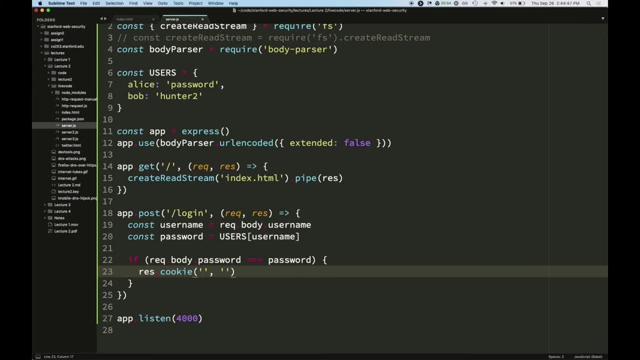 Let's do something really, really naive at first: Sign Sign. Well, if we did signed in, then we wouldn't know who was signed in- right Username and the user. How about? What was that? Yeah, yeah. 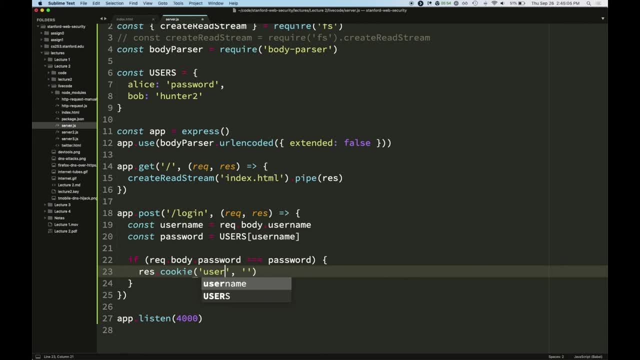 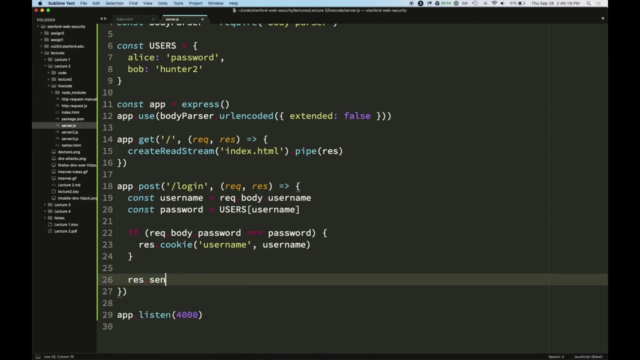 So let's, let's just call it username, for simplicity, and then that'll be, and then we'll make it be the user's username that they're logged in as. How about that? Okay, So, so now, Um, So let's respond with something. 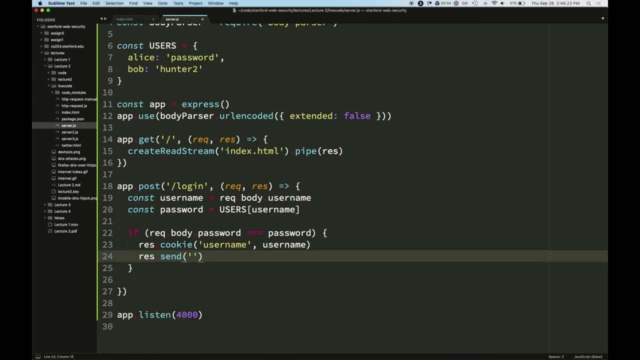 Let's tell them: you know um. if they logged in successfully, let's tell them: you know nice. Otherwise, let's tell them: uh, fail, Okay, Uh cool, Let's let's see if that works. 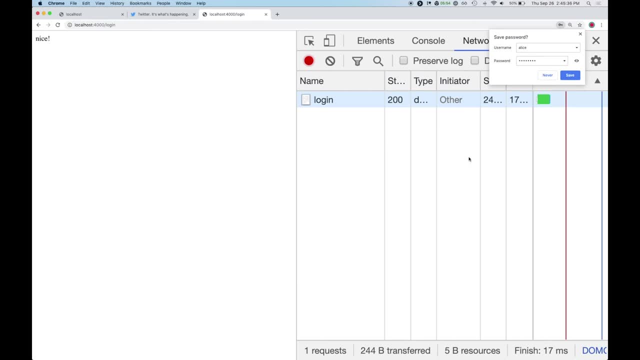 So, uh, the server automatically restarted. I'll just refresh. Oh wait, What? How am I Nice? Oh, I remember I refreshed. I resent the same um the same password I typed in before, Okay. 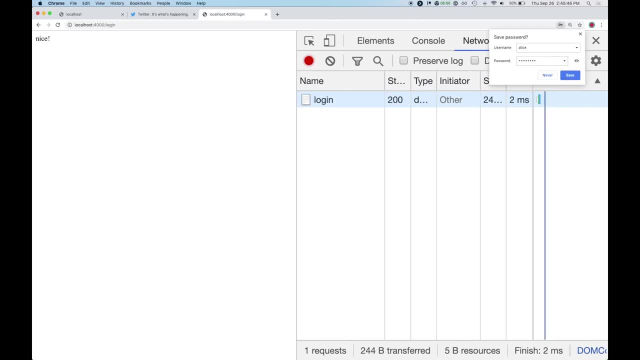 Let's, let's do that again. So I'll go to the homepage, Type in Alice password. Nice, Okay, So I do it again. but I I do it wrong, Fail. Okay, So it works, It works. 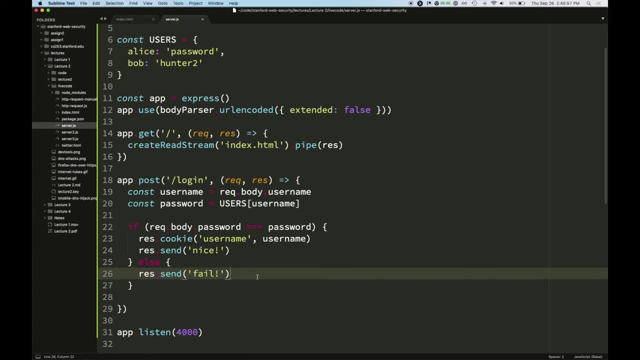 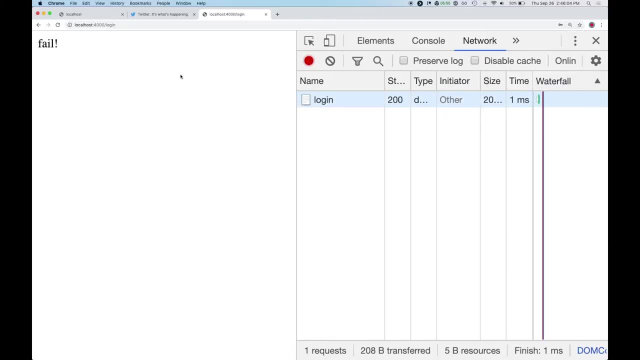 Okay, So now, um, now the, the, the, um, so we're detecting this correctly. but did we? did we see if the cookie was set correctly? We didn't, So let's see what happened there. Um, right, 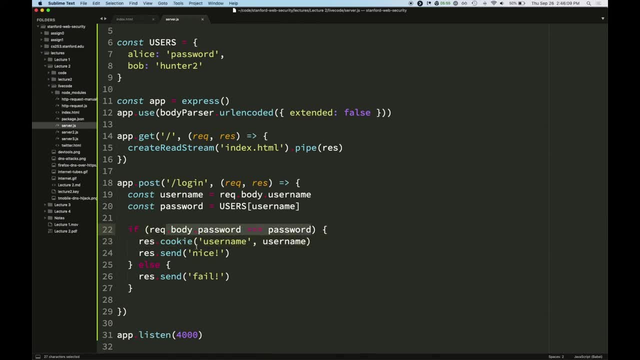 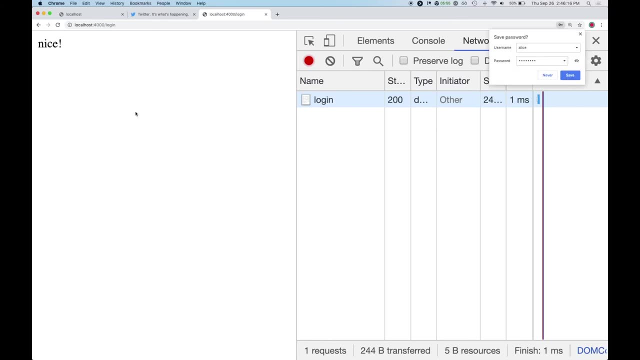 So because, remember, we said if we, if we get the password correct, we're trying to send this cookie down to them, Right? Um, so let's see if that worked. Type Alice password Log in. Okay, So now if I look at the request, 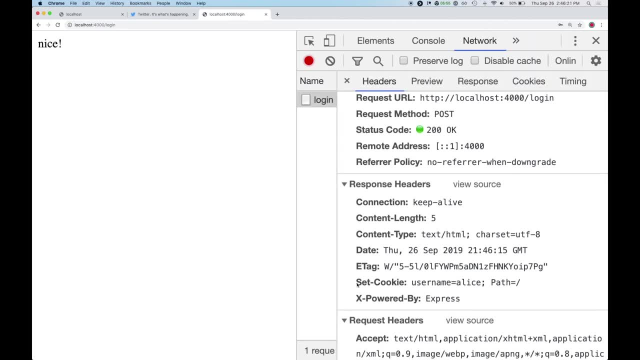 I should see in the response set cookie username Alice. Uh, don't worry about path, We'll talk about that that later. But, um, but this is the server telling me. remember that you are Alice, uh, and tell. 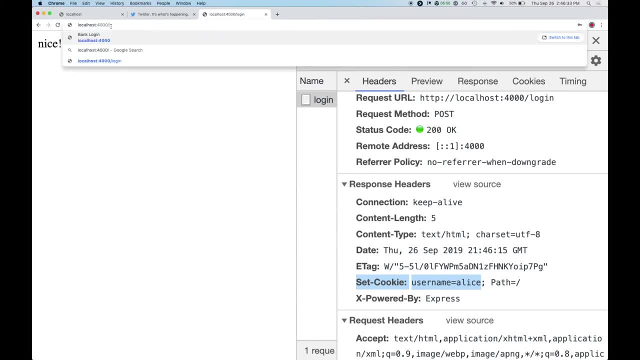 me that every time you talk to me again. So now, if I go to the homepage and I re and I load that up, we should see in this request: even though I'm, it doesn't look like I'm logged in because the server's not doing anything. 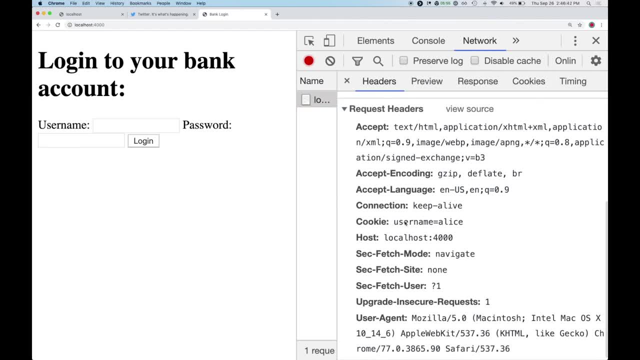 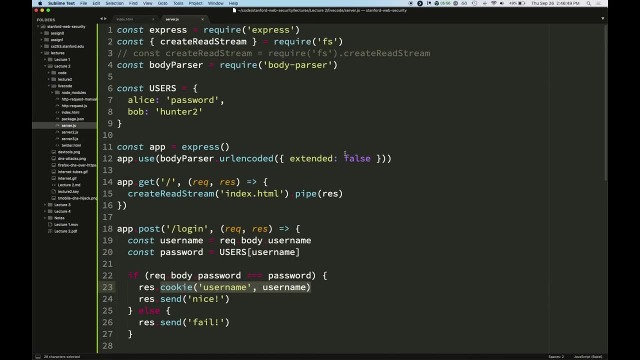 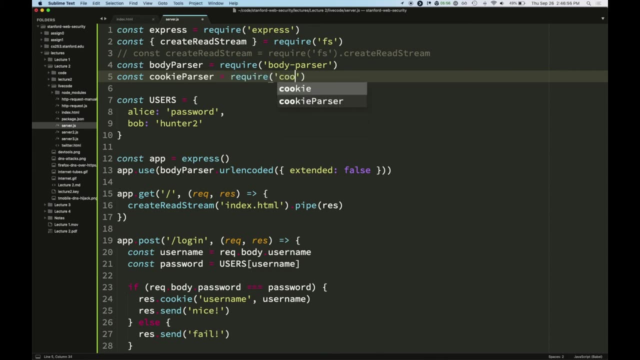 with it. The request should contain cookie username Alice, which it does. Great, So let's use that to log in Alice when it's present, Right? So how can we do that? Well, we need to um, import a thing called cookie parser really quickly, because I don't. 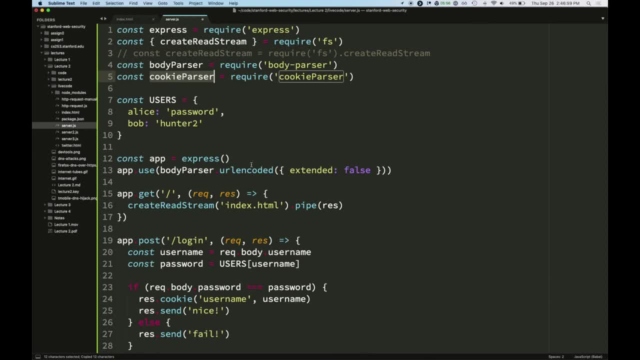 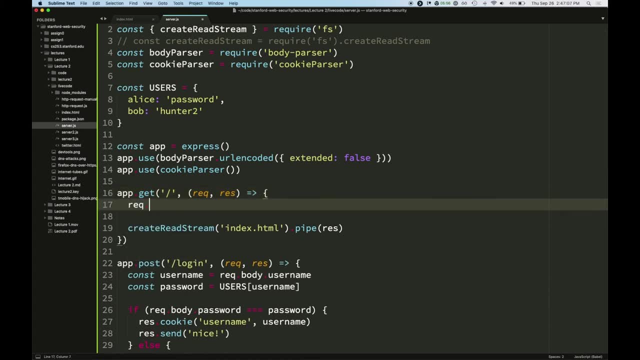 want to parse the cookie, Um, and I just use, I just type app dot, use cookie parser to to to have it do that for me. And now, just because I did that, I now magically have a thing called rec dot cookie which gives. 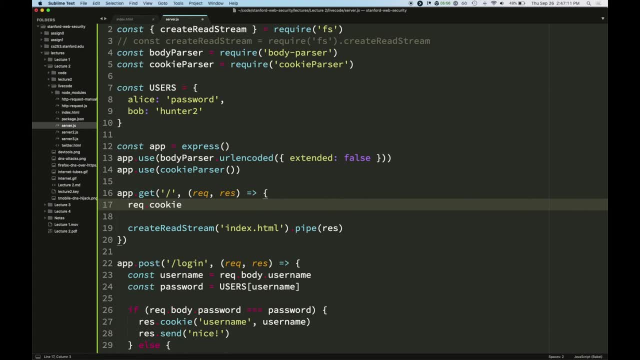 me an object with all of the cookies, um, that are on the request that I just got, And so what we're doing in here is this is for the homepage. So when the user loads the homepage, I'm going to say who are they presenting themselves? 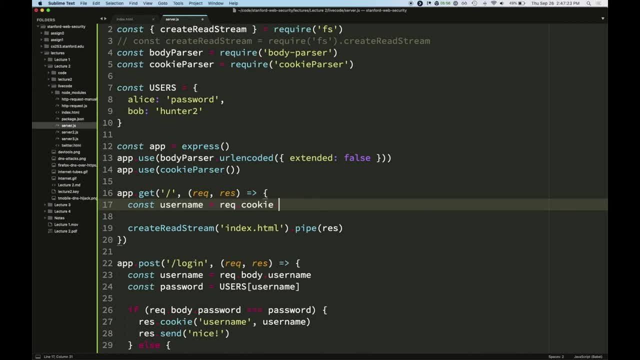 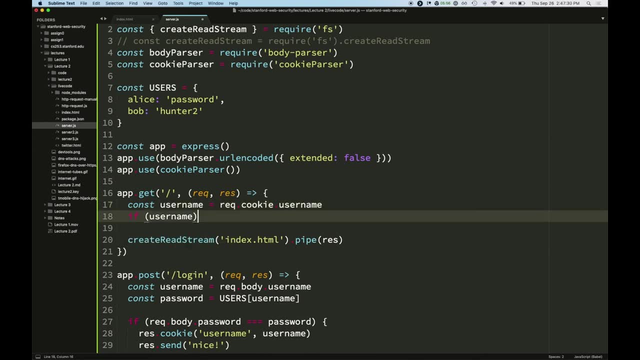 as. So I'll pull the username off of the cookie right And I'll say: if there is a username, cause this could be undefined. if there is a username, then I'm going to greet the user and tell them you know something like: uh, what should? 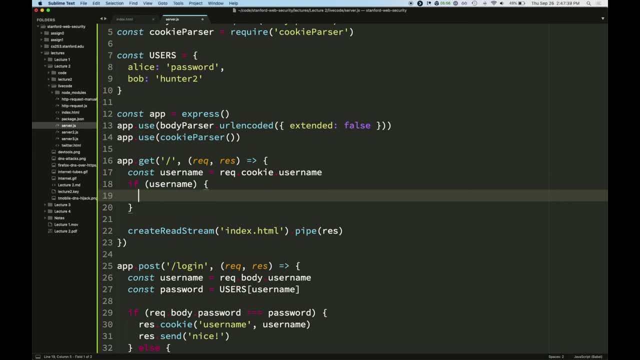 I say I should say uh, hi and then their name. How about that? So we'll send hi, Hi, Uh. this is just a way to include um, a variable in your string. So I'm going to say hi, username. 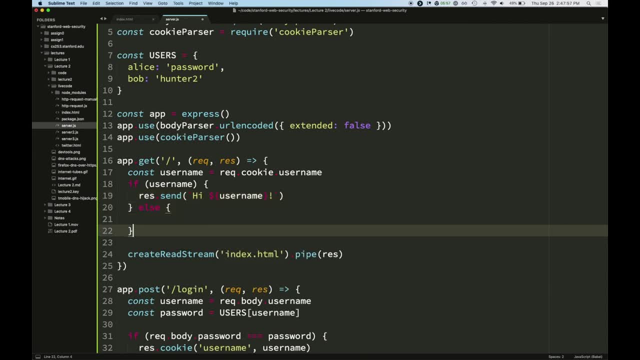 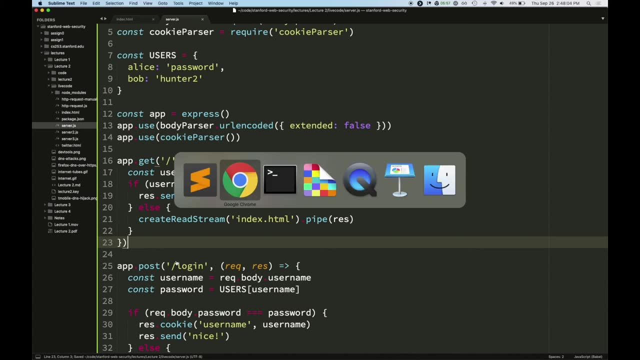 Okay, And otherwise, if there's no username, I'll just give them the the login form like before. Right, Make sense, Everybody, Okay. So now if I refresh the page, um, my browser should remember that I'm logged in as Alice. 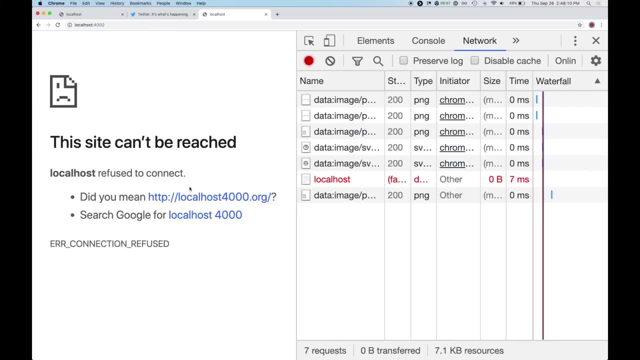 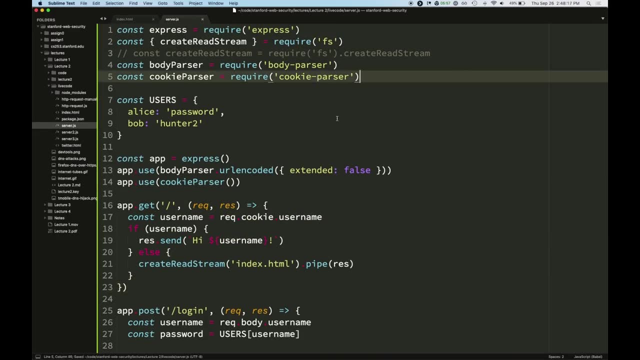 cause that cookie is set. So if I refresh, I should just now magically be logged in as Alice Great Uh, cookie parser. Let's see. Oh, I imported it incorrectly. It's supposed to be like that. Okay, That was easy.